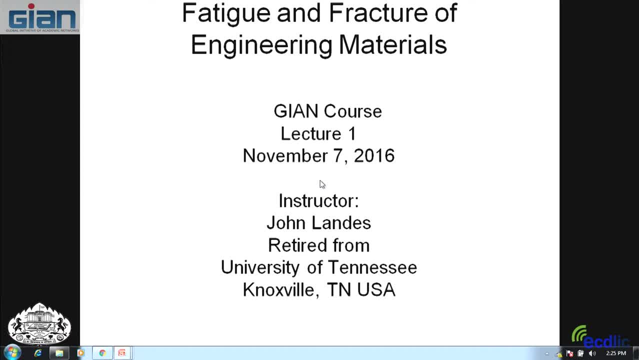 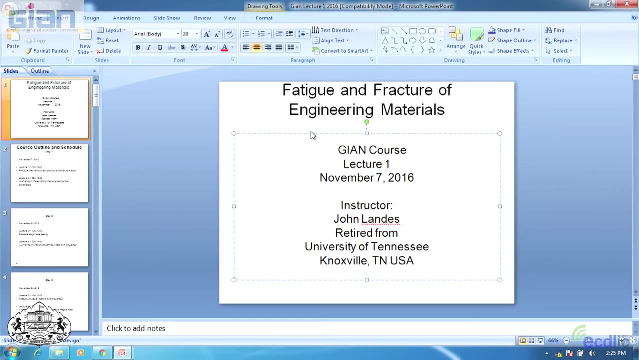 I thought I would show you something. I've got it stuck There. it's unstuck, Thank you. This is not my laptop, so I'm not quite used to it. I wanted to show you something. Here is a map of Tennessee. For those of you who aren't. 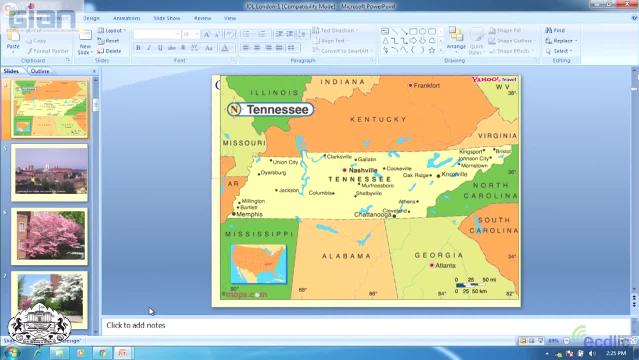 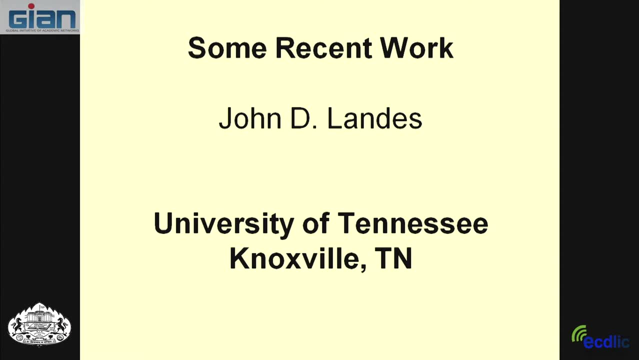 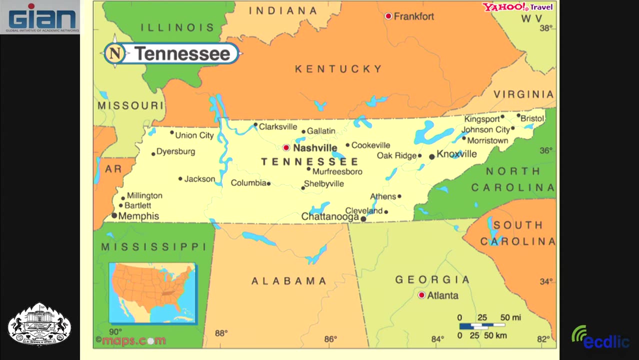 familiar with the United States. this is in the Southeast. We are in Knoxville, This area right here. we are in Knoxville. in that area the weather is a little bit colder than here. There's a lot of wind. The wind is getting a little bit cooler and cooler than here. 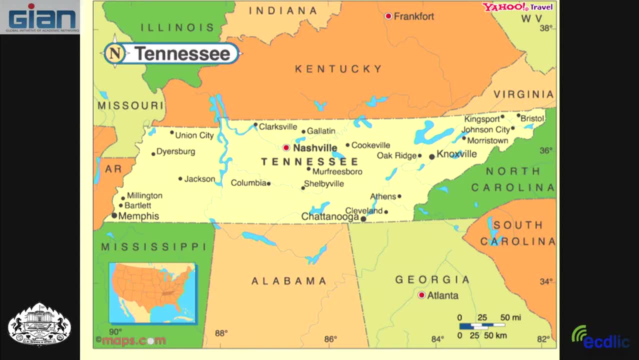 a lot of diverse people there. you see Oak Ridge here at Oak Ridge is a national lab with a lot of research. Knoxville has the University of Tennessee and so a lot of highly educated people and in the area is Smoky Mountains and a lot of mountain areas here and the other side of the 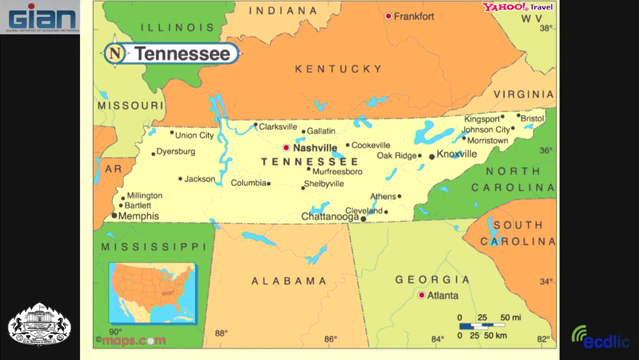 thing is the mountain people. mountain people are sometimes called rednecks. if you're a mountain person, you need to have long hair and a long beard. you can tell if you're a real redneck if you are sitting on your rocking chair and a bird comes along and builds a nest in your beard. you're. 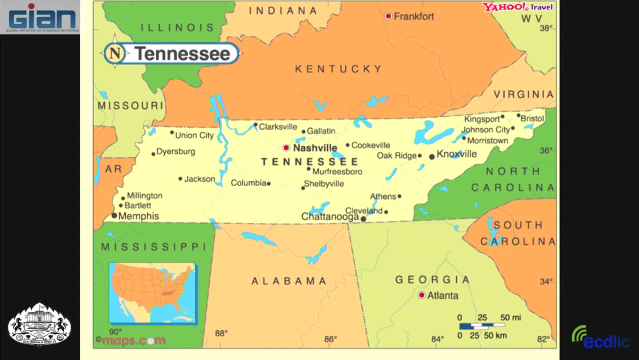 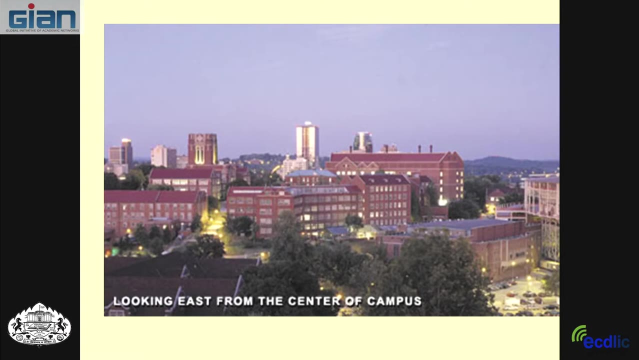 known as a real redneck, and you're also known that it's probably time to get off the rocking chair after that happens. we we get along with both. they speak a different language, but we've gotten used to it. show you a little bit here. this is what the city of Knoxville 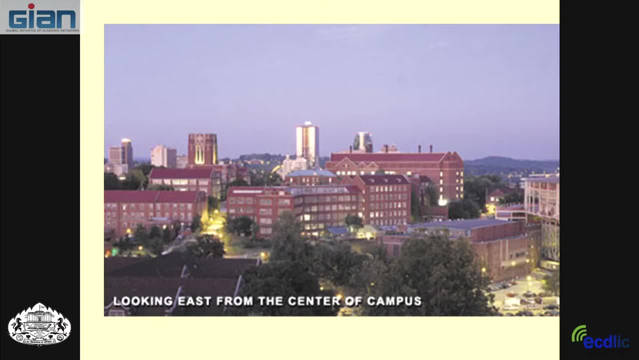 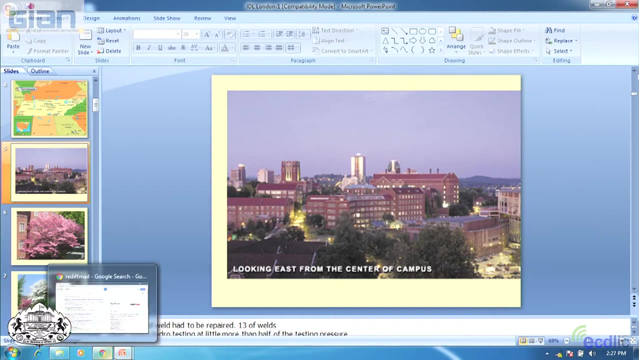 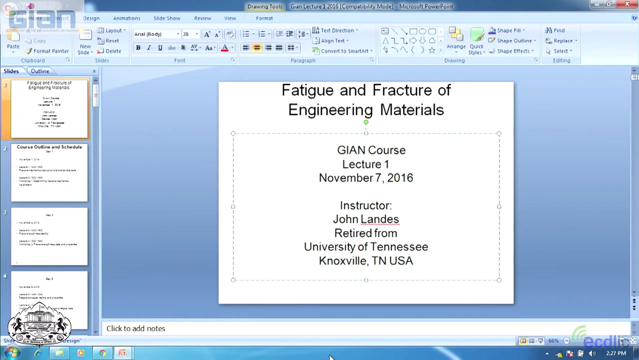 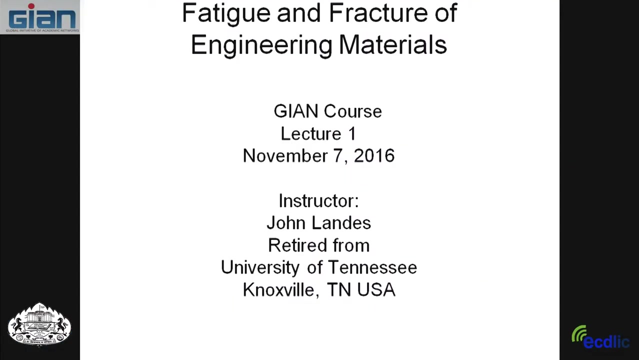 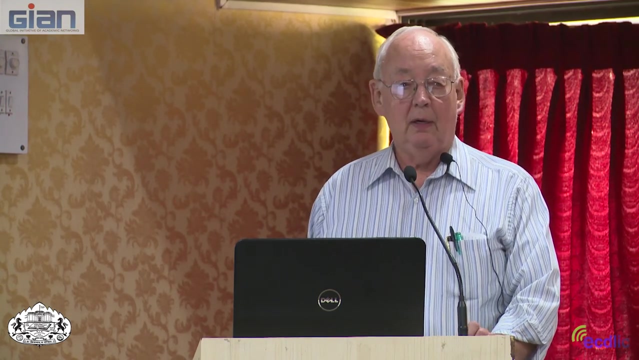 looks like there's about 200,000 people in in the city itself and more around the the area, so that that is a little bit of where we come from now, if we can get back to the main course. I want to say a few things before I start on the lecture. there's not a real big group, so I want to 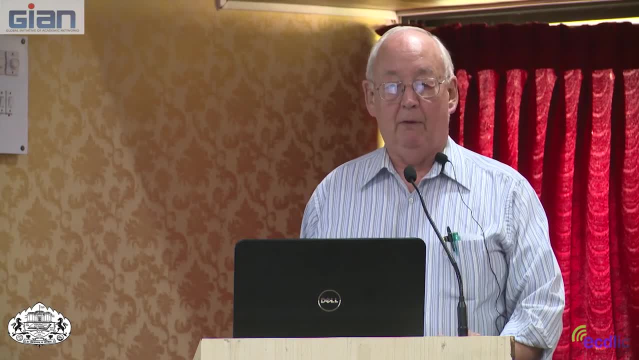 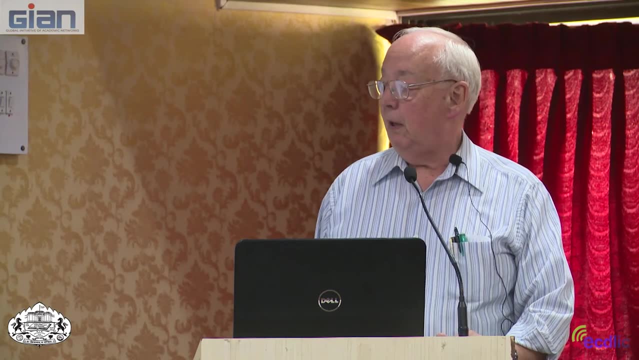 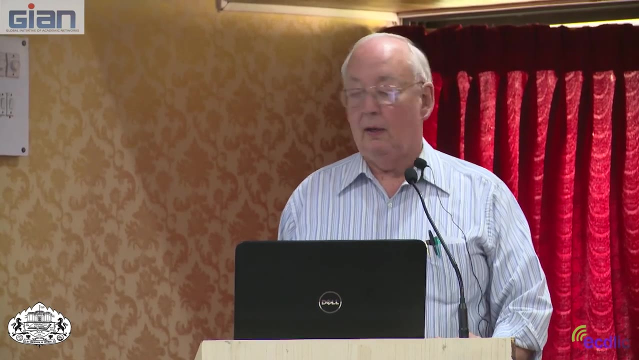 keep this as a teaching session rather than a formal lecture. so anytime anybody has a question during the conduct of my lecture, stop, then we'll try to answer that question. if I don't know the answer, I'll either make it up or say I don't know. the other thing is that we have a lot of 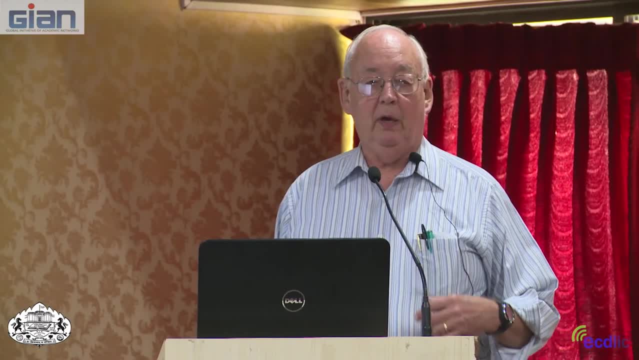 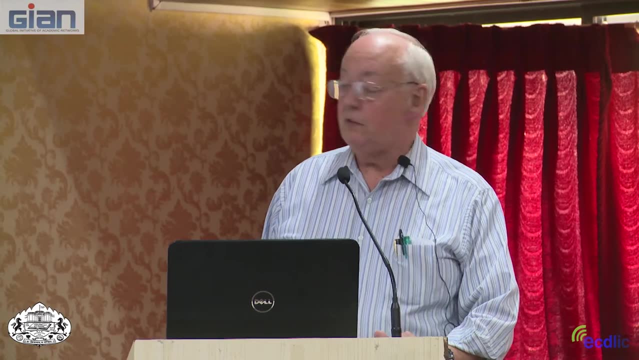 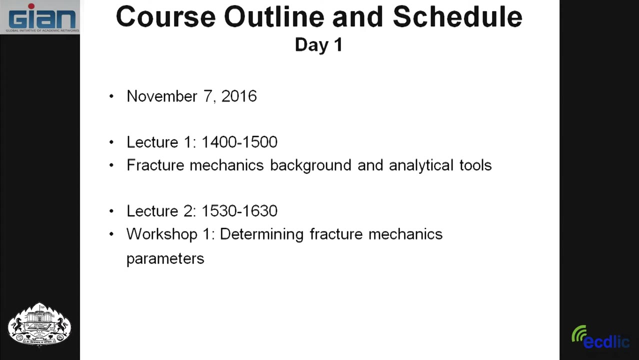 people who like to be weasta trouble. I apologize everybody for letting us off, but I do have to note. one very convenient thing is: it's right after lunch and it's warm here. if you get really tired, put your head down and take a nap, but try not to snore. this is a little bit of. 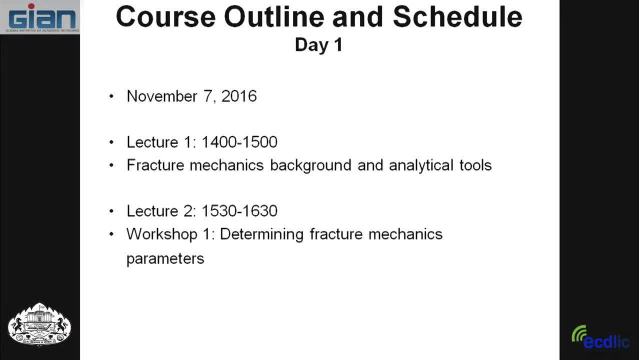 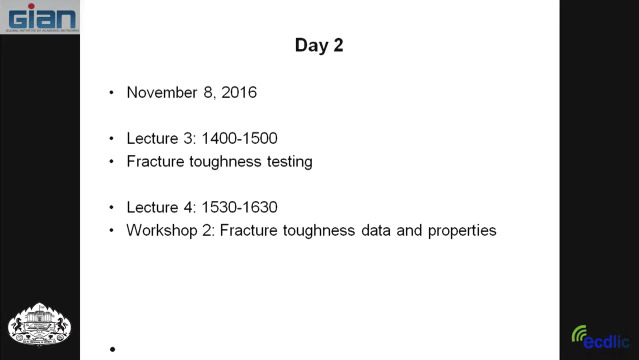 the outline. normally we're supposed to go two to three. take that two letter break, the PNT break or vice versa and then. So this will be how it goes. I'm not sure that I'll keep right on the schedule I have here. If not, it's quite okay. 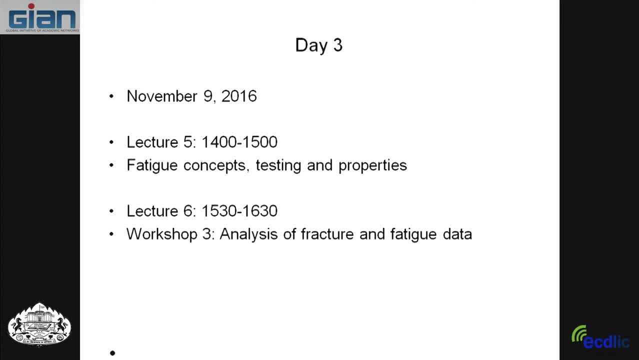 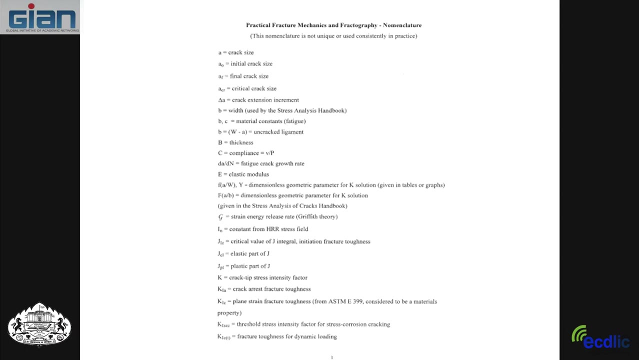 The first week I have more important stuff than the second week, So if you want to nap, try napping next week more than this week. These are all the days. I didn't want you to memorize it, And one of the things we have in Fracture Mechanics is nomenclature. 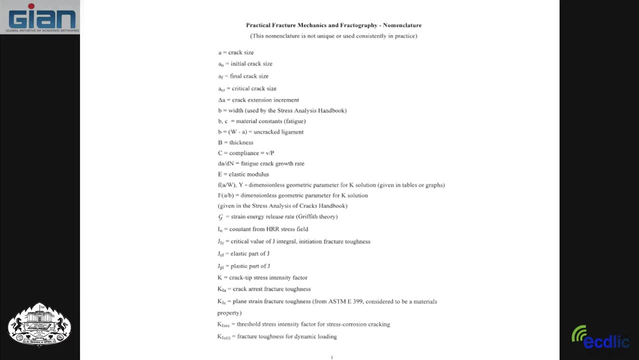 Eventually, I want to get a handout for everybody so that you'll have this. The nomenclature again is not something to go through, but something I always give to students when I do this course so that they can go back. We have a lot of nomenclature. 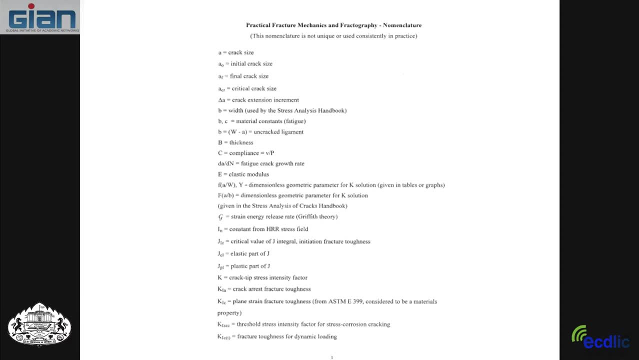 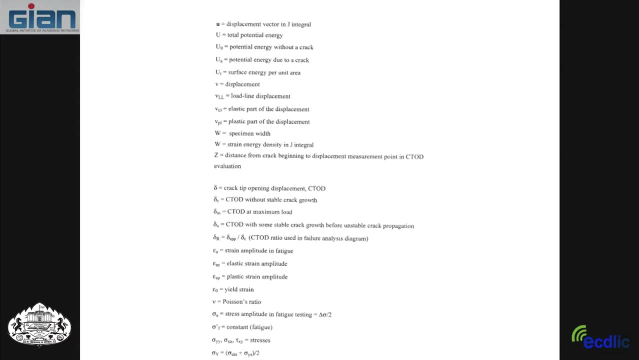 It's not unique. Sometimes the same term has different symbols, Sometimes the same That symbol has different terms. but there's a lot of nomenclature, The Roman alphabet, the Greek alphabet, and here are the case solutions that we'll get to. 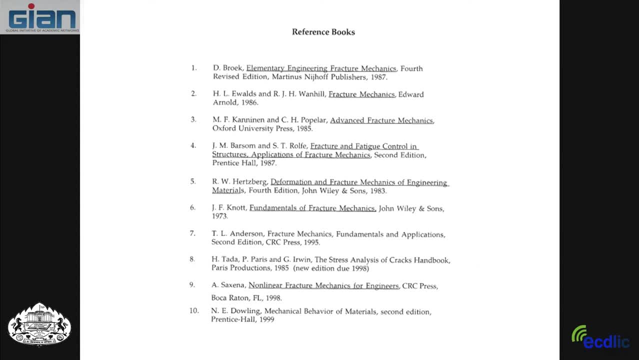 Also, I have in here some reference books. If you work in Fracture Mechanics, you might be interested in what kind of textbooks to have. I was going to bring along some examples, and when I picked them up they weighed more than my clothing. 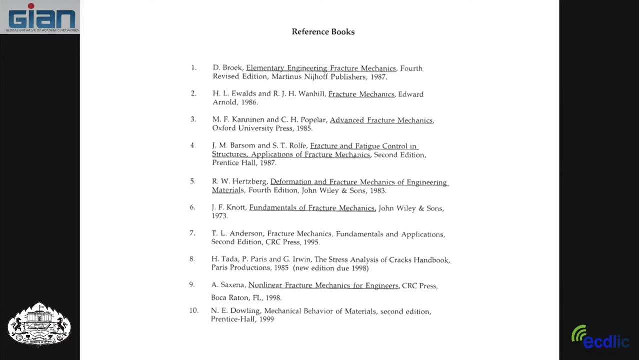 so I didn't bring them, because I thought I'd rather be dressed than have the books, And so I'll show you some of the ones. When I teach a Fracture Mechanics course at the university, I use this as a textbook. 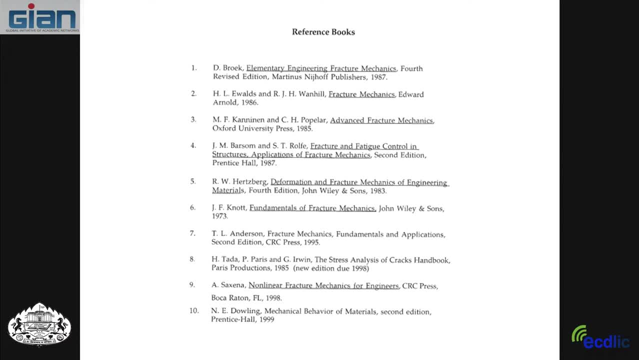 Ted Anderson. It has the most comprehensive linear, elastic, nonlinear things And this is a case solution book that we'll talk a lot about. Here's one: A colleague of mine was Saxena, who is Indian, and we worked together for a number of years. 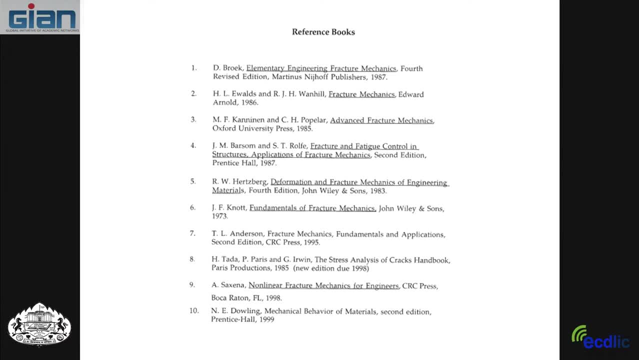 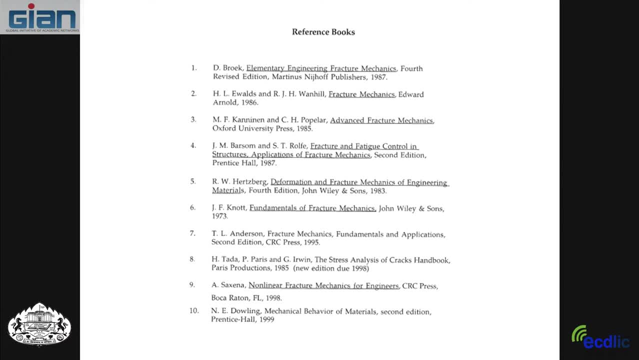 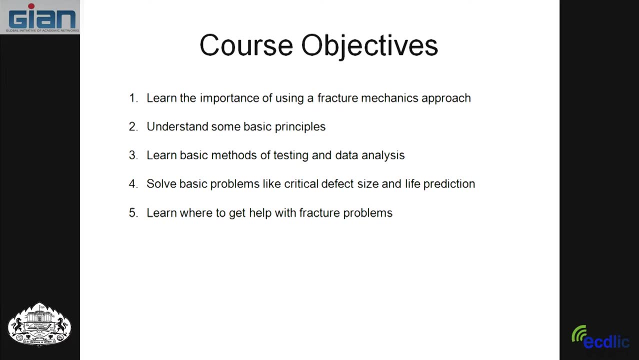 He was also a colleague of mine. Both of these worked with me at Westinghouse. Some journals: Course objectives: You should learn the importance of using a Fracture Mechanics approach, Understand some of the basic principles, Learn to do how you do testing and analysis, and solve some basic life problems. 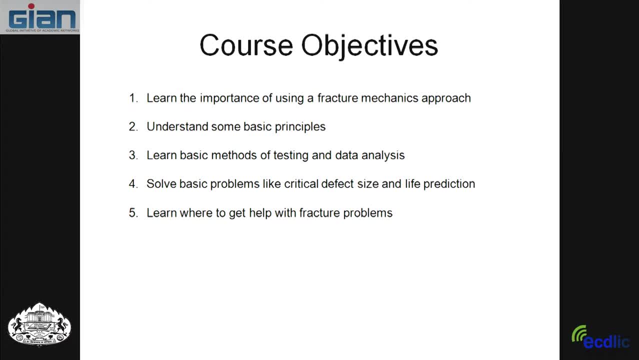 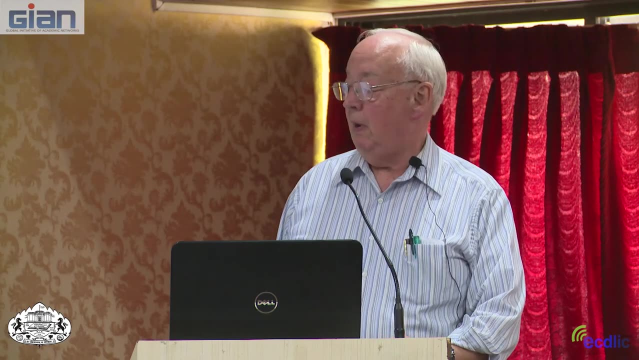 If you can't remember all this stuff, you should learn how you can get help from people. I do a lot of paper reviewing and a lot of the papers I review are written here in India, So you have quite an active group of people working in Fractured and Fatigue here in India. 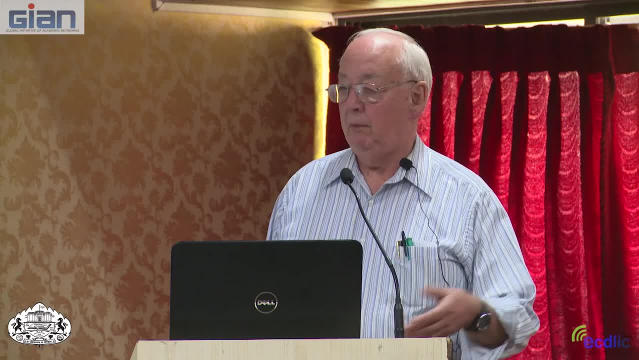 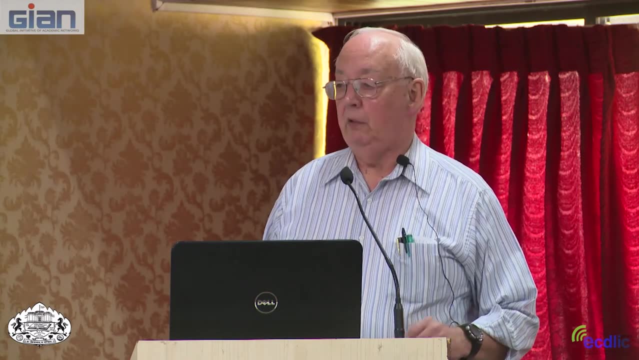 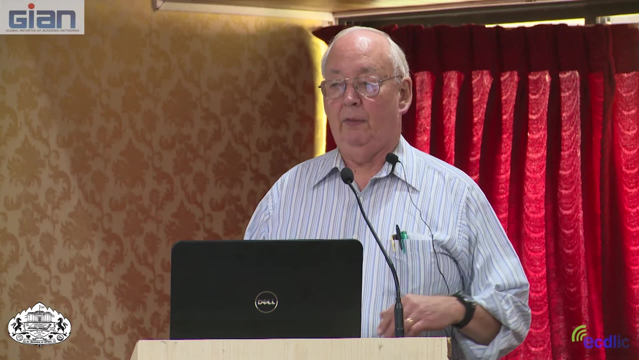 So often see that, And you're only beaten, maybe by the day, And you're only beaten by the Chinese. So a little bit of introduction. This first whole lecture is kind of what I call arm-waving stuff. I didn't mention it, but my background is more in the mechanics side than in the materials side. 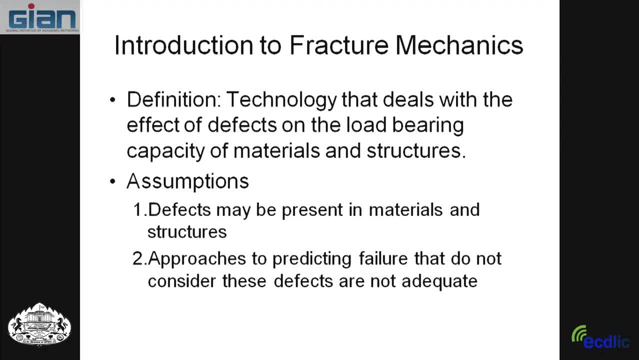 So I tend to be mechanics-oriented, And this is not real mechanics stuff, but just arm-waving definitions of things. The definition that we often give for Fractured Mechanics is a technology that deals with effectiveness. It's a technology that deals with the effects of defects on load-bearing capacities of materials. 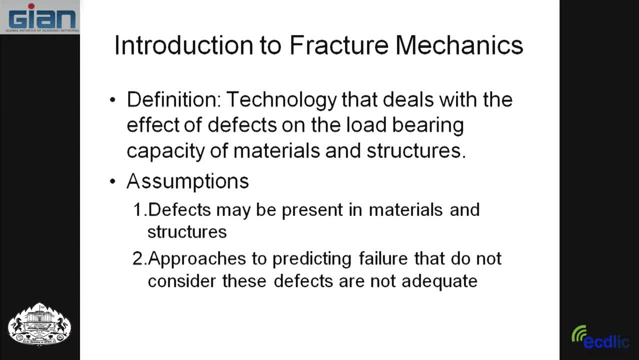 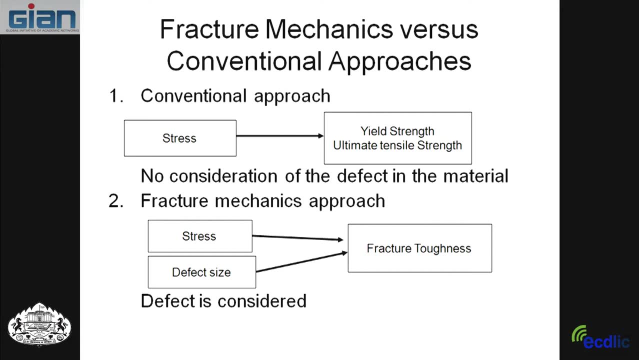 and structures And we assume that there may be defects in the materials. And if you have defects in the material, the approach you use to predicting failure- that doesn't consider the defect, might not be adequate. Here's a little schematic that I use. 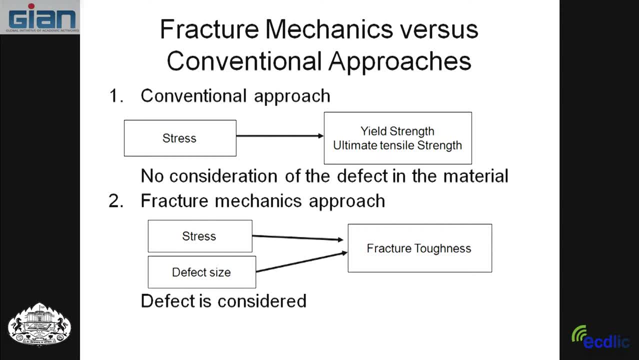 What we teach the undergraduates is the conventional approach. For those of you in engineering you of course know you have strength in materials, Strength in materials courses. In strength in materials you learn how to calculate stresses in all kinds of bodies And then, once you calculate those stresses, you can look at failure depending on a stress. 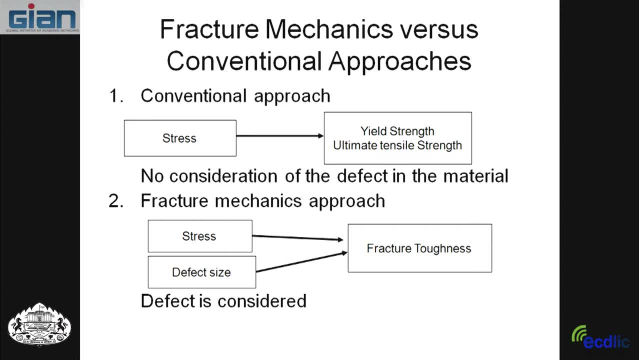 value like yield strength or ultimate tensile strength or maybe strain, But that doesn't consider what happens when there's a defect in the material. When there's a defect in the material, then you should use the Fractured Mechanics approach. 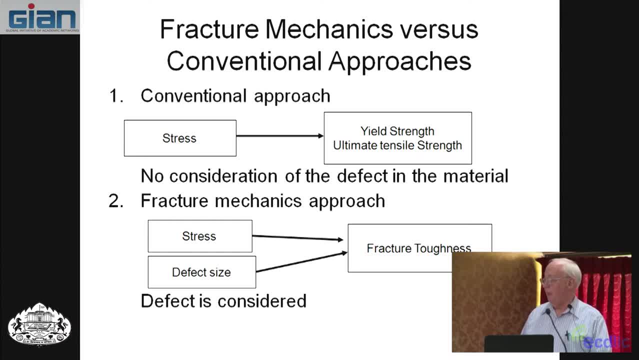 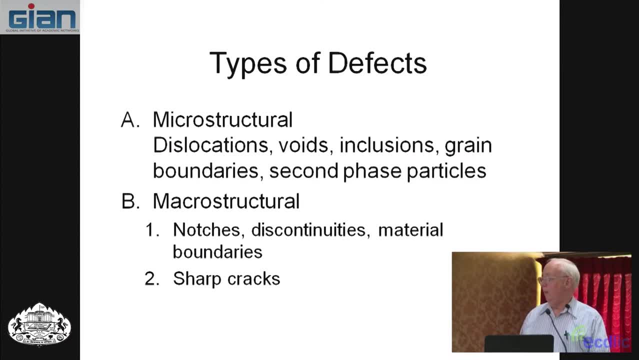 which puts together the stress and the defect size into a term called fracture toughness. So in this approach the defect is considered. Now here are a lot of types of defects, but in Fractured Mechanics, at least mathematically, we assume the defect is a sharp crack. 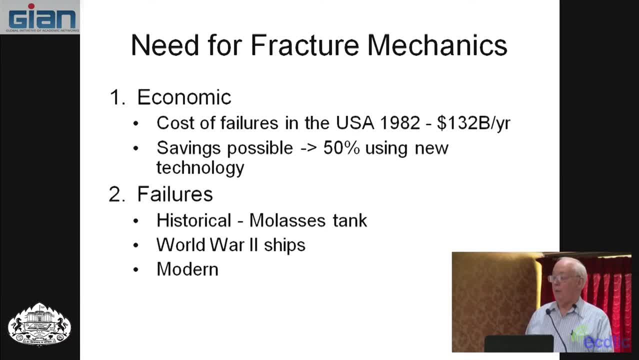 And so I want to do some apologetics, which is, tell you why Fractured Mechanics is the right approach. It's because the defect is not a state defect. It's because it's not a state defect or a cause or effect of a defect. 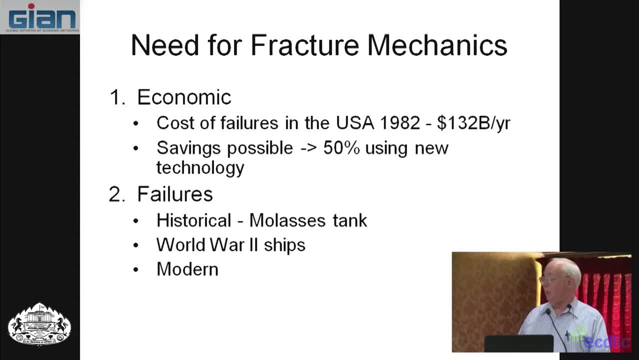 And that's the answer. It's the correct question. So let's talk about the defect. You know, how do you do that, How do you do that? How do you do that? Well, I think one of the things that's important to note is two things. 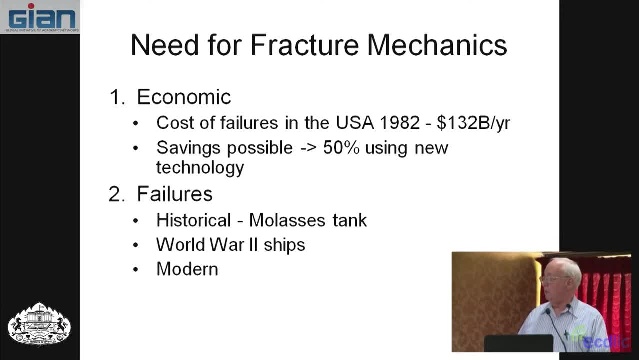 The first and the most important, And this is going to be the concept of non-reacting, because we're looking at structural defects and the difficult notions of the defect. So you know, the defect is not a state defect, It's just a state defect. 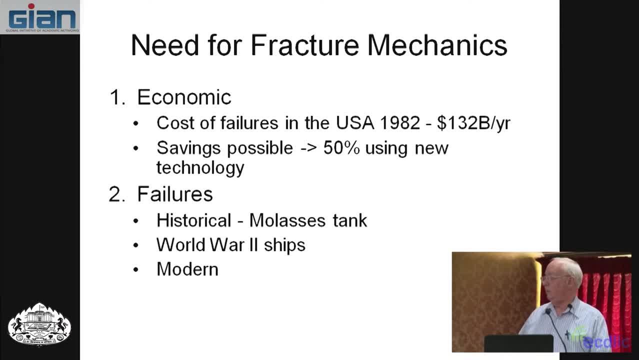 And it's not a state defect. And the second and the last point is that is actually in the range of a degree of a defect was more than $132 billion a year. Now, if you convert that to rupees, I don't know if I can do that in my head. 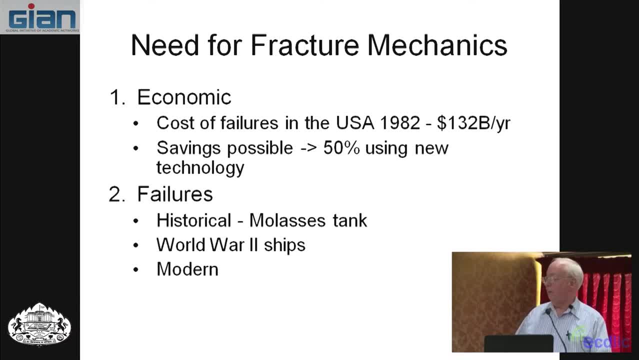 but it's probably more rupees than you can count. So that's cost of failures is a lot. The study also found that if people would use the newer technology, they could save at least 50% of that cost. Now, back in 1982, fracture mechanics was a newer technology. 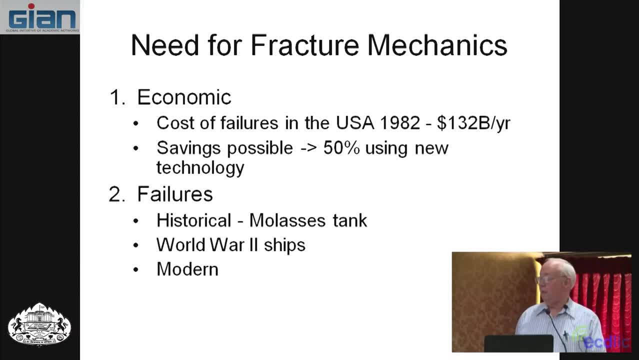 But in a lot of industrial centers it still is a new technology. Not everybody is using it yet. so people are learning more and more about it, And I do short courses on this around the US and always have a lot of students who are interested in learning this for their industry. 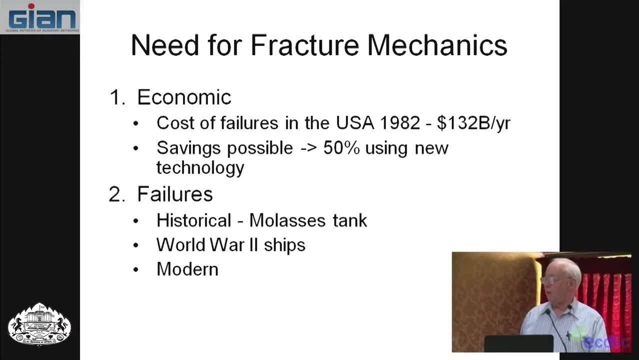 The other part of the need for fracture mechanics is safety And we like to talk. We talk about failure. Can't give any lecture in fracture mechanics without going back and talking about historical failures And some of them seem a little humorous today. but they weren't probably at the time weren't too humorous. 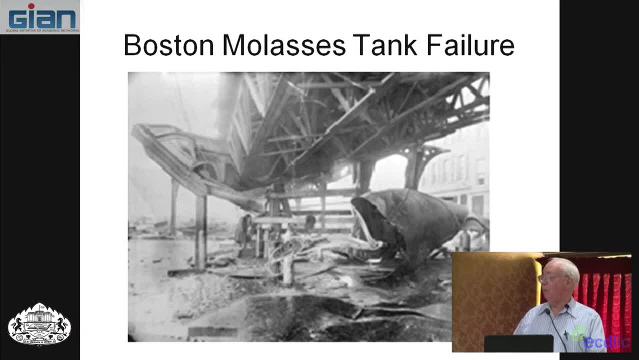 Here's: one of the real classics was the Boston Molasses Tank failure. This occurred in about 1919, so almost 100 years ago. in the city of Boston There was a molasses tank. It was a tank that burst and a wave of molasses came. 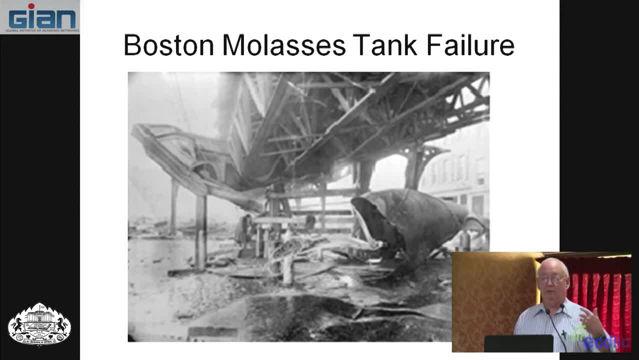 It's for those of you who do meters- it was at least 15 meters high, maybe higher than 15 meters or 5 meters. sorry, 15 feet to 20 feet high, And it came at a high velocity and just swept everything away. 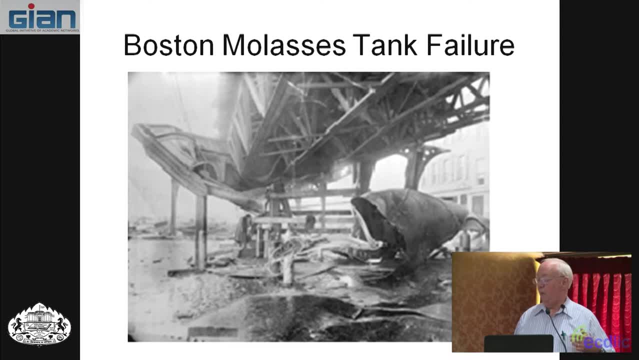 Killed scores of people and horses. Now I talked about molasses tank failure For quite a while. nobody knew at the time why it failed and can't really go back and study it. But I was wondering: why have a molasses tank in the middle of a big city like Boston? 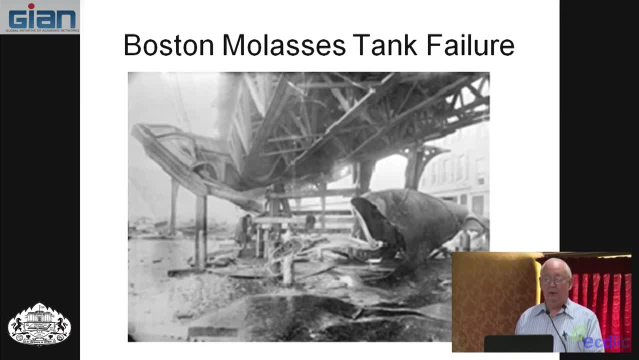 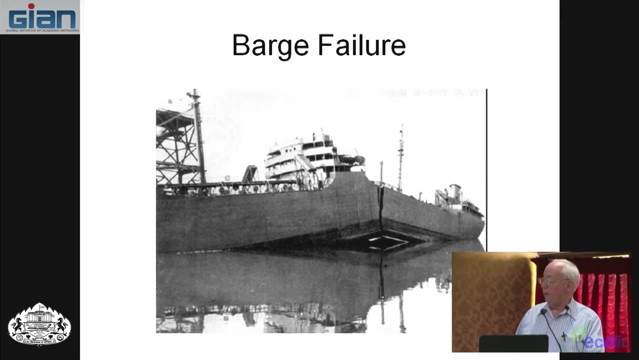 And found out that the molasses tank was there for the brewery. They were using it to make a beverage, And apparently they didn't make a beverage for a while after that happened. Here's another type of failure. This is a barge that broke, but it's not what I wanted to talk about. 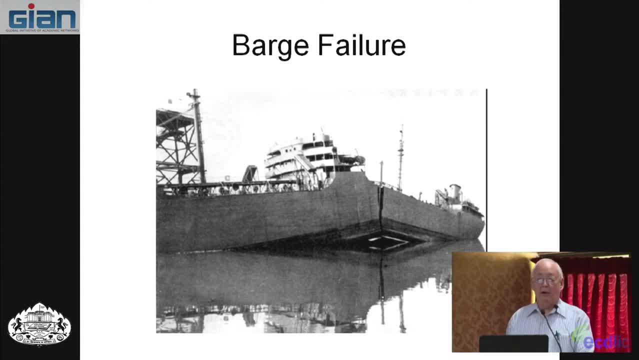 I wanted to talk about Liberty Ships. You perhaps don't know US history, but in US history the World War II started And they couldn't get supplies to the European front fast enough because there weren't enough ships. So they started building these things called Liberty Ships. 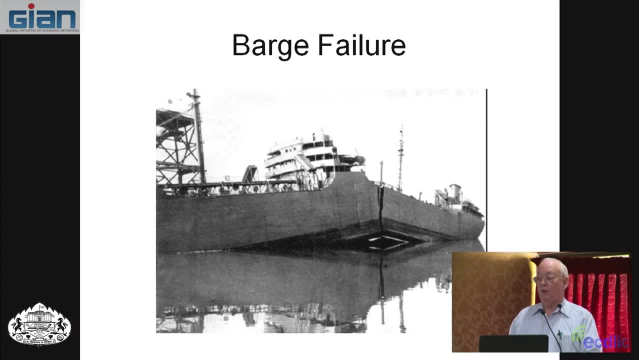 The Liberty Ships were a whole new design. It was completely welded, rather than riveted pieces. They welded it, so it was like one big structure And they built them fast. I saw a video one time that showed how they built one complete ship from nothing but metal laying around on the floor. 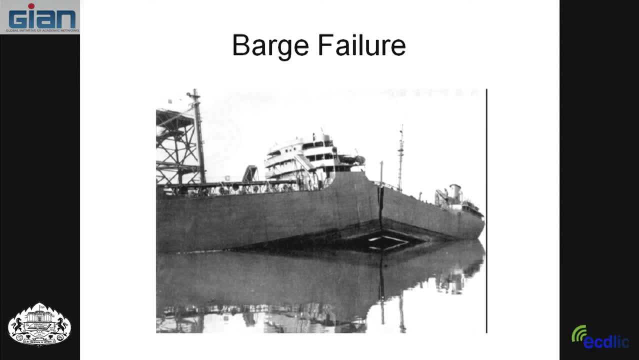 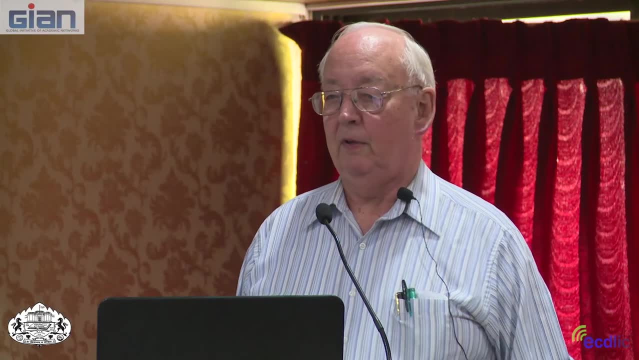 to a whole complete ship in about four days. So I don't think we could do it anymore. You probably can't call somebody up and get an answer back in four days, But they built the ship in four days And they built many of these ships. 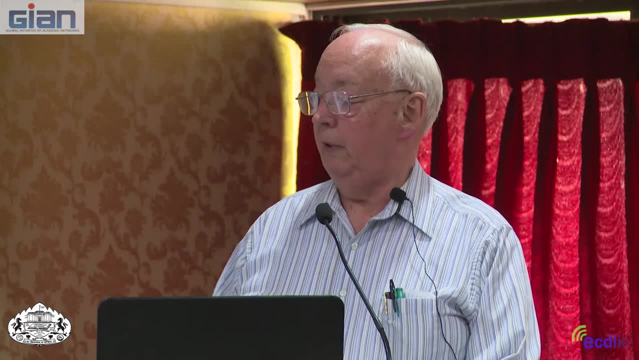 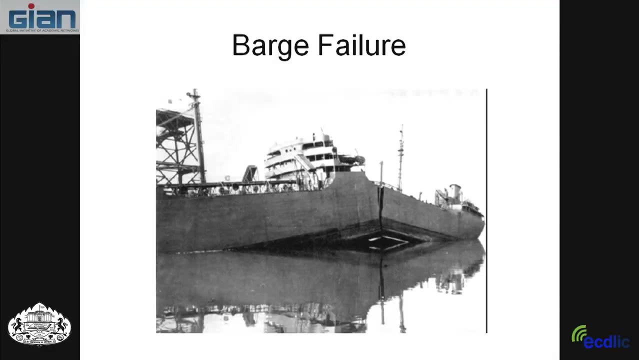 They built more than 2,000. And as they started to sail across the North Atlantic, where the water was cold, some of the ships failed. And of more than 2,000 ships, some 400 had bad cracking problems, some 90 bad cracking problems and some 20 of them had complete failure. 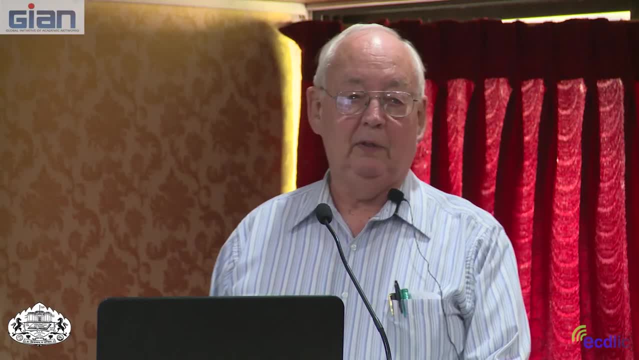 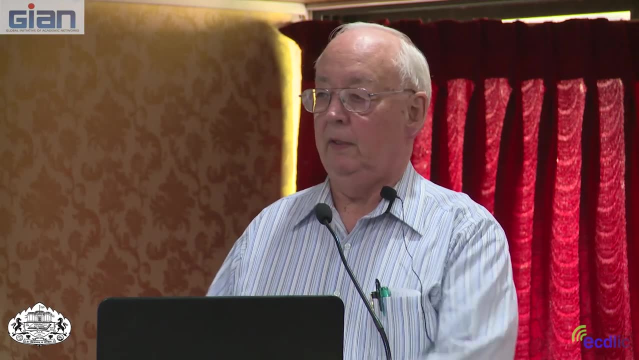 Complete failure was a little bit like the Titanic. If you've seen the Titanic movie that came around about 10 years ago or so and people saw that, how it broke in half and went into the water, these went down quicker. They didn't have a lot of actors there, sort of dragging out the failure. 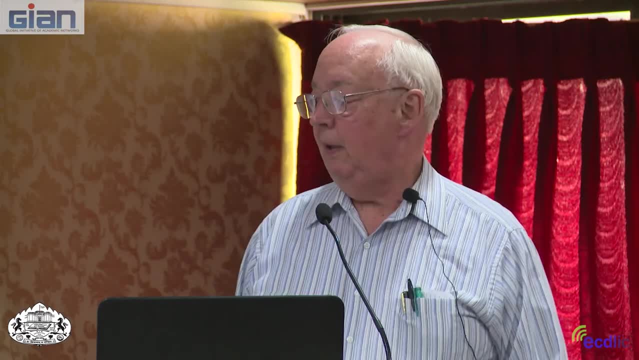 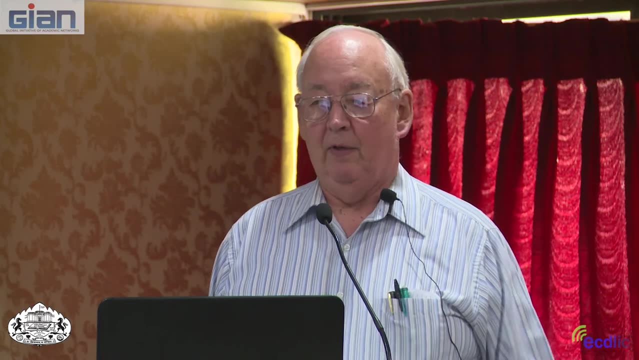 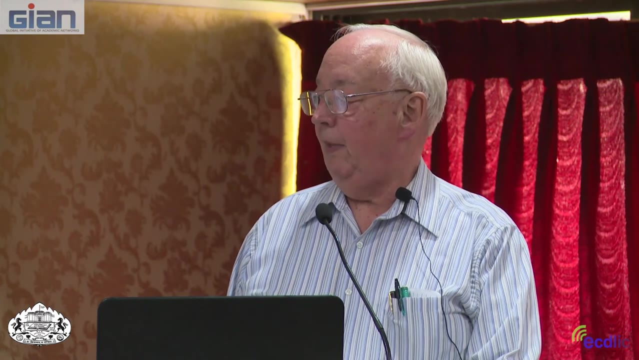 But broken too down in the ocean. You can imagine being on such a ship. you would have been very disappointed in the design and building of that ship, albeit for a short time maybe, But a lot of failures After they thought about it. it was a materials problem. 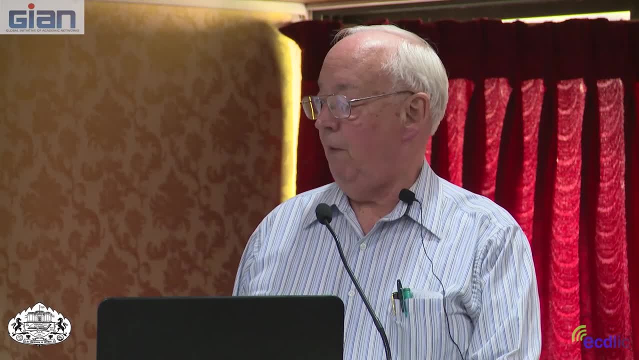 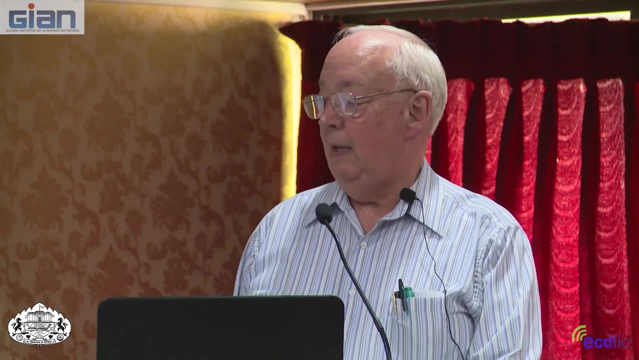 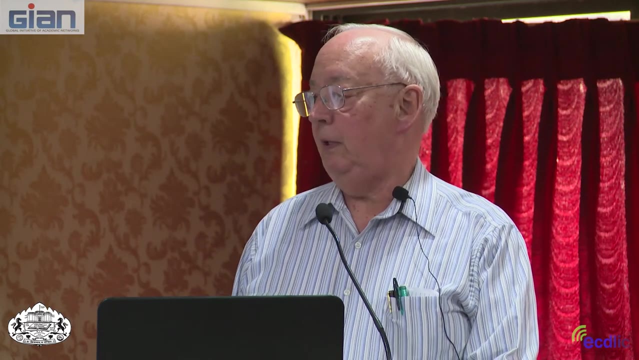 Nobody knew about fracture mechanics And they solved it by using the Sharpie impact test. Those of you in materials know the Sharpie impact test. They found if they had a material that had more than 10 foot pounds of energy, maybe 13, some joules- it was safe. 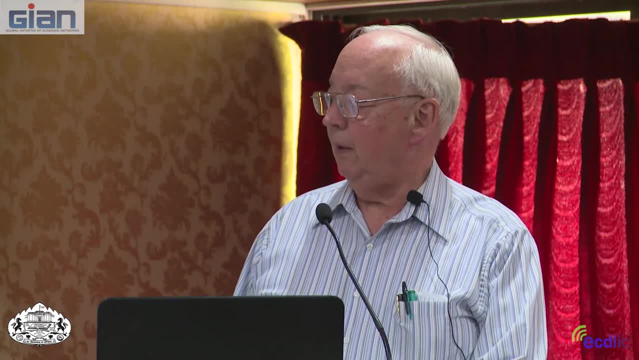 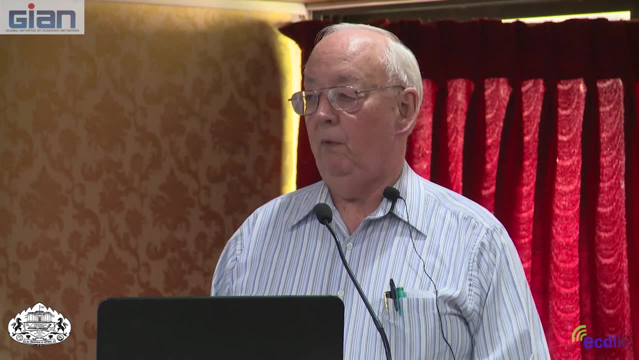 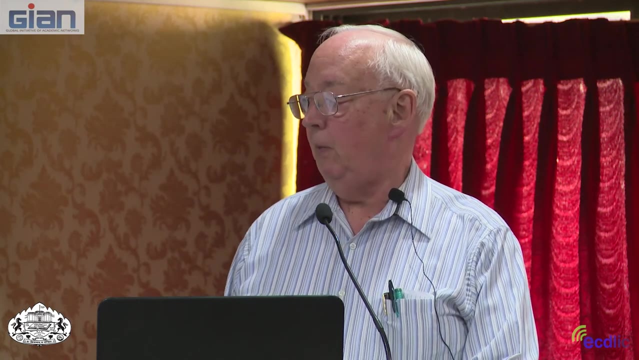 And so they used that. But the important thing about these failures were the Navy got very concerned about failures and fracture And the initial modern fracture mechanics approach started with George Irwin who worked at Naval Research Lab in Washington DC. So this got the Navy thinking about fracture. 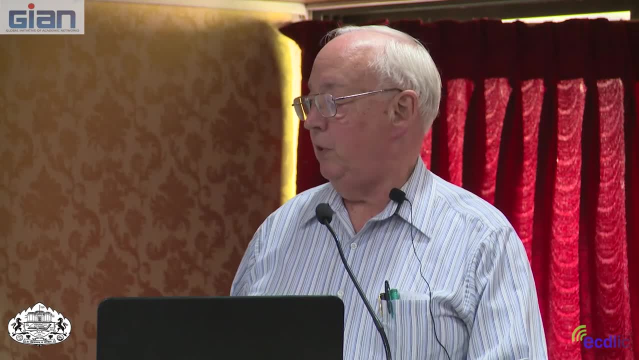 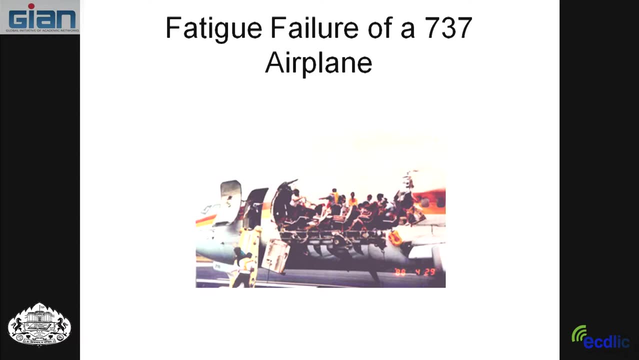 and really, really helped push that technology on Some more failures. These are a list of them. Here's one. I'll show you more. when it comes to fatigue, This is a failure of a 737 airplane. It was Aloha Airlines in the Hawaiian Islands. 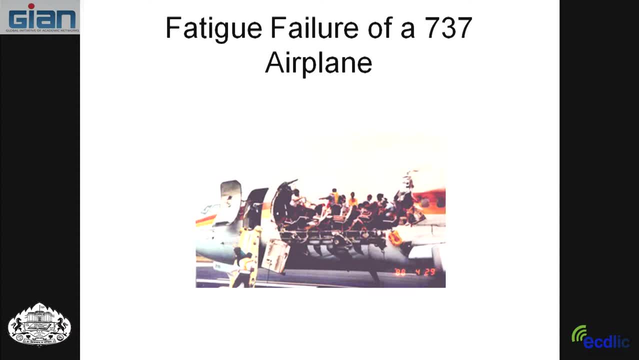 When they were flying due to a fatigue problem, the top just came right off of the fuselage And people were riding in what we would call a convertible airplane. Now in the US, when people have enough money, they get a real expensive car. that's a convertible. 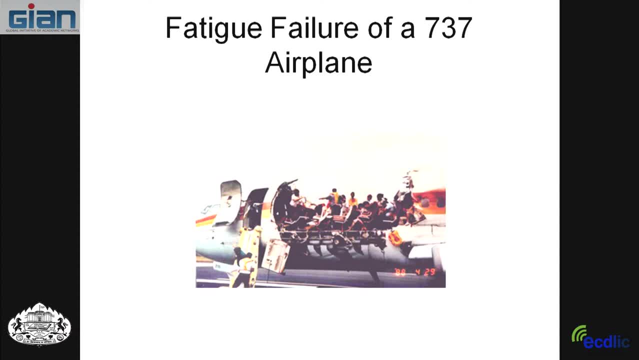 where the top comes down and they ride around with their heads sticking out. They have hair blowing in the wind And they really enjoy that a lot. The people on this airplane when the top came off didn't enjoy it one bit. The good thing about this was that the pilot was able to land it with only one fatality. 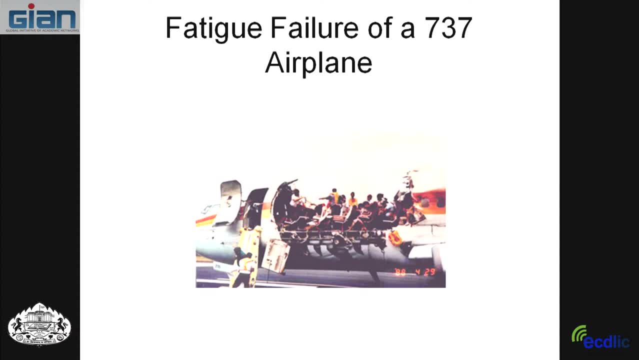 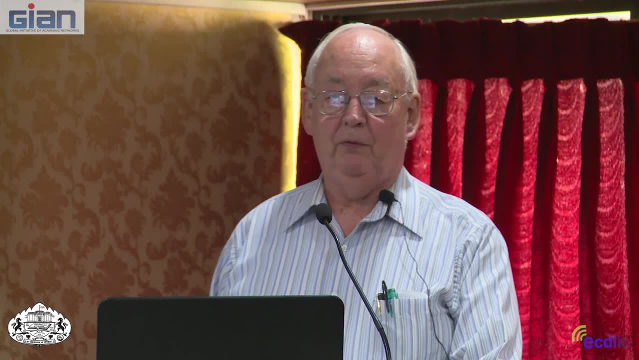 The fatality was- I think was a flight attendant who wasn't buckled in. So a good reason: when you're flying, keep your seatbelt on in case the top comes off. You don't want to go flying out. It's no fun at all. 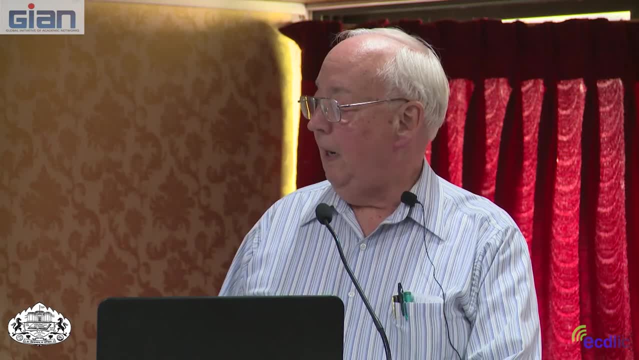 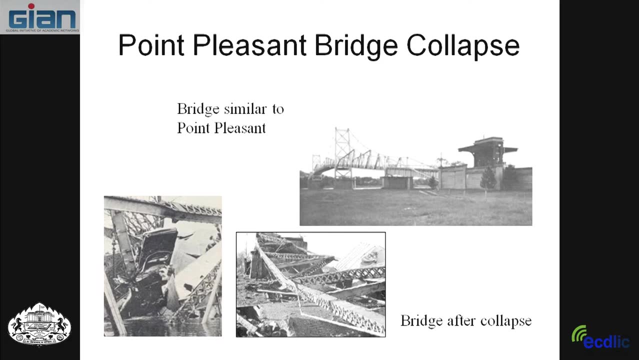 So that's another thing we'll talk about when we hit fatigue a little bit. Here was one failure that was well-known, And this was a bridge collapse in the US Point Pleasant Bridge, between Ohio and West Virginia, kind of in the northeast area. 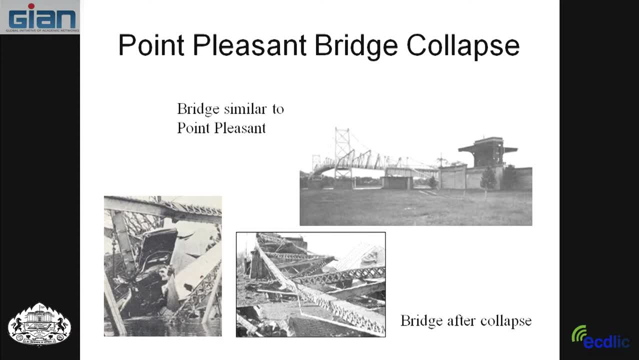 And it was due to an environmental cracking problem. We'll talk about environmental cracking later on in the week. It happened in the winter in December, just before our Christmas holiday. It was a big disaster And people involved with this. many people were killed because they had cars on that. 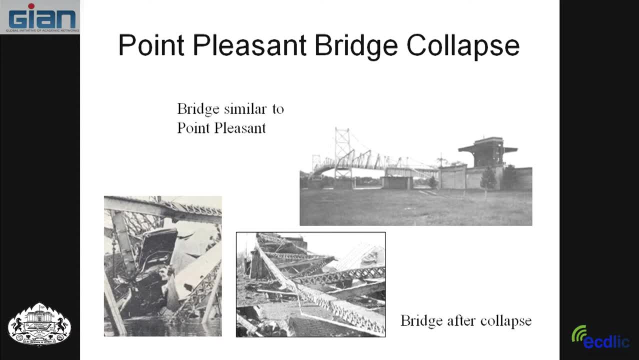 that fell into the river And it was a real tragedy for these people. So this is environmental effects and cracking causing that bridge collapse. This is not the bridge, but this is about what it looked like before a failure- Those pieces that were failed. 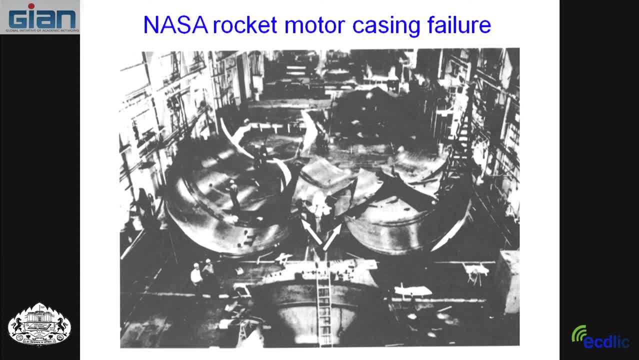 One last failure, I think, to talk about NASA rocket motor casing. NASA is our National Aeronautics and Space Administration in the US responsible for putting rockets into the air. What happened is that in the US in the 1950s, people talked about one day putting something into space. And then suddenly the Soviet Union put the Sputnik up, Sputnik first thing, And everybody in the US panicked And they got real busy and said we've got to beat the Soviet Union. We can't let them be ahead of us in the space race. 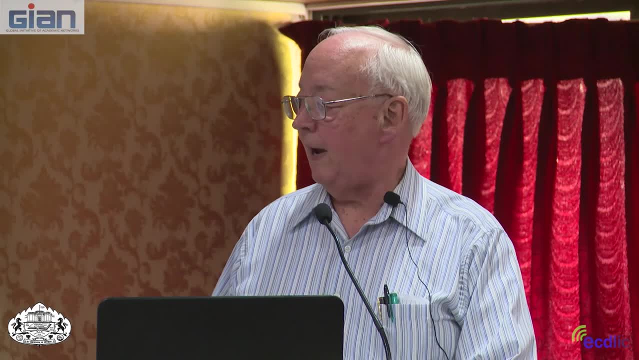 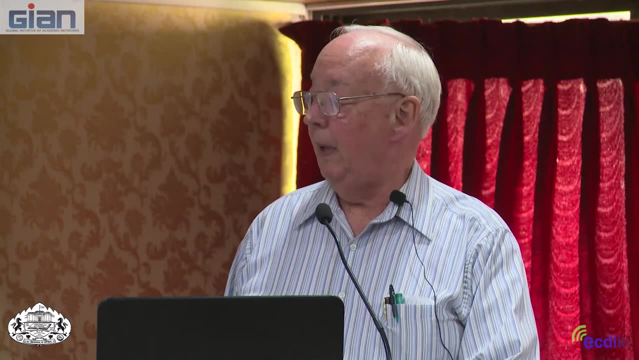 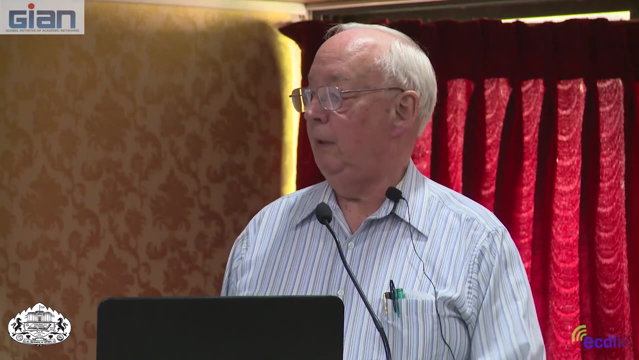 So they started building these sort of things very fast And they built them of materials that had fracture problems sometimes. So some of these rockets blew up And because of that NASA got involved in fracture mechanics And was very instrumental in developing testing techniques and the like. 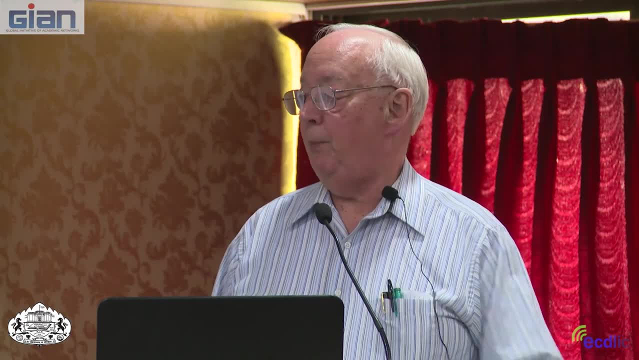 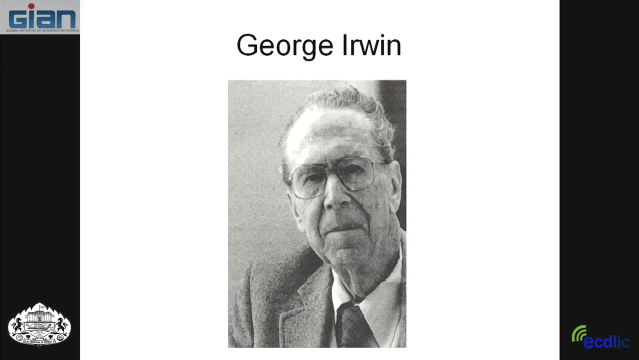 So that helped All of these failures, helped push the need for fracture mechanics along. I think this is- yeah, that's all the failures. This is the person we call the father of fracture mechanics, George Irwin. He was at Lehigh University while I was there for a little while. 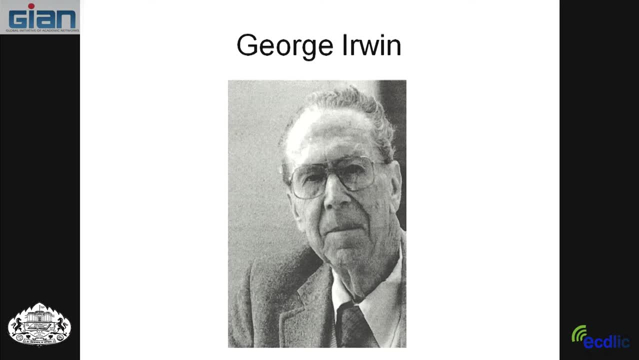 And he was involved with fracture mechanics. He developed the basic Stress approach to fracture And whenever I had students that went to a conference they always wanted to know if Dr Irwin would be there. If he was there and the students gave a lecture, he always came up and congratulated them. 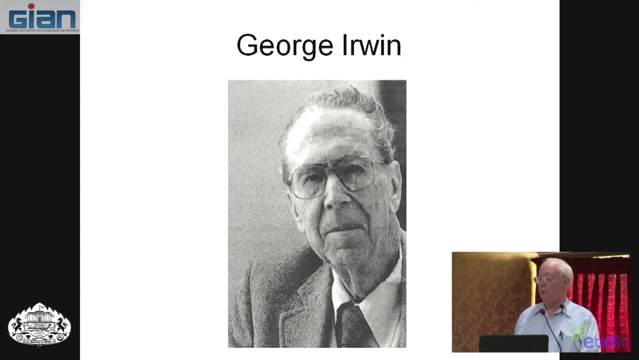 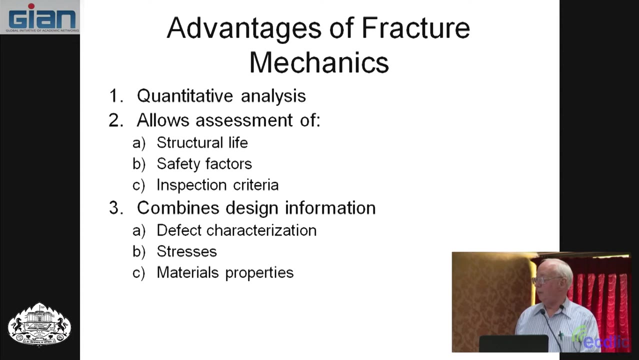 He worked in fracture mechanics area until he was about 90. And he passed away then some months later. Continued working until his death. Here's one last thing about advantages of fracture mechanics. It's a quantitative analysis. You can get actual numbers out of this. 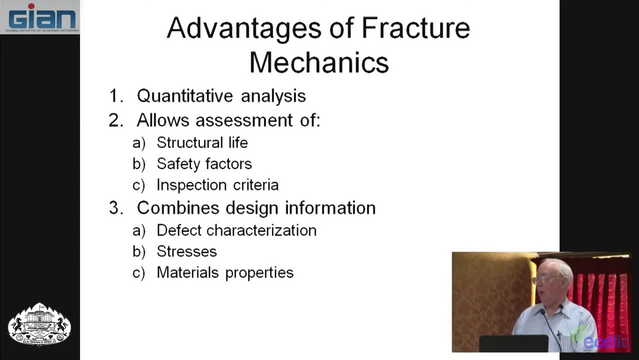 Instead of saying qualitatively it's okay or it's not okay, you get actual numbers about this. You can pick out structural life, design, safety factors and inspection criteria- The three areas that we combined. I'll show you a lot during these lectures. 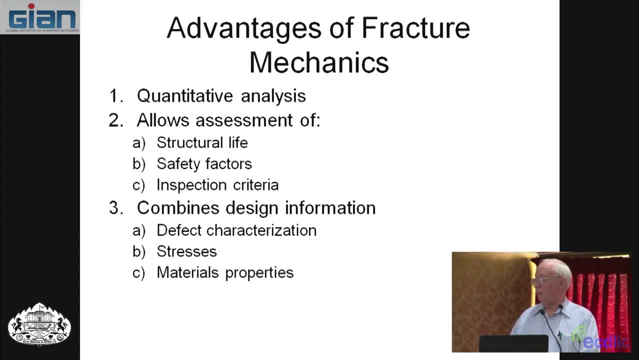 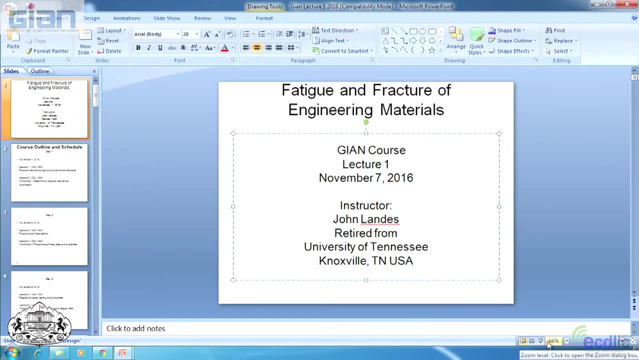 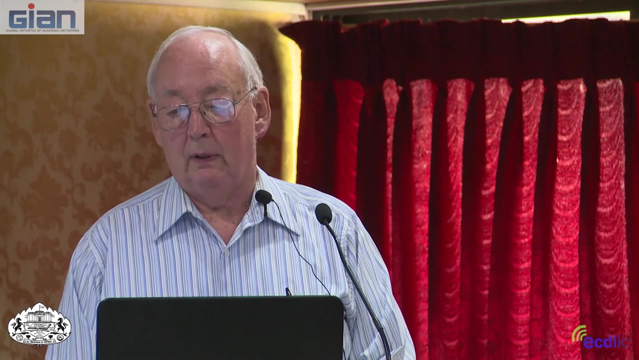 The defect size, the stresses and the material properties. So this kind of brings together the mechanics people, the metallurgists and the non-destructive inspection people. Okay, I'm going to go start the next segment. My lectures don't last exactly one hour each. 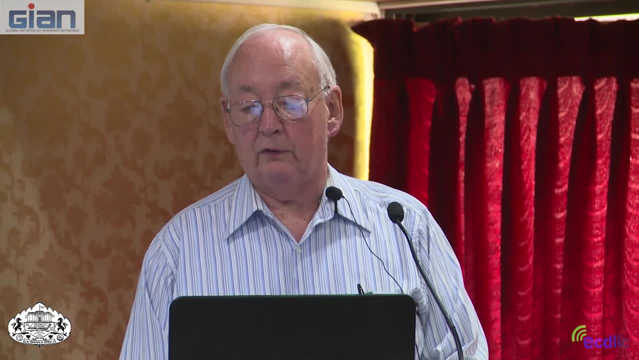 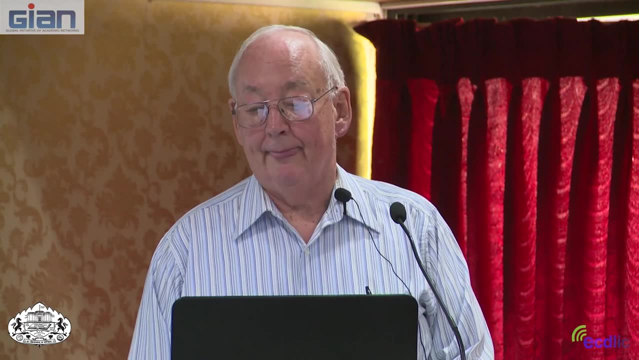 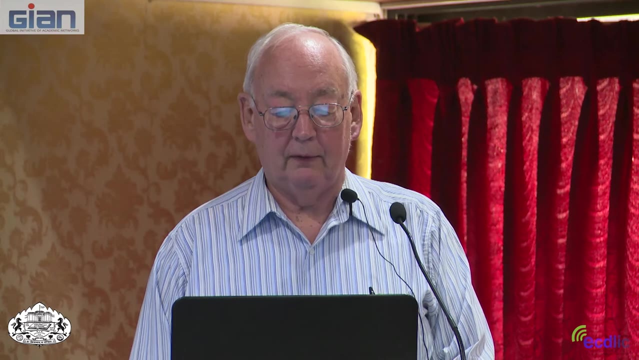 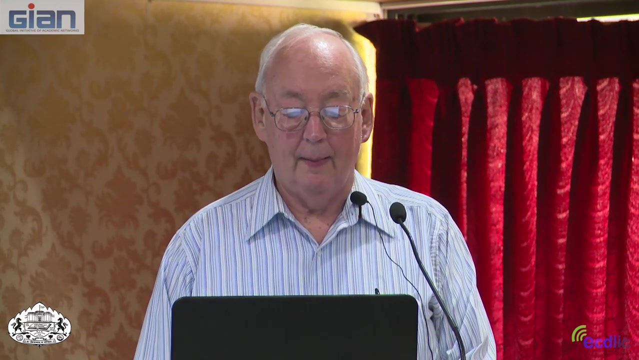 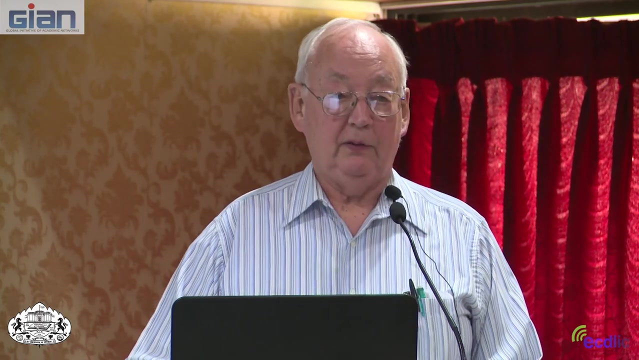 They are somewhat varied, So I'll find a nice stopping place when it comes time for that break, But I have to figure out this computer. Okay, So that's the arm waving part, where you hear the stories about failures and all the bad things that happen. 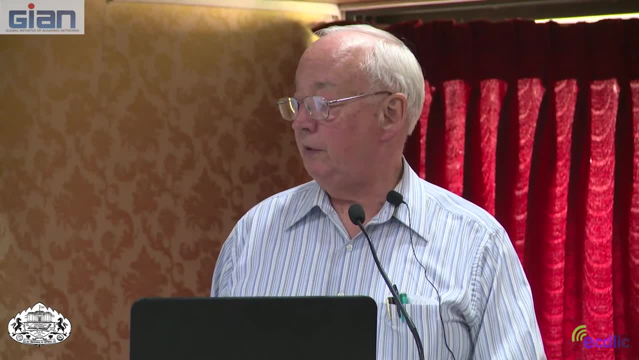 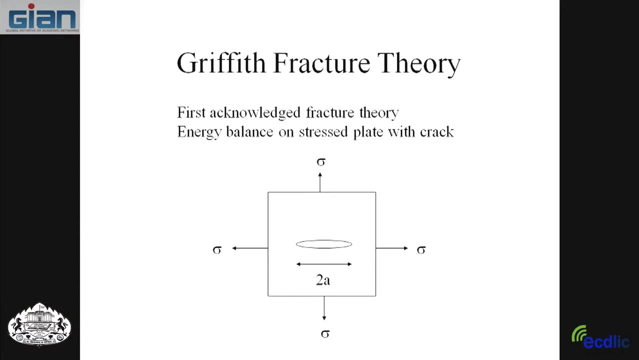 The fracture mechanics itself requires some analysis. So I want to talk a little bit about analytical techniques in this lecture. So start out with the very first fracture, The theory which is the Griffith's fracture theory. It was based on energy balance And he developed that in the 1920s but never really went anywhere. 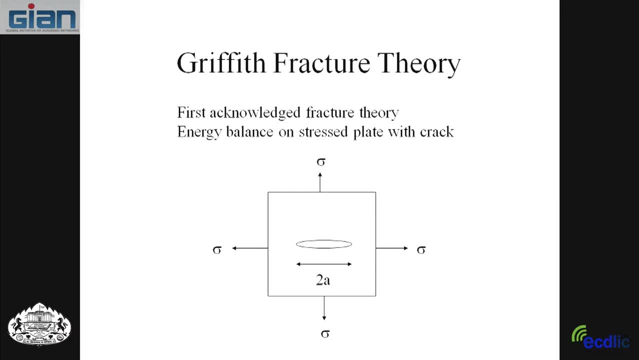 Because the energy balance approach was a little bit complicated and clumsy, And so people just never got anywhere with it. But I'll mention that his theory was this: Take a plate that is stressed by actually- And this is a two-dimensional sort of a two-dimensional thin plate- 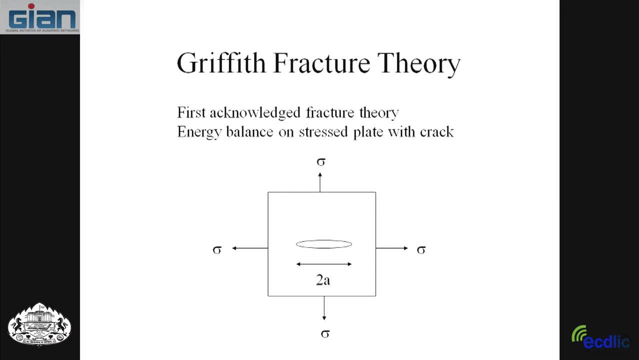 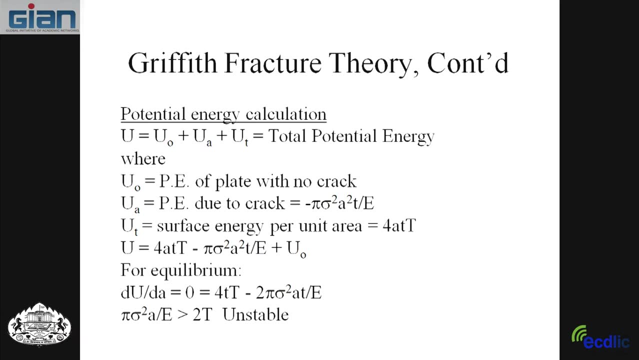 It has a defect, size 2A. It has stresses by axial, as I said, And then he developed the energy of this. So the potential energy of that plate had three terms And the first term U naught was potential energy with no crack. 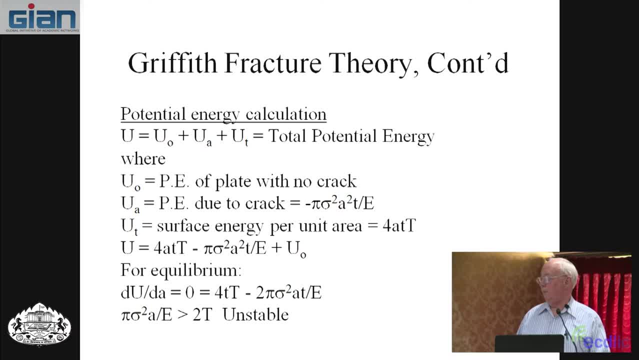 U A was potential energy change due to the introduction Of the crack, the 2A crack, And this solution came from an elastician named Inglis And said: this is really what would allow Griffiths to develop his theory. Anyway, sigma is stress by axial stress. 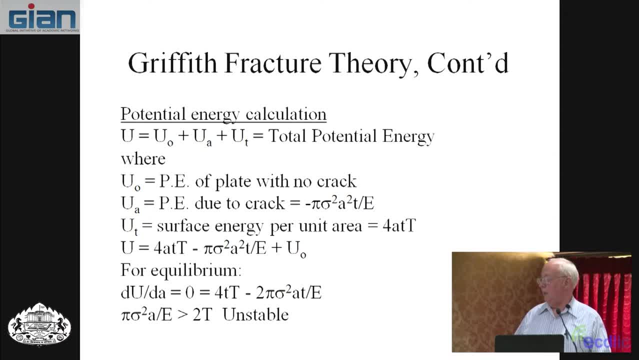 A, of course, is the half defect size, T is the thickness of the plate And E is elastic modulus. So all those terms come in And notice that the potential energy due to the impact The introduction of a crack is negative. 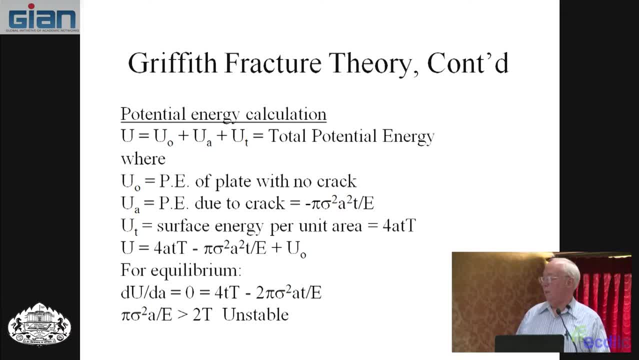 So if you start with this potential energy and introduce a crack, The total potential energy goes down. And then the other energy term is the development of new surface. So the surface energy term has this 4A times T times capital T. Capital T is sort of a surface traction term. 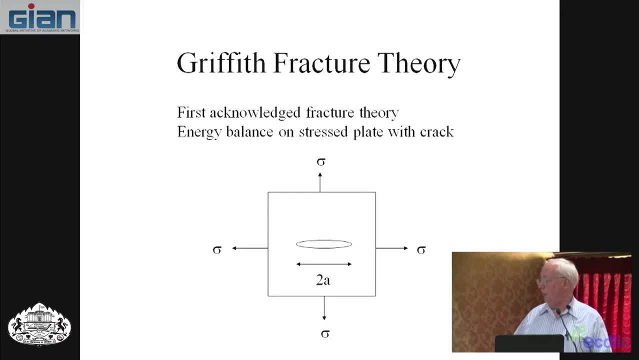 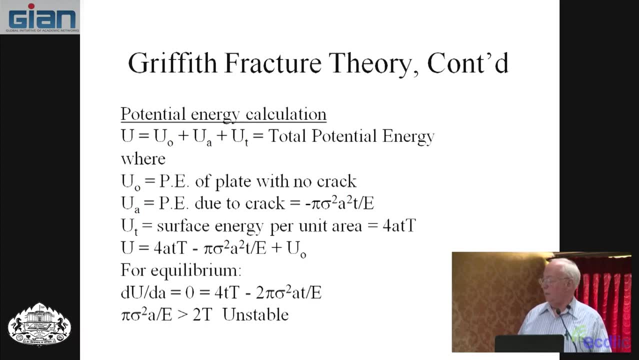 4A because You have 2A crack length and you have a top and a bottom. So you have a top surface, a bottom surface And a thickness gives the total area times the surface traction term. Then if you add them all together you get total energy, like that: 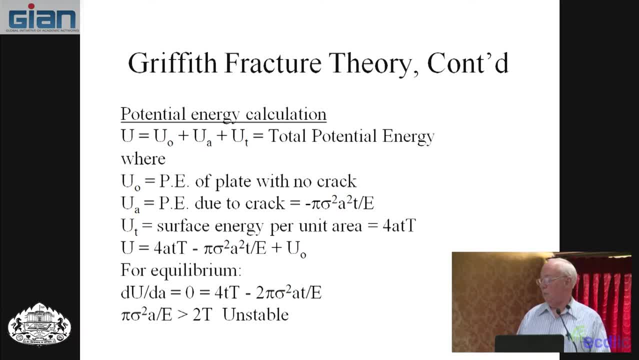 Now, if you take advanced mechanics of materials and courses like that, You learn that you can use an energy approach for equilibrium. The energy approach does this: You take the first derivative of the energy with respect to the variable and set it equal to zero. 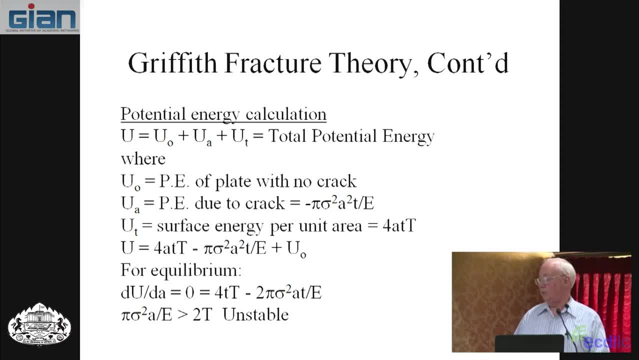 And that gives you the equilibrium position. So the equilibrium position is this: And if you take a second derivative and get a negative value, Which you would see, if you take a second derivative with respect to crack length, You would get a negative value. 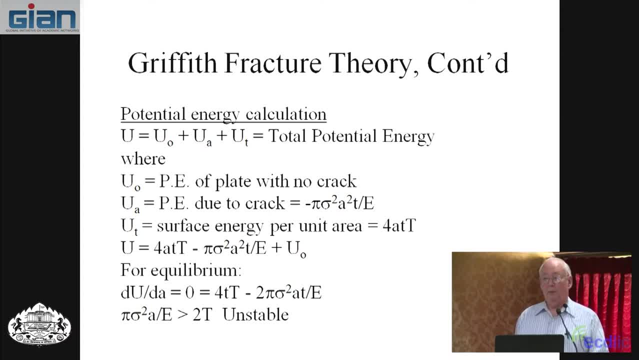 Then that equilibrium is unstable. Stable equilibrium is like having a ball in a dish: You push it up the side and it rolls back to where it was. Unstable is like having it at the other end of the dish. It's stable on top. 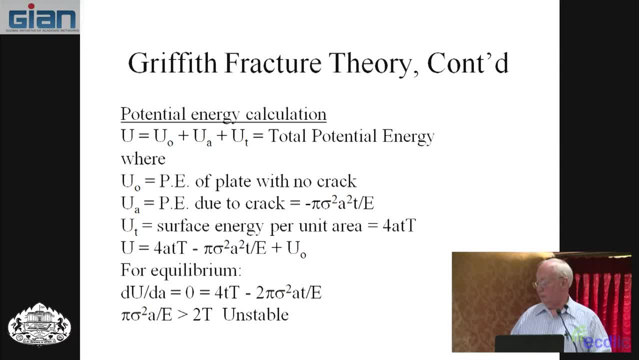 You move it away and it keeps rolling away, So that's unstable equilibrium. Now, that was the Griffiths approach And he said: this is what you need to cause fracture. It's a little bit clumsy, The people who work with Griffiths. 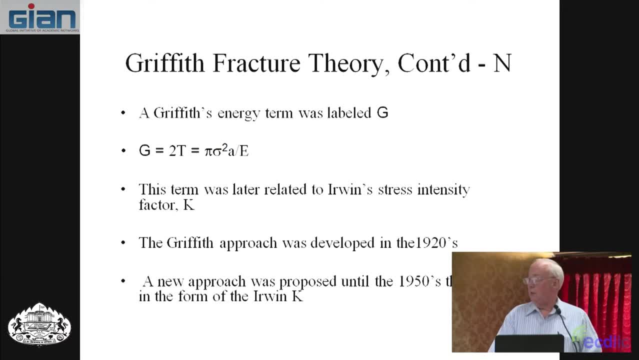 And it's still a valuable thing, Especially when you have materials that are not homogeneous And isotropic. Nevertheless, the Griffiths G was labeled like this, And later George Irwin came along And showed how this was related to crack tip stress intensity factors. 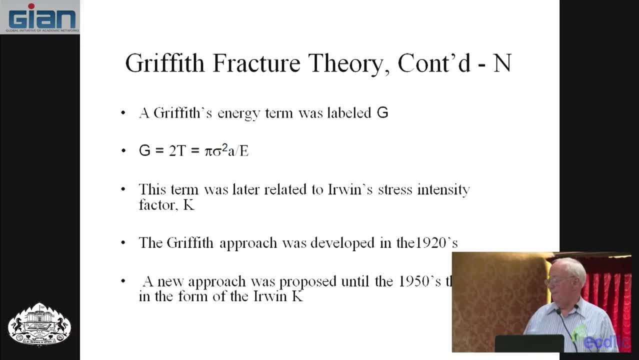 So the Griffiths approach came in 1920s. The new approach from Irwin came in 1950s, So more than a 30 year gap between those two And some of those failures I showed you Were the important in developing that. 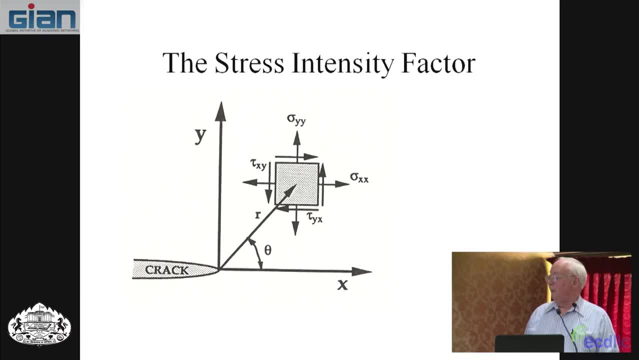 So that was an important thing. Now, the Irwin approach is a stress intensity factor approach, Based on stress rather than energy, And he showed that if you have a crack tip And look at the stresses around the crack tip, And this is two dimensional. 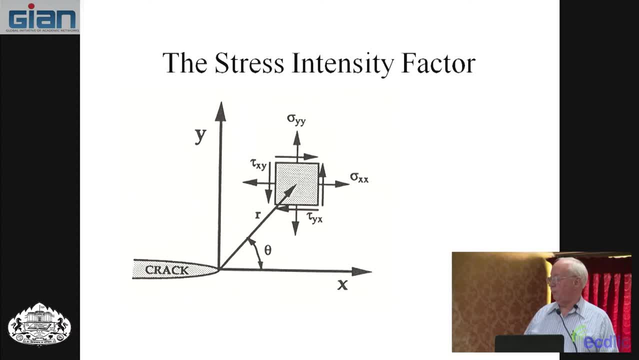 X direction, Y direction, Normal stresses and then shear stress, Tau, X, Y. That element then is at a distance R from the crack tip And at some angle theta from the horizontal. So those terms all come into the stress analysis terms. Now, before you look at them, 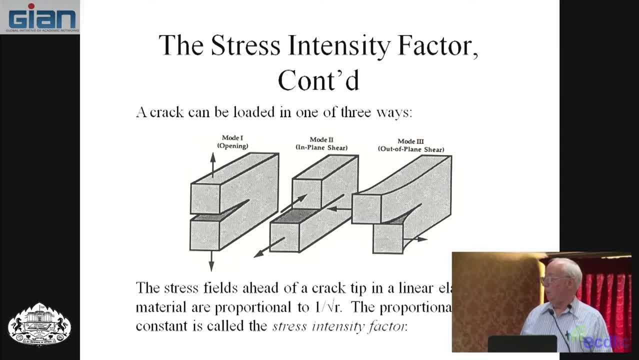 You have to talk about the modes of loading. There are three modes of loading. One is opening mode, And opening mode has all the loads and stresses perpendicular to the crack. Mode two is in plane shear. The loads are parallel to the crack. 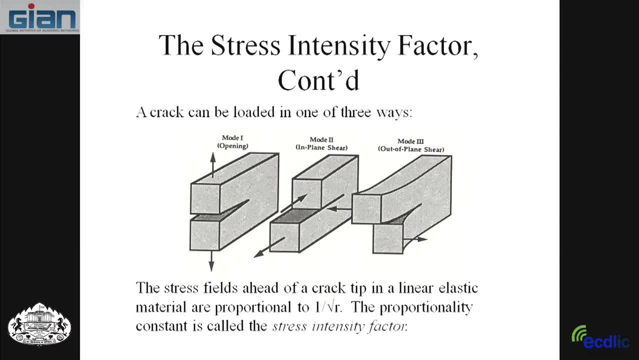 Loads and stresses, But they are in the plane And mode three is out of plane shear. The stresses and loads again are parallel to the crack, But they are out of the plane tearing the thing. This is what people used to use in the old days. 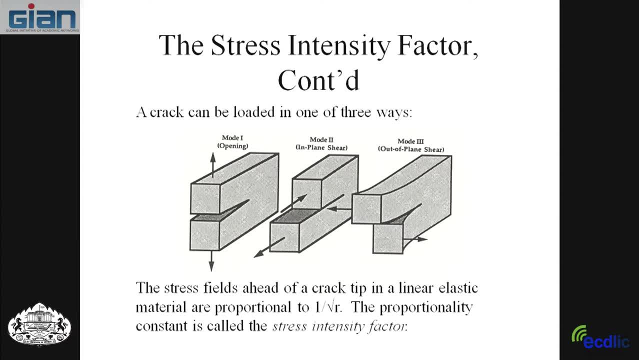 When they wanted to tear up the New York City phone directory. I don't know why they wanted to do that, But people did So. you use a mode three approach. 90% of what we talk about in fracture mechanics is mode one. 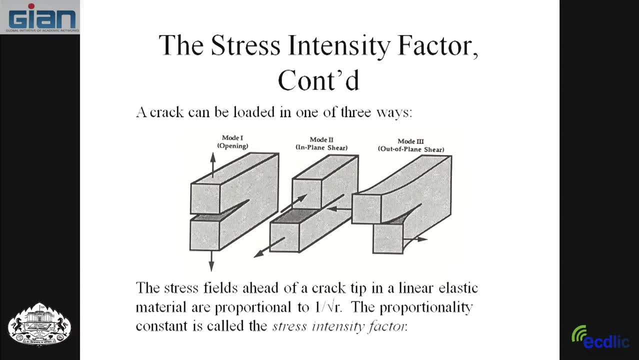 Opening mode. It seems to be the most damaging. Mode two comes of interest If you are familiar with research. What happens in research? People study something, They write papers on it And then, if it's not a real popular subject, it sits around. 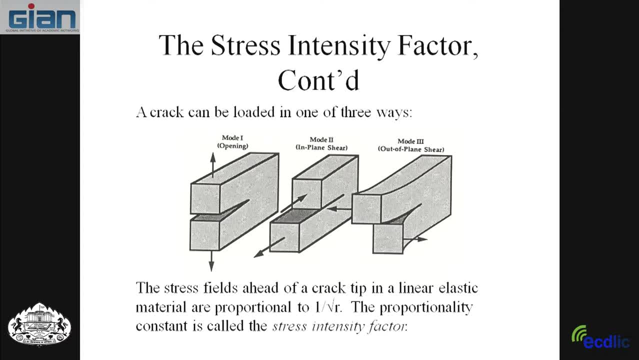 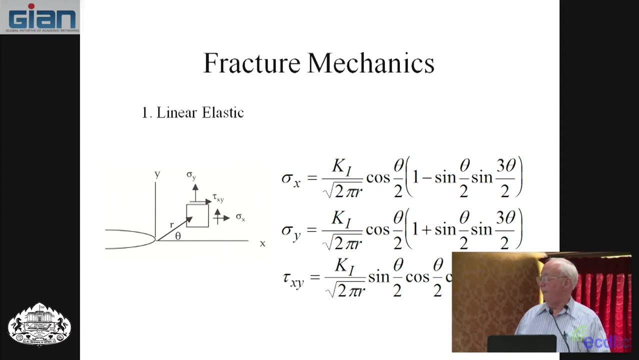 Fifteen years later, They study the same thing And write the same papers. So there's this every 15 year cycle, People doing the same work over and over again, And that's the way that one goes. Anyway, back to mode one. 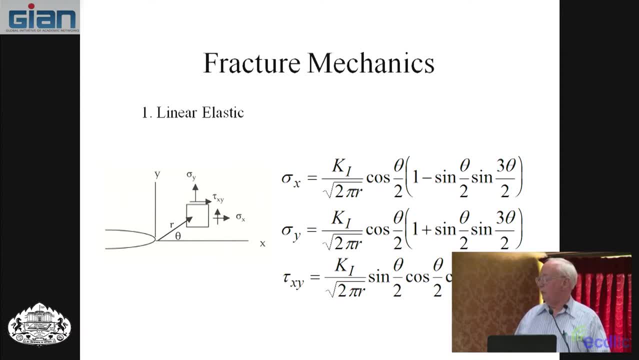 For mode one, loading At the tip of the crack, The stresses look like this: Not something that you should memorize. Nevertheless, the important thing here Is that these stresses Are unique distribution. The distribution terms Are the distance R from the crack tip. 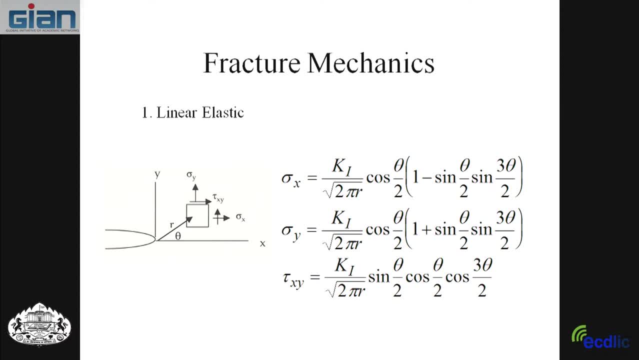 And the angle from the horizontal theta. So these distributional terms Are unique, No matter how you load, What geometry there is, If it's mode one loading, You always get the same stress terms, And that was an important thing in the fracture mechanics. 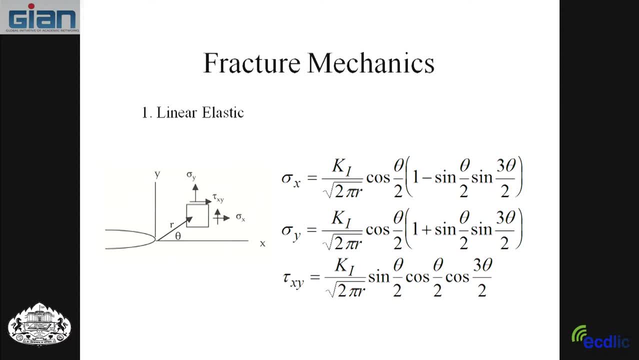 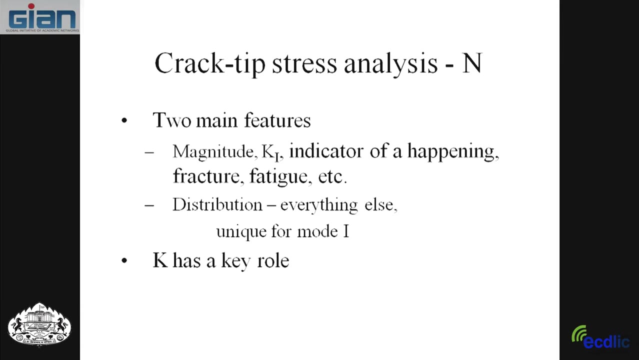 The important parameter then, Is the K- And George Irwin called that- Crack tip stress intensity factor. That is the term that relates The boundary loading To the crack tip stress And gives the magnitude of the stresses Around the crack tip. 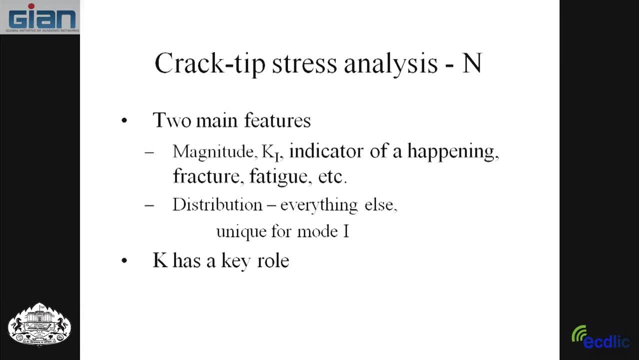 So in the stress analysis The two main features are the K, The magnitude term. It's an indicator of what happens In fracture, fatigue and whatever, And then the distribution terms Are unique For mode one, So K has an important role. 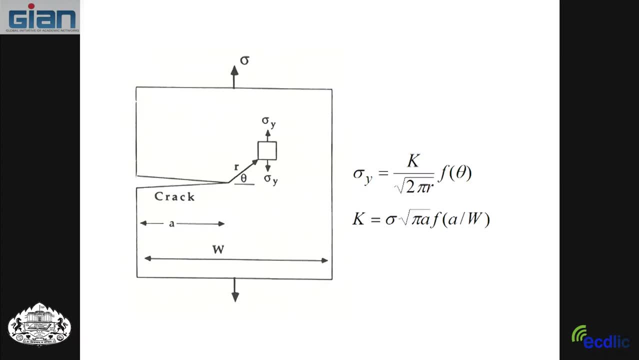 And we're going to get into K's In this lecture. So here's kind of How The terms look. The stress in the Y direction Has a K And, in these terms, Square root of two pi R, R being the distance from the crack tip. 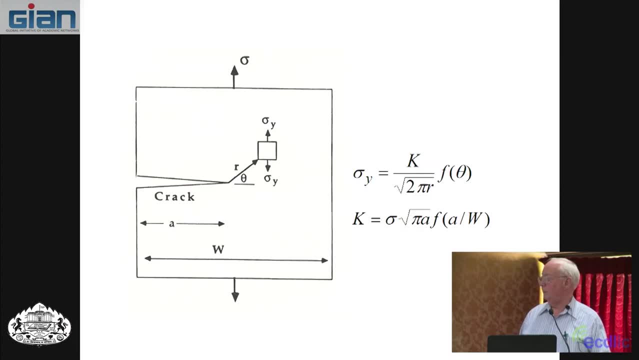 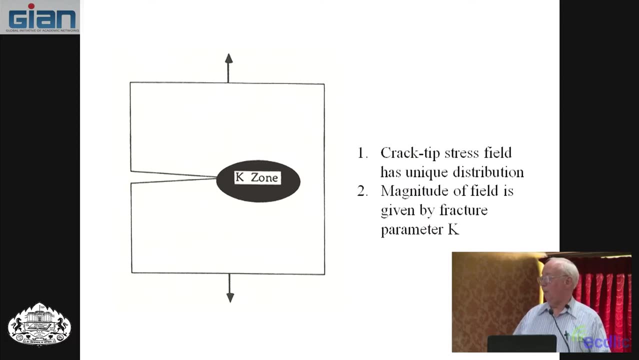 And a bunch of theta functions. All these theta functions In doing Fracture mechanics. then People look at The area around the crack tip As a black box, Because there is a unique distribution. There is a zone around the crack tip. 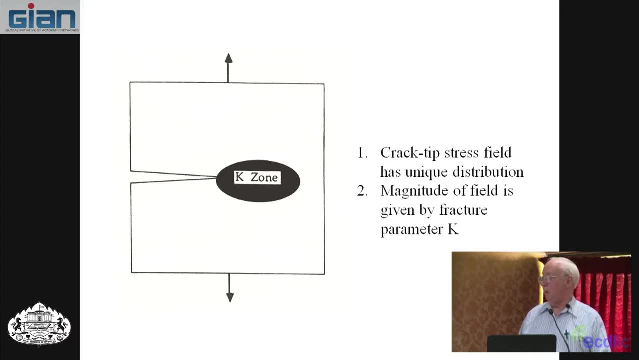 Characterized by K. That tells you What's going to happen. That zone is not given a size, But just as an area Around the crack tip And the magnitude of the field, Then given by K And the magnitude of that field. 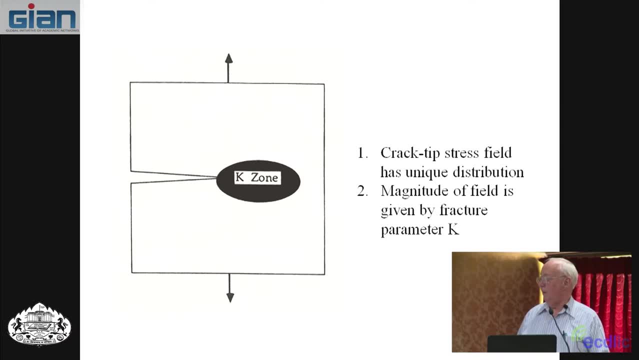 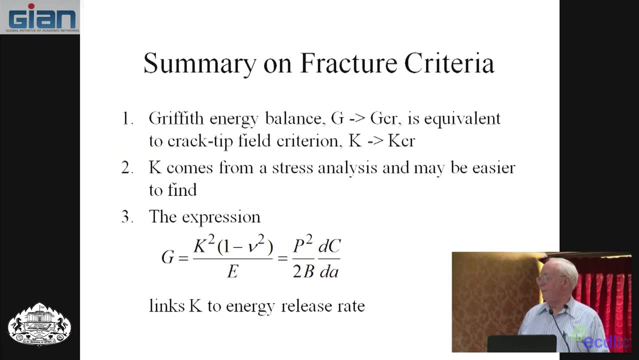 That's the fracture you would get, Whether you're going to have Fracture, toughness, Failure, Fatigue, failure Or environmental effects. However, When Irwin developed that approach Based on stress, Griffiths also had the energy balance approach. 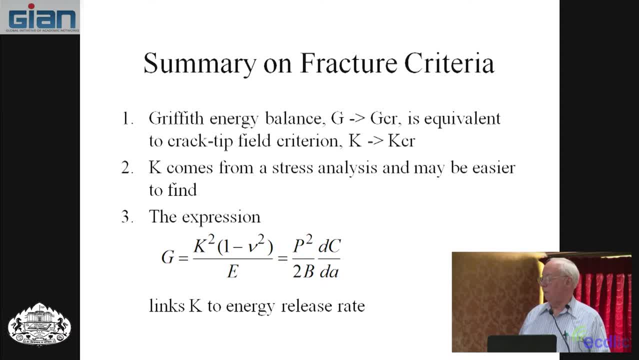 And so George Irwin did this. He showed that the Griffiths term Was related to the K. So Whether you use the Griffiths approach Or a K approach, You have essentially the same analysis. However, In most analysis, 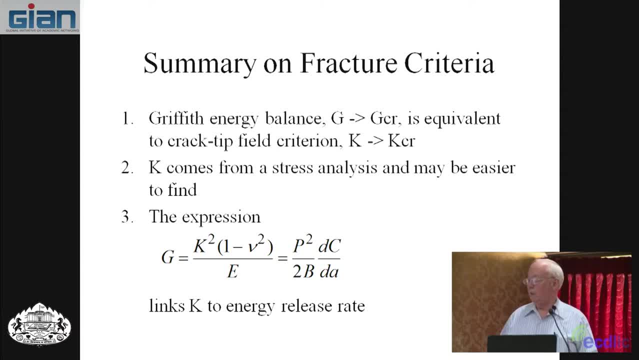 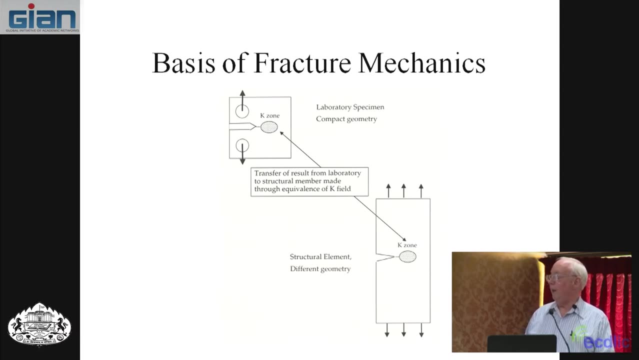 It's much easier to calculate stresses Than it is energy. People use Theory of elasticity Or numerical methods To calculate stresses, And then it's easier to calculate the stresses. So Here is what you can do With the Griffiths approach. 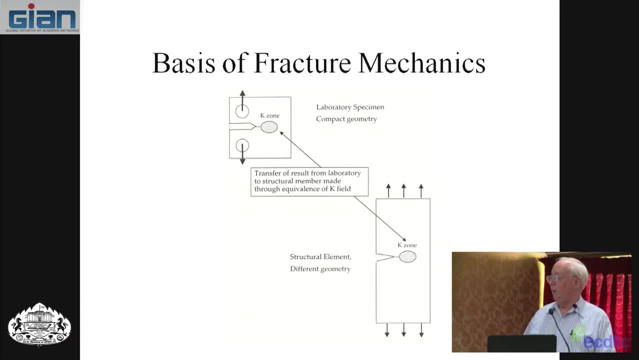 It's kind of the real basic Fracture mechanics theory. You can go in the laboratory And use a specimen. A lot of our specimens look like this. In the laboratory You use that specimen And then, if Whatever fracture event happens, 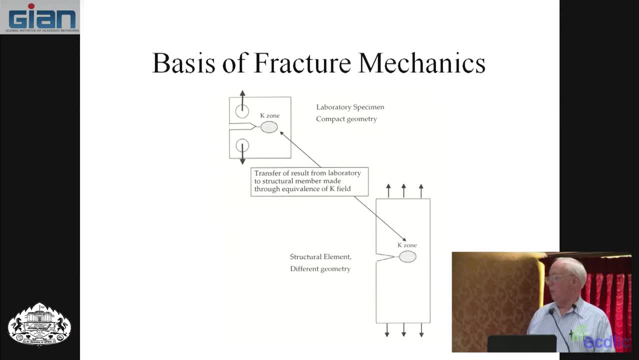 To that specimen. You can relate that directly To the structure And this is representative Of a laboratory specimen Related to the structure itself. And this is the transfer term then. So the K And the K field Is the transfer from laboratory. 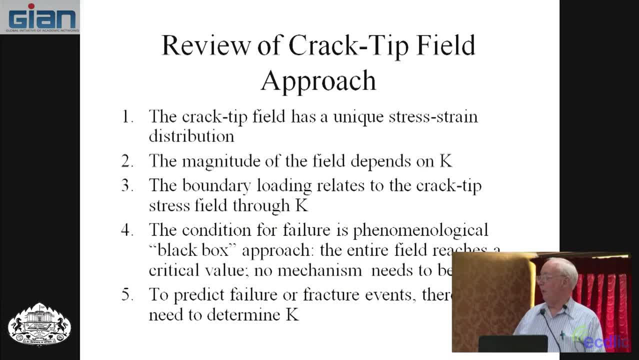 To structure. So here is In some words About what I just said. We use the crack tip field approach And the magnitude of that Depends on K And the boundary loading Relates to crack tip stress field Through K. 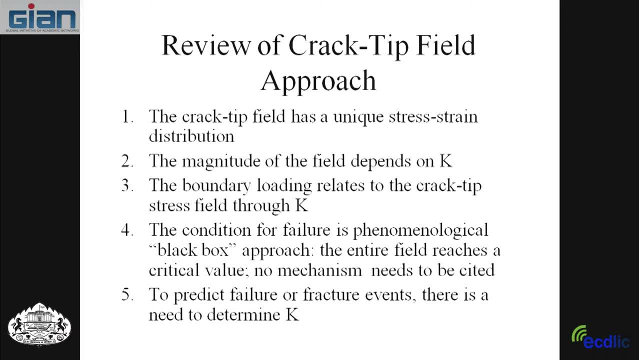 Which is phenomenological, Meaning that It's the field reaching a critical value Rather than a mechanism. So you don't say You get failure when stress hits a certain value, Strain hits a certain value, But rather When K hits a certain value. 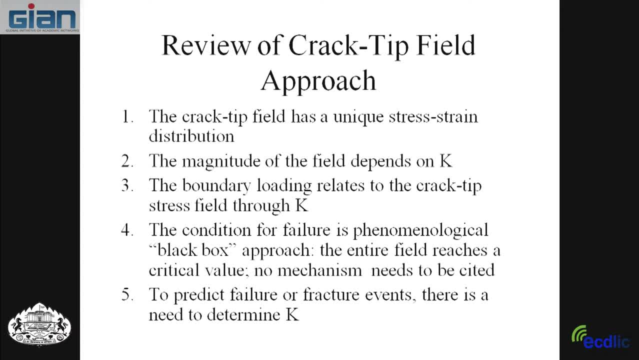 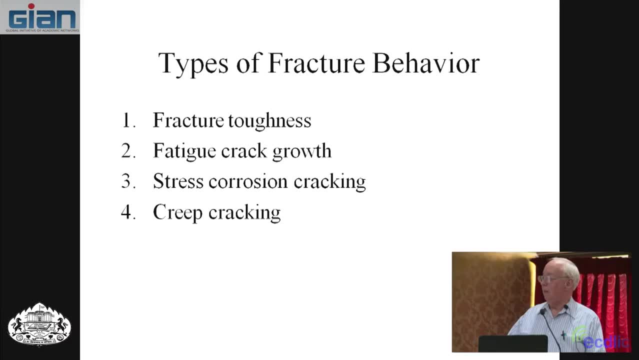 So, in order to predict failure, K is a real important term To use. The type of failures Can talk about. then, Fracture toughness, Which is failure under A monotonically increasing load. Failure due to fatigue, Which is under cyclic load. 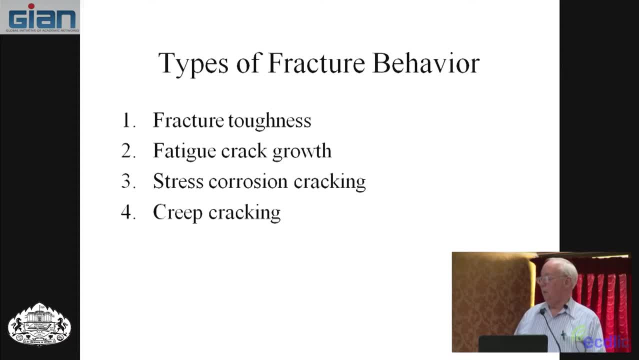 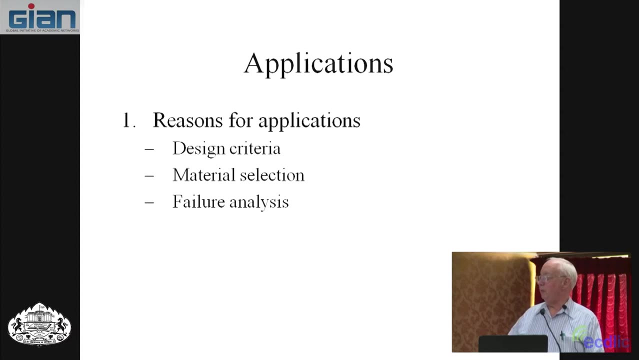 Failure due to stress, corrosion, cracking, Which is The combination of a bad environment With stress and cracks. And then, if you work on high temperatures, Sometimes people worry about Creep cracking. Here are some reasons For doing applications, The two main ones. 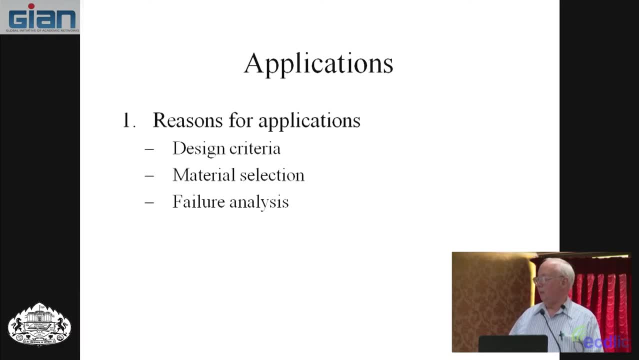 One is to set design criteria And the other one To set material selection. Anybody who is not very good At one and two Often ends up doing number three, Which is failure analysis. So failure analysis Is a fairly big topic. 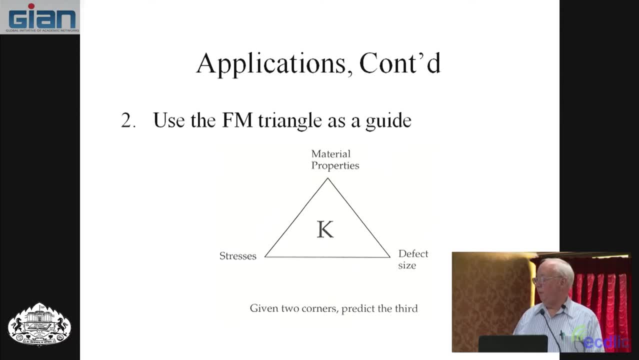 And can be approached With a fracture mechanics point of view. We put the different areas That are Involved in fracture mechanics On a triangle And they are: the defect size From the non-destructive people, The stress analysis from the mechanics. 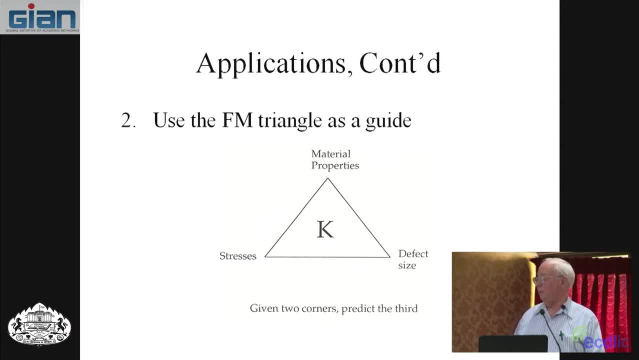 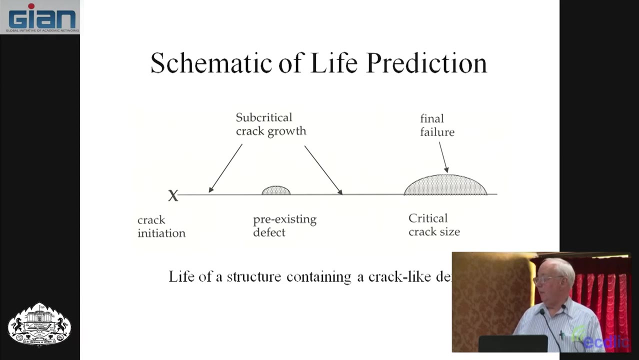 Or mechanical engineering, And then the material properties From the metallurgists and material scientists. They all go together Through K, The crack tip stress intensity factor. The life prediction Can be done this way For fatigue or corrosion That you could initiate a crack. 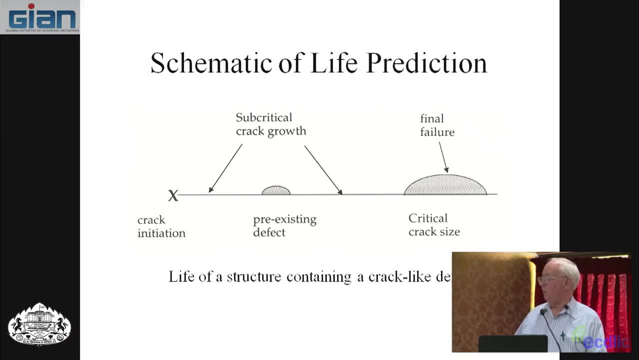 Or have a pre-existing crack And that could grow Due to some sub-critical crack growth mechanism And then reach a final size. So in my lectures During this week I will show you How to put that all together. So, due to this, 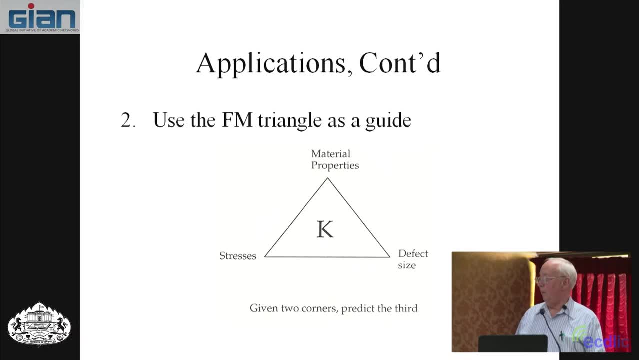 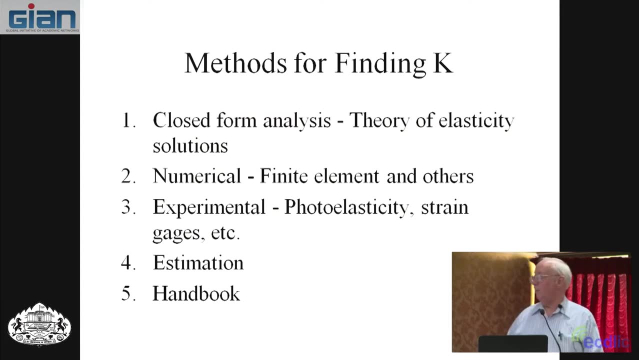 K Is the most important thing To develop, And we want to talk about Finding K For the analysis And the things we are going to learn. So here are some of the methods That we have used In the beginning. 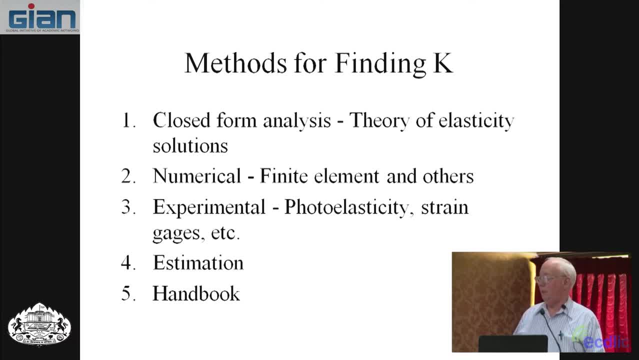 People used closed form analysis, Theory of elasticity, But that was fairly limited. Nowadays numerical Like finite element is used a lot. But more than anything Is the handbook approach, And I have- Everybody has these fracture handbooks With K solutions in them. 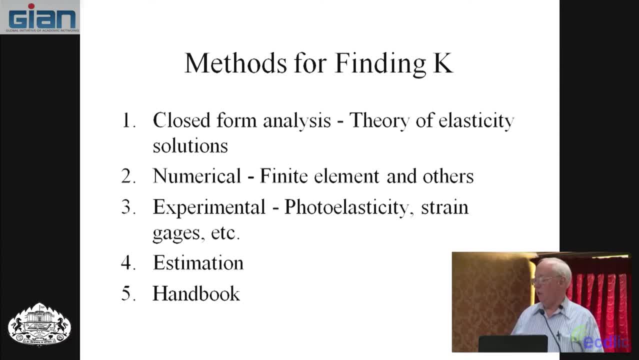 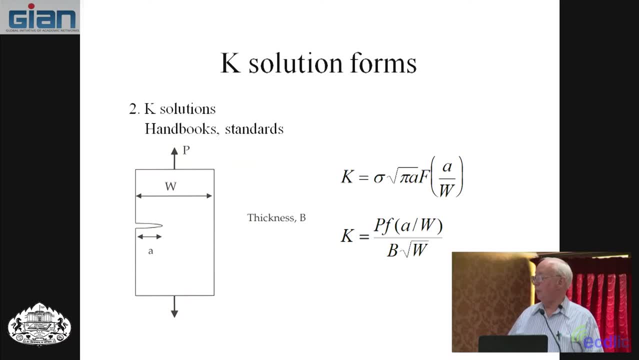 There is something That I will show you Some of the important parts of that. Here are some of the K solutions That you would use. There are essentially Two formulas, And these are Sometimes confusing people. One is given If you are given a stress. 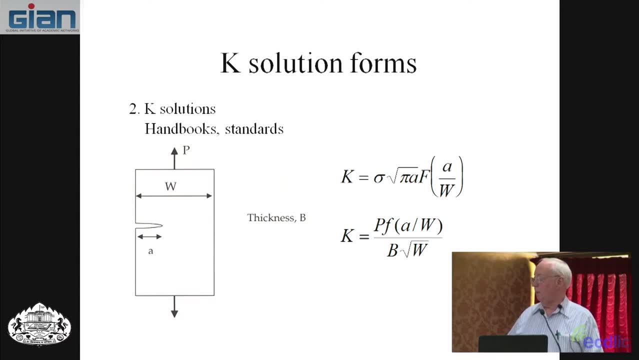 For a material, Then stress: Sigma, Spirit of Pi, A And a function Of the geometry F of A over W Does not mean F times A over W, But means a function of A over W. The other one is: if you are given: 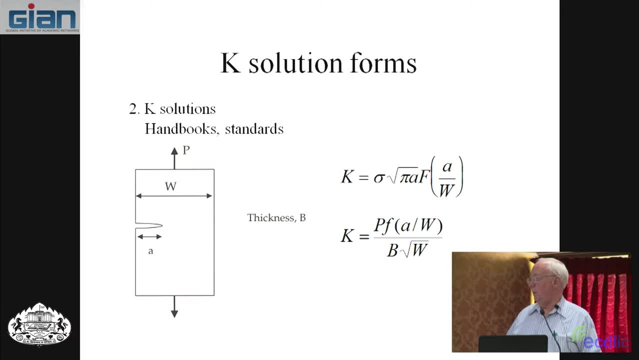 Mainly the load. Then you use the load, The little f, And these terms: B here is thickness Out of plane, W Is the planar width And A is crack length. So those two approaches, The little f approach. 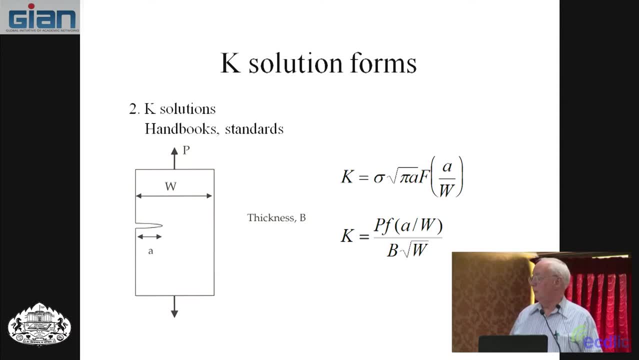 And they are both Important things. This is more used In structural analysis. This is more used In experimental work And laboratory work. Here are the Units used In most of my things In the US. I usually use engineering. 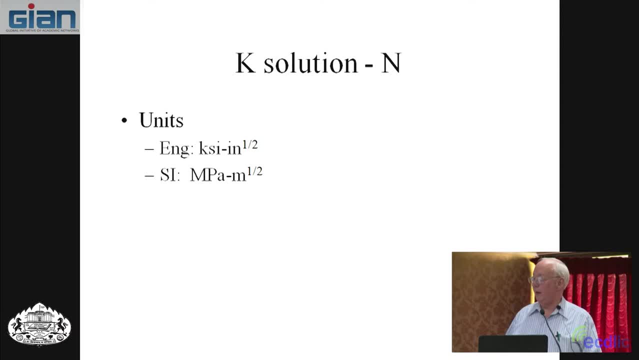 Or English units. I changed most of the problems That I could To SI for you, But I didn't do all of them Because some of them were on graphs That I couldn't change, So you should learn both of these. 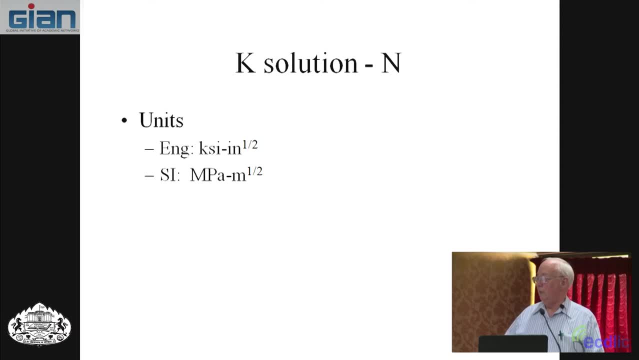 KSI Square root of inch. For engineering or English units And for the SI units, MPA Square root of meter. Sometimes people ask me What is length, Inch squared is area And so forth, But what is the square root of an inch? 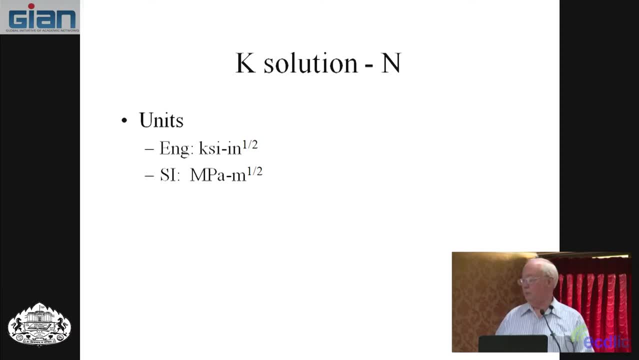 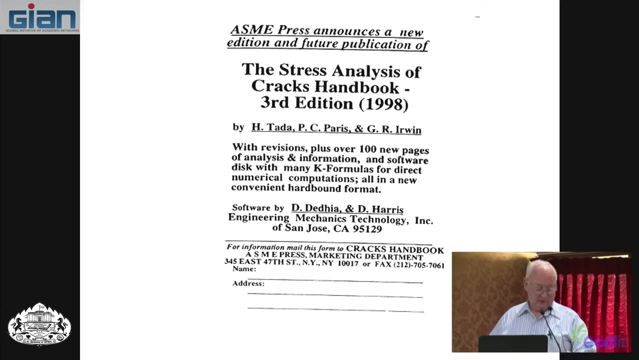 It doesn't make any sense. And I tell them: Use it long enough, You will get used to it. You will never ask again. What is the square root of an inch? It just is Here. is that analysis, The handbook terms? 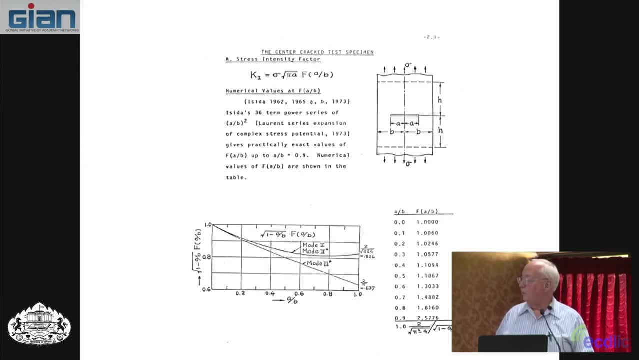 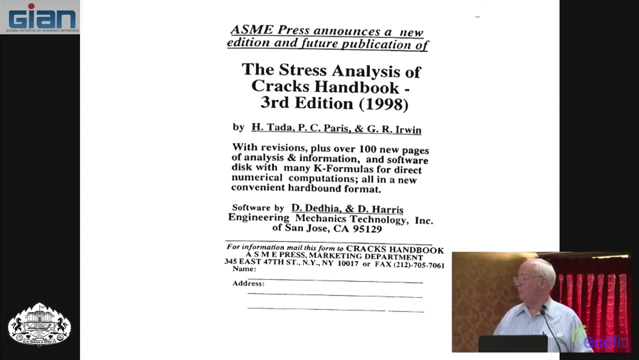 And in this Things I show you One of the Important geometries Is the center crack Specimen. It is like the Griffith geometry. Now, This was done by Paris Irwin And somebody named Tata. Tata was a Japanese student. 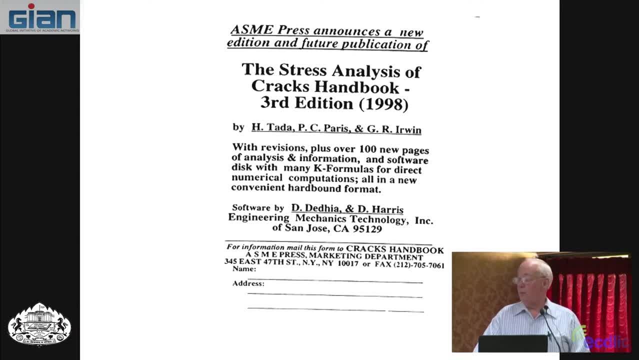 When I was at Lehigh He came to work with Paul Paris And when I first met him He could hardly speak any English. And then I met him again 30 years later And he could hardly speak any English, So he spent all his time. 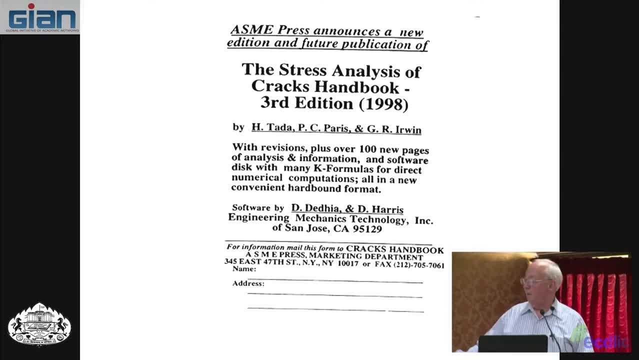 In the US, Stuck in an office Developing these solutions for Paul Paris And never learning to speak much English, But it didn't matter. Anyway, He developed most of these solutions. Paul Paris and George Irwin Had their name on this. 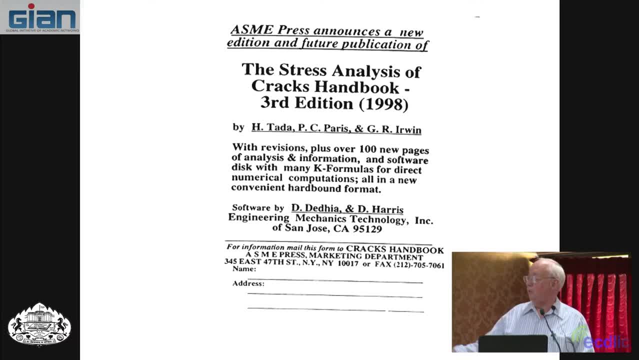 And this is one of the handbooks. There are others In this handbook, And the reason I always use this one: It is the only one I have, So it makes it a lot easier to use it If you have it. So here is one of the geometries. 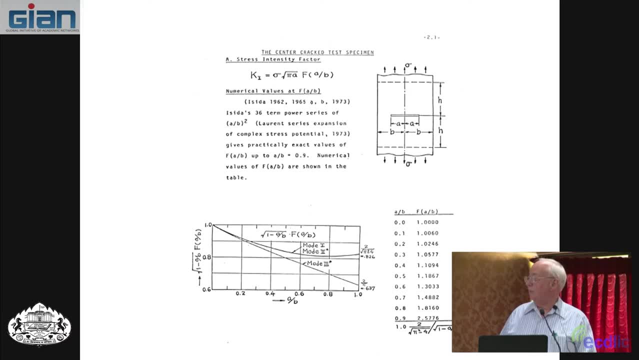 And the center crack Has 2A crack length, 2B for width. Now we normally use Capital W for width, But Tata for some reason Used 2B And you can't explain to them. Don't use 2B. 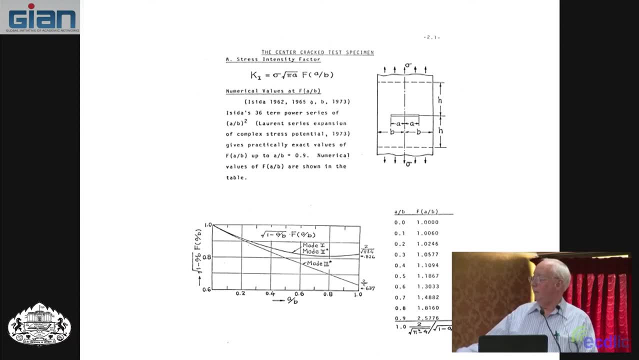 Because he hardly speaks any English, And so You just have to get used to that. The difference In that then? This is the capital F approach: Sigma Square root of Pi A And capital F function. The capital F function. 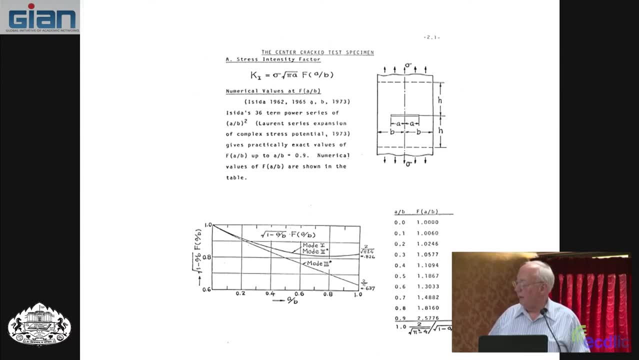 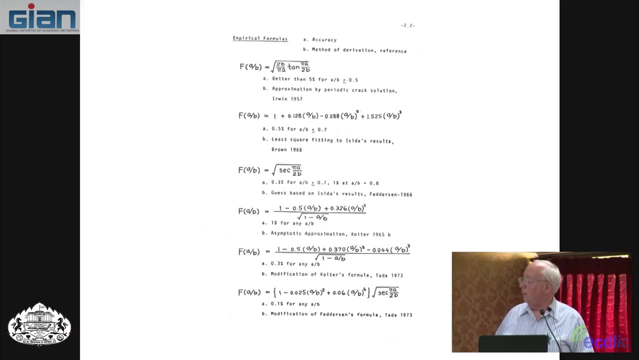 Is given graphically Or in a table, And the graphical solution Is not the capital F itself. I am going to hand out Some of these solutions, But I will go over them a little bit. This one Has a lot of work on it. 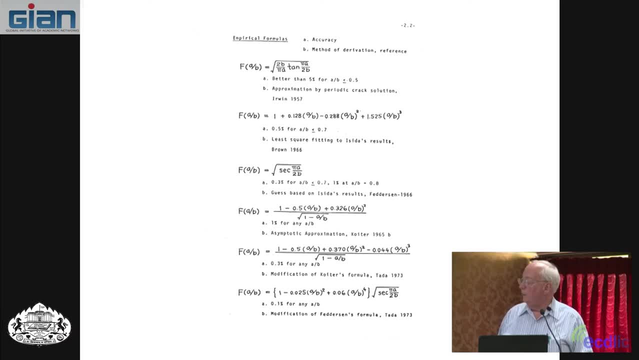 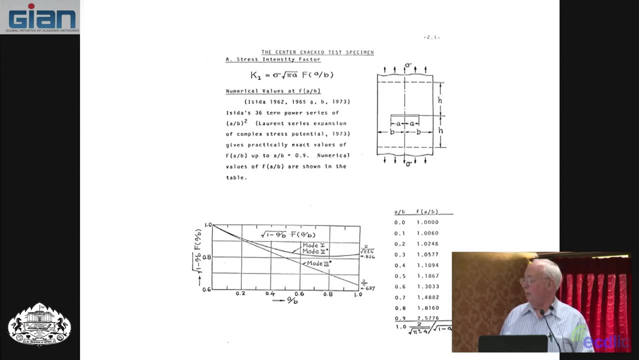 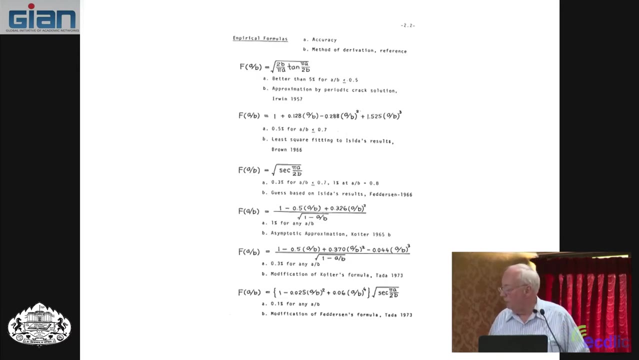 People develop Formulas For different Capital S for the same thing, And did a lot of work on this, And So there were a lot of choices For solutions. Now, the one that is used a lot Is this one: 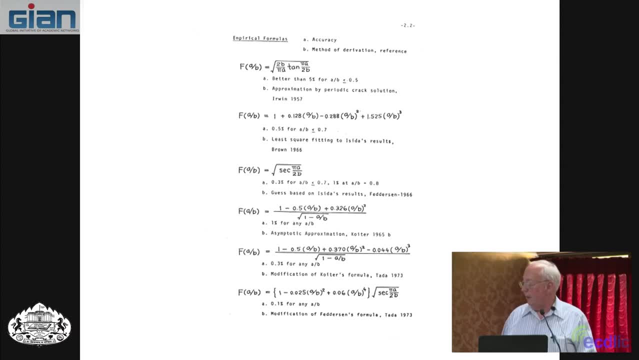 The quantification Of Feddersen formula. Now, Feddersen Is A person Who was involved with Fracture Mechanics Back in the 1970s. He came to about every meeting And one time He came to a meeting. 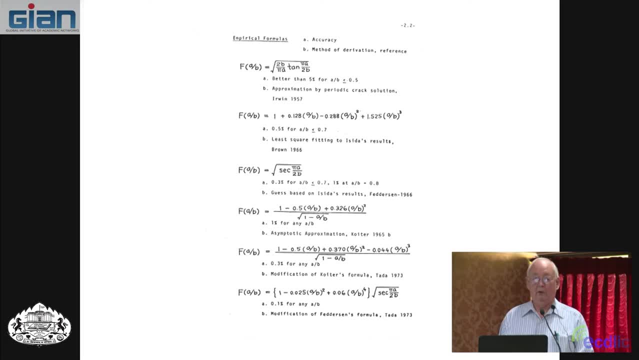 With his hair dyed all funny color And he said: guess what I did? I just bought a casino in Las Vegas And I am going to give up Fracture Mechanics And go into casino business. And I never saw him again. 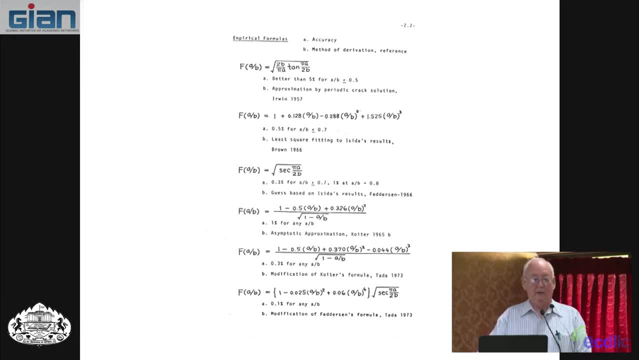 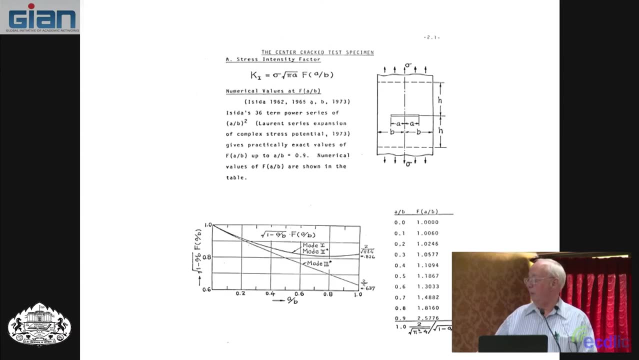 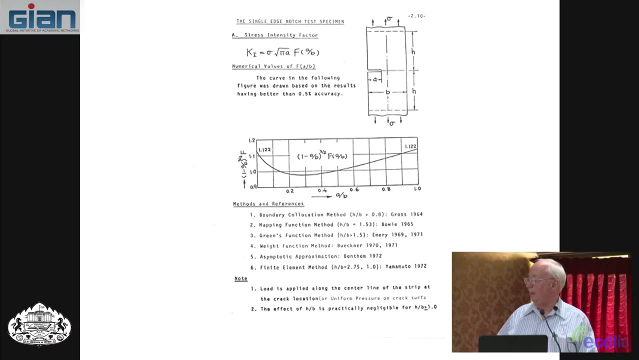 So I took from that That casino in Las Vegas Pays better than Fracture Mechanics. But nevertheless, This is his legacy. His formula is the main one used here For this, Some others In the handbook, And there is hundreds of them. 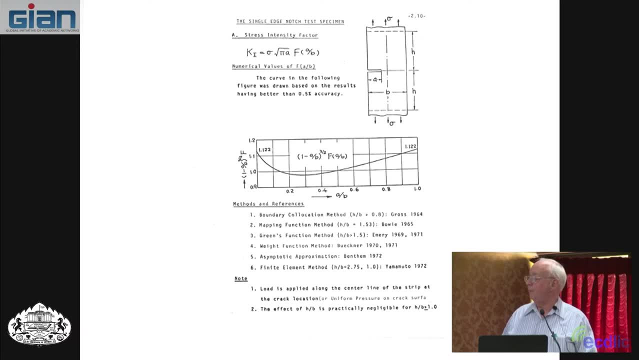 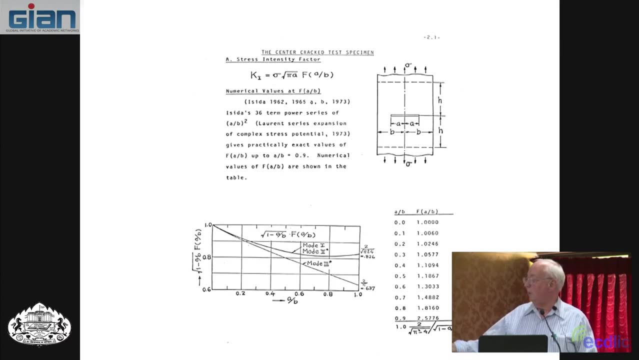 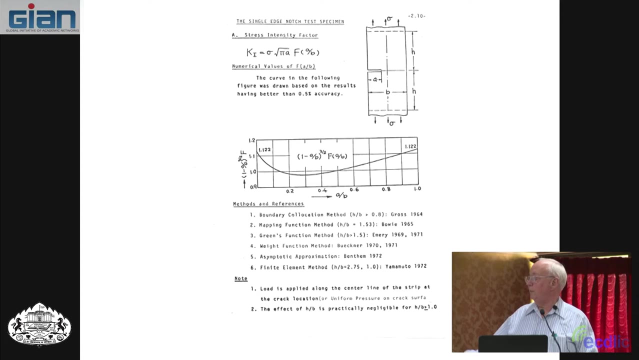 Here is an important one: Single edge crack. Single edge crack Is essentially The central crack Where you take a line down the middle And cut it in half, And cutting it in half Then relaxes The boundary here a little bit. 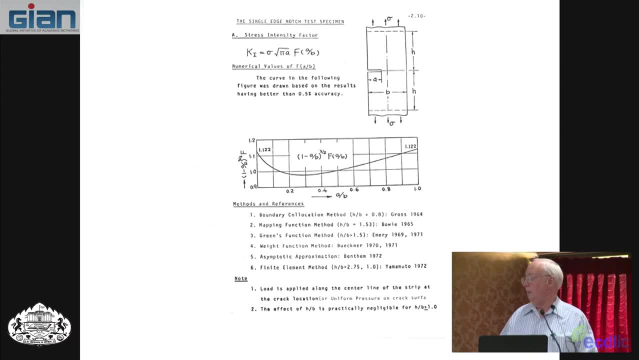 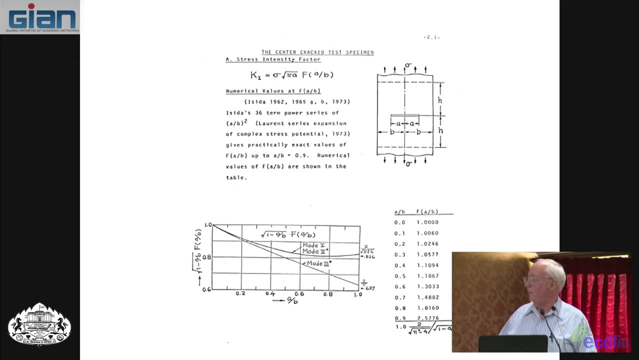 So it changes the solution Considerably. Namely, Point out this: That when you Have a central crack And you get a very small crack Compared to the width, We say that A over B, It tends towards zero. 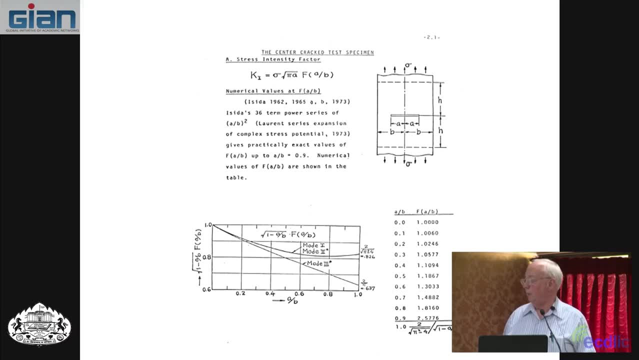 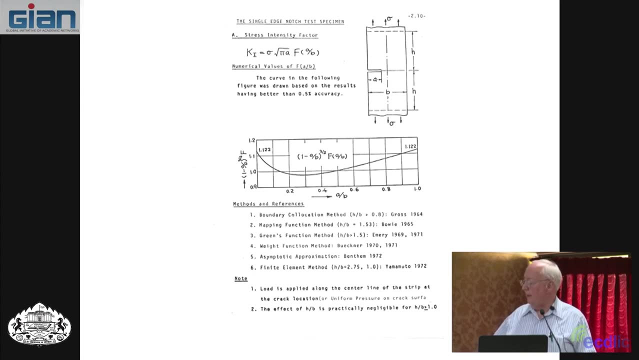 The F function Tends towards 1.0.. In an edge crack, When you have a very short crack And this tends towards zero, In the limit, Capital F Tends towards 1.122.. So Cutting it down the middle. 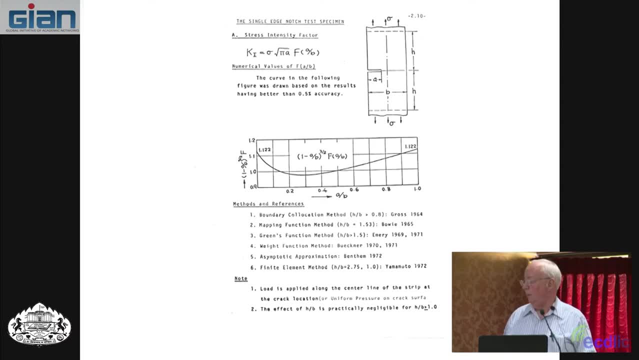 Relaxes that line, Causes the K To go up a little bit. And The other thing here: Point out that, Whereas this has a table, This does not have a table, But rather it has Just a graph And that graph. 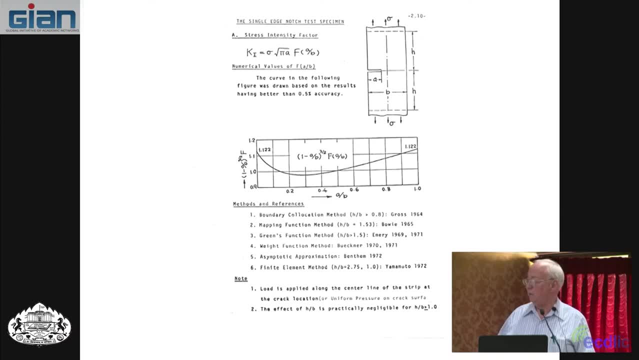 Is a little bit hard For some students to use Because it's normalized. The reason it's normalized Is to make this curve flatter, So we go off to Very high numbers quickly. But with that it's normalized And it's much flatter. 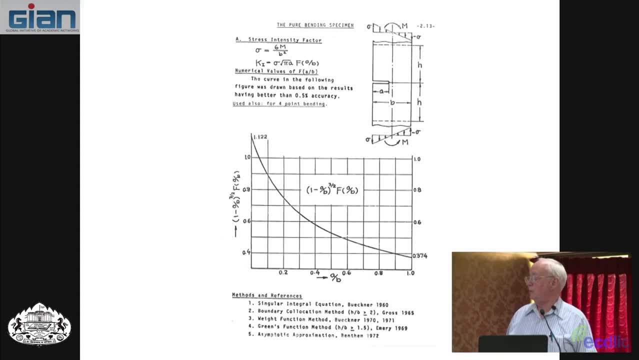 Some of the others That we won't use much. But I'll just show you A single edge crack With bending rather than tension And in the limit It tends to 1.122.. All edge cracks In the limit of a small crack. 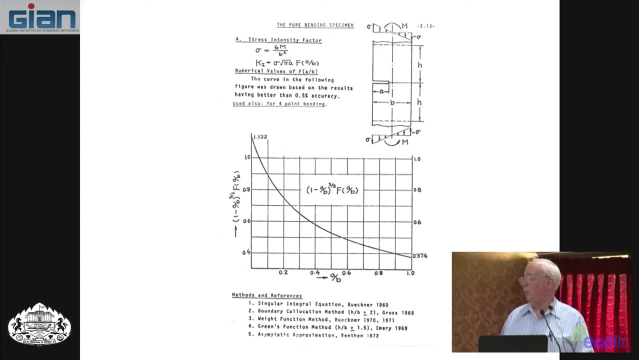 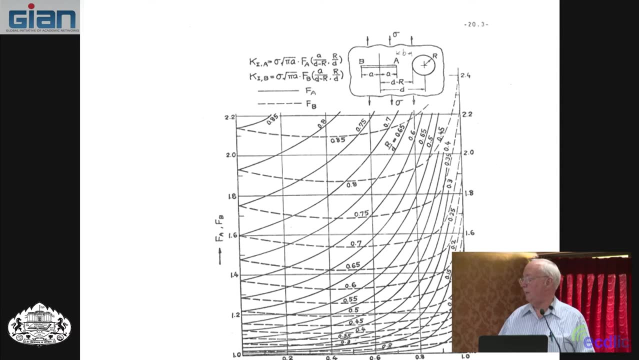 Compared to the width Tends to 1.122.. Some of the solutions From the handbook That we won't use. Just to show you How complicated they look, Here's an example: A crack approaching a hole On one side. 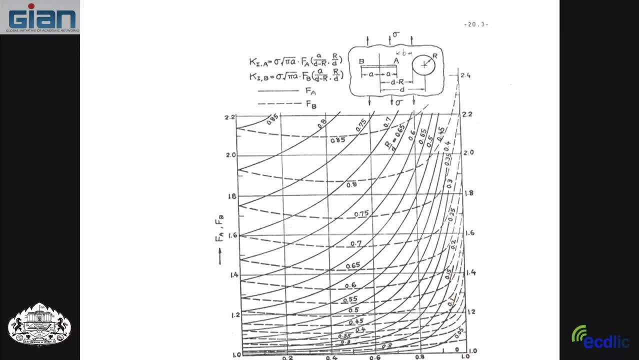 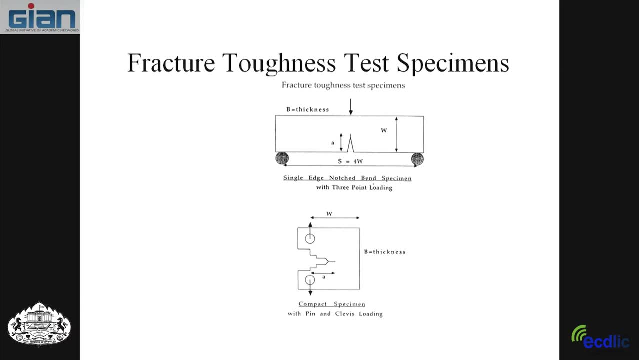 And an empty plate on the other. So you have the solution For the A side and the B side Being different And all these criss crosses of curves. Okay, That's the break time And we'll come back And talk about the fracture toughness. 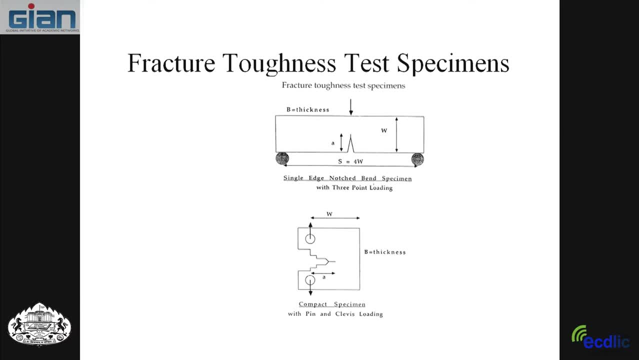 And maybe hand out some stuff. So let's take that break, The classical two letter break, And come back at. Try to come back at 3.30. So we can get back on time. What I would like Is for everybody to get. 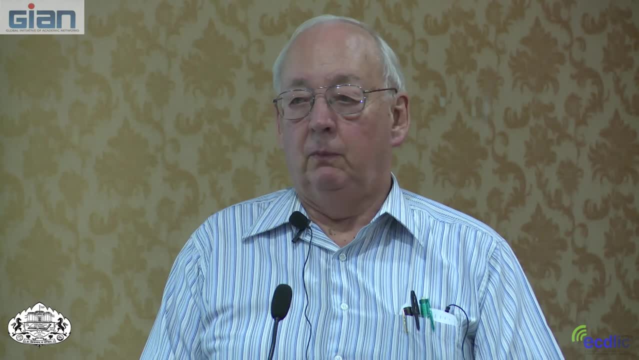 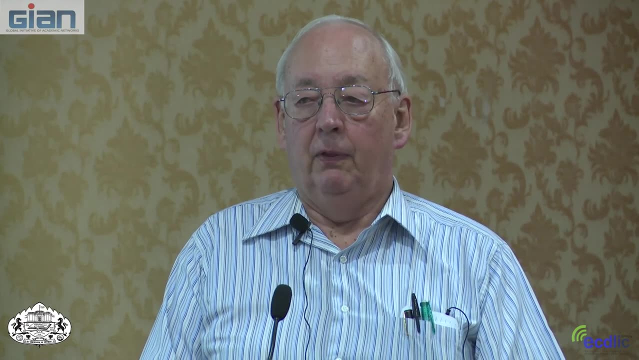 A copy of my slides. So we've decided that they will be Put in PDF file And then, if you can upload them, You will have a chance To upload all those slides. They'll be important in the future We're going to have 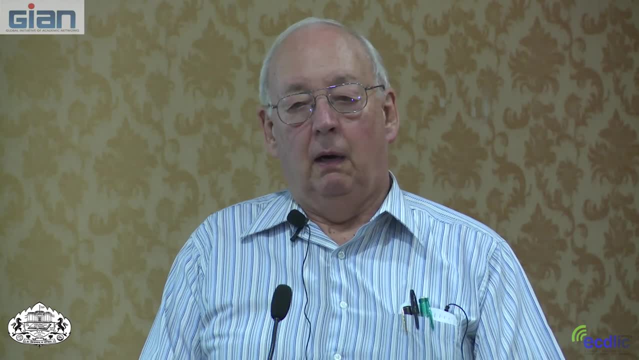 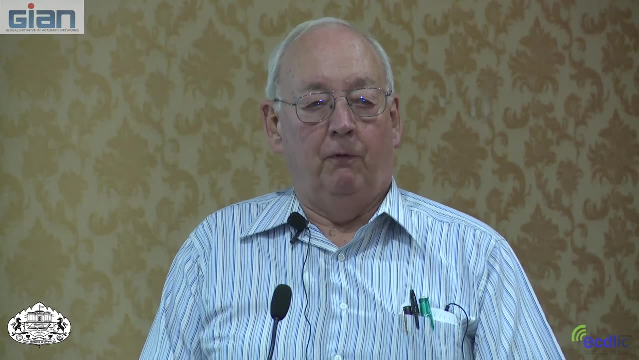 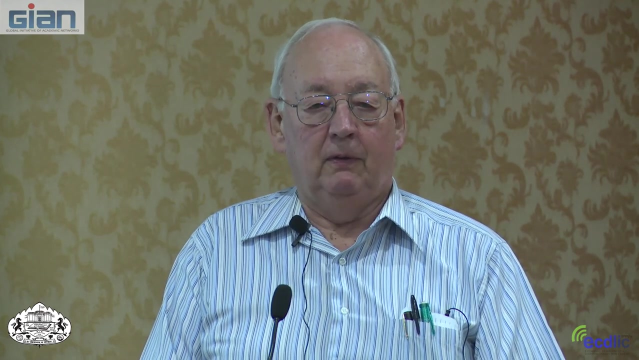 A little quiz at the end And it's open book, So you should use Everything there. As an engineer, We don't work from memory. Engineers usually work from books And charts and all kinds of stuff, So I never given a little quiz. 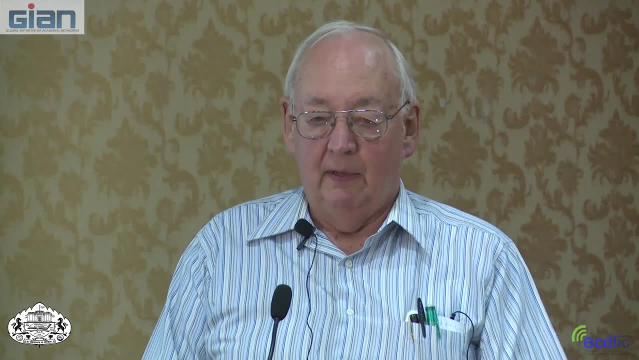 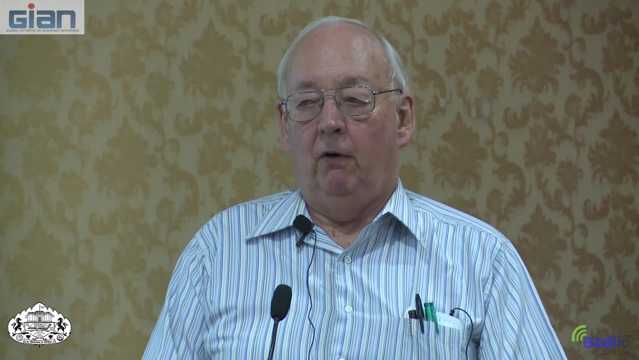 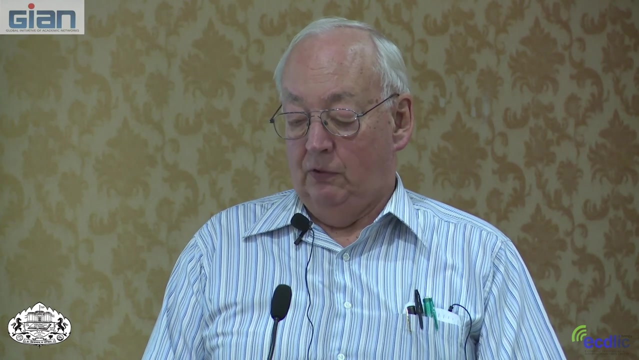 To have people work from memory. This goes against engineering. Now Showed you some case solutions For typical Structural element types And they're in that handbook. Now, besides the handbook, Are the case solutions For various Geometries that are: 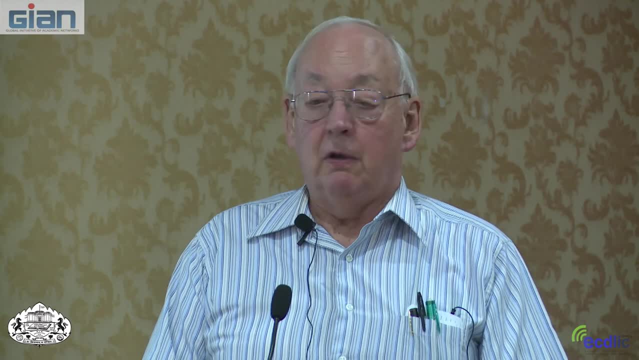 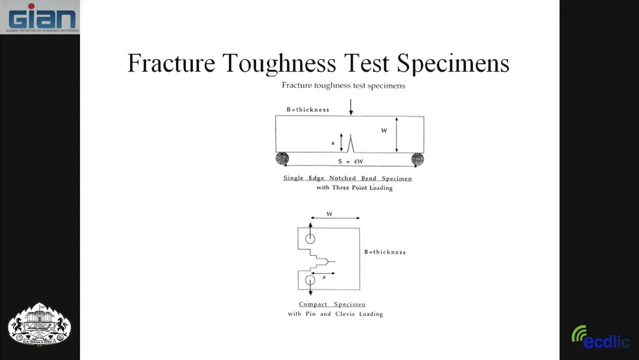 People use in testing. I have fracture toughness testing, But almost all the kinds of testing I'll talk about Use specimens that look like this: And this is a single edge Bend specimen. And this is a compact specimen, The single edge bend. 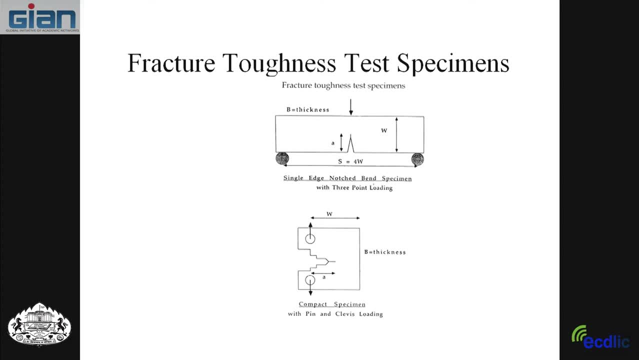 Is in three point bending And has the span. This S distance To the planar width, W of Four to one. For the most part I use ASTM nomenclatures, Which uses W for width, And skip that, But not always. 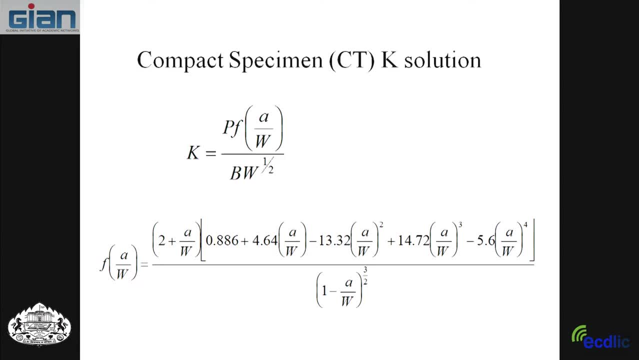 Anyway, The solutions For K Have this F function, Which is a real bad polynomial. Now, if you're going to use Calculate that polynomial All the time, It's a pain in the neck for number one. Number two, I never go through it. 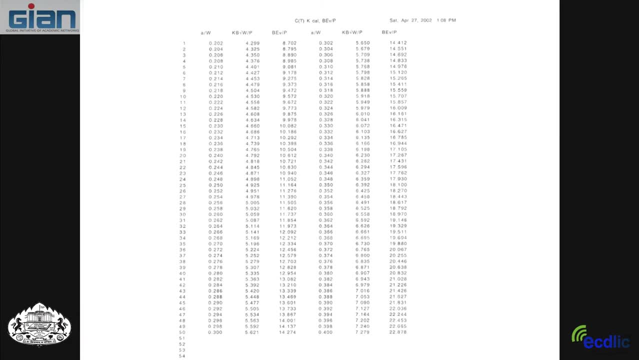 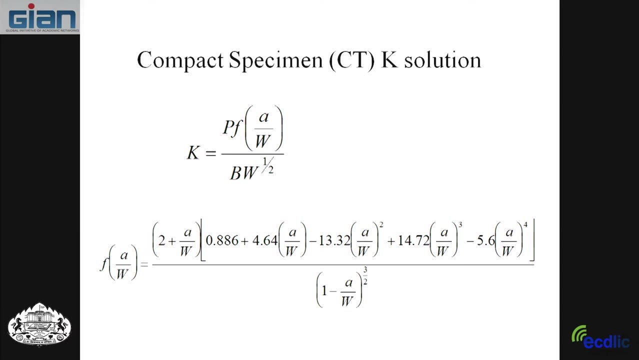 And get the right answer, Because I make a mistake Somewhere along the line. Print it out In a table. Now, if you rearrange this, Take B square root of W Times K And then divide that by P, So B K. 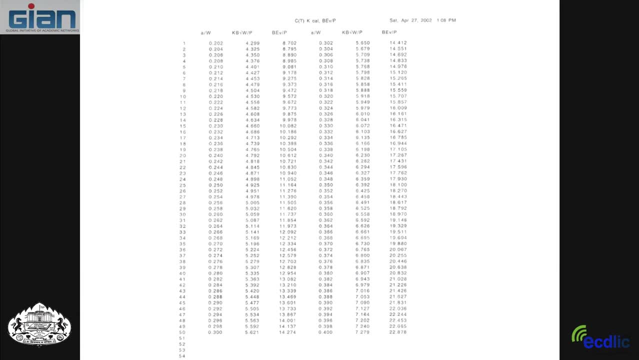 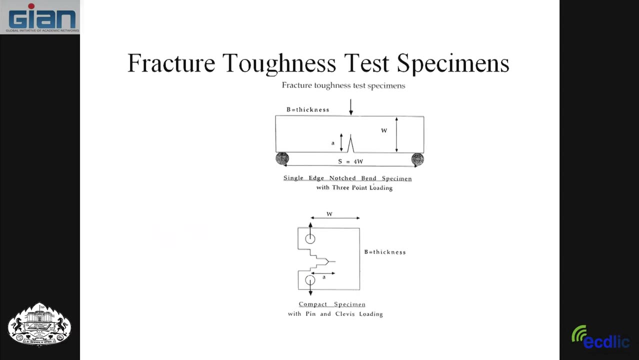 Square root of W divided by P Is a little F function. So it's this column. It's a little F function. Start it with A over W. Which A over W is In this specimen? Crack length From the center of the pin holes. 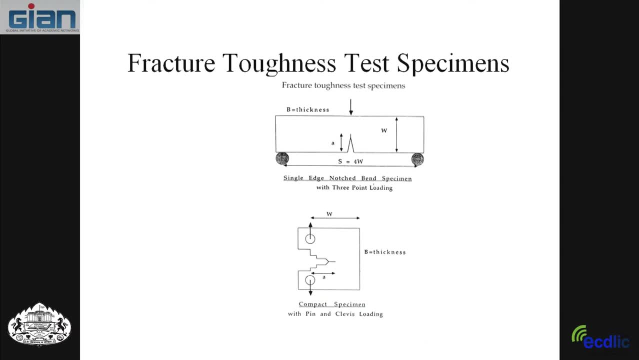 To the tip of the crack. Here it's from the edge of the specimen To the tip of the crack, And then W is the width- here W Isn't Good- or From the center of the pin holes. 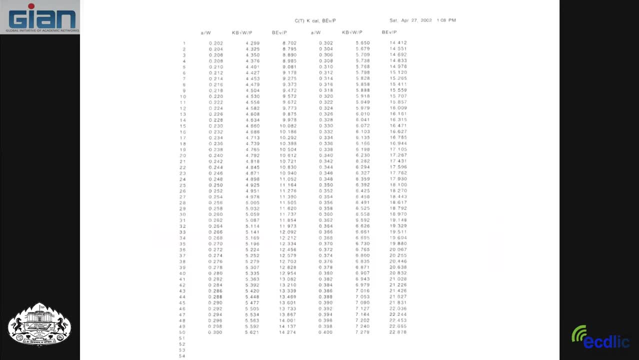 Is the W. So rather than using that polynomial all the time, That's convenient. if you have a Computer controlled Test system, You just put it into the test system. But if you're doing things by hand, Like we'll be doing, 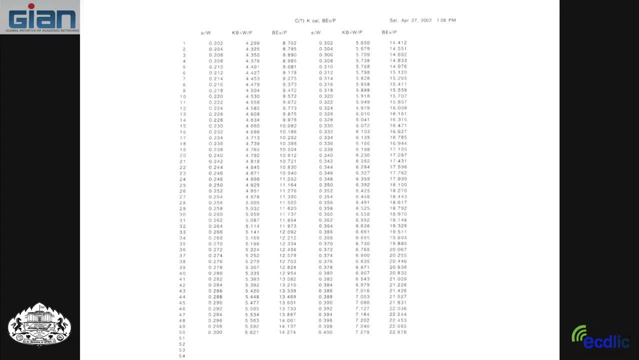 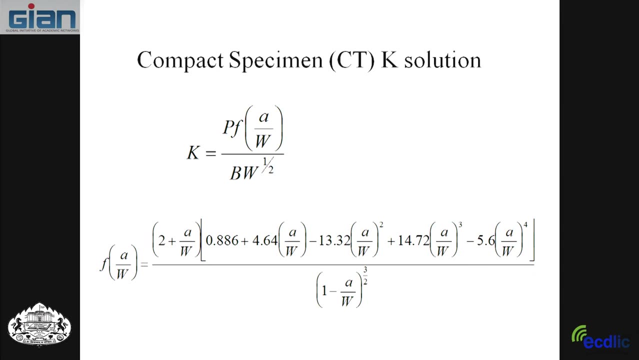 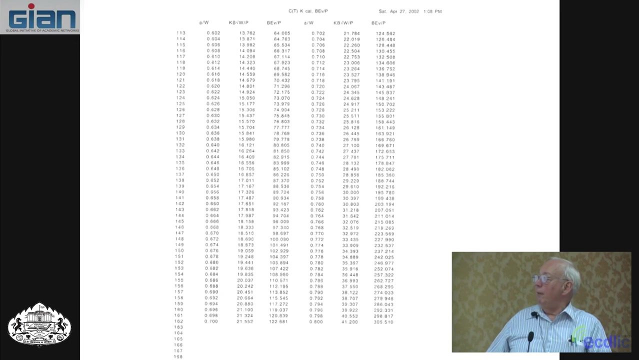 It's much more convenient to have that table. So I've handed out this whole table. This is for K calibration for the C comma T In In fracture mechanics. That's called the compact specimen, So I'll show. you Have that whole table. 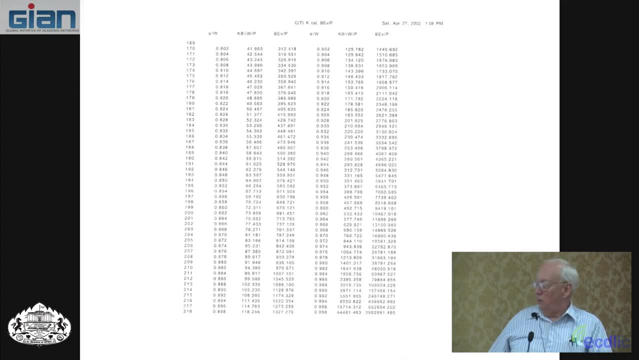 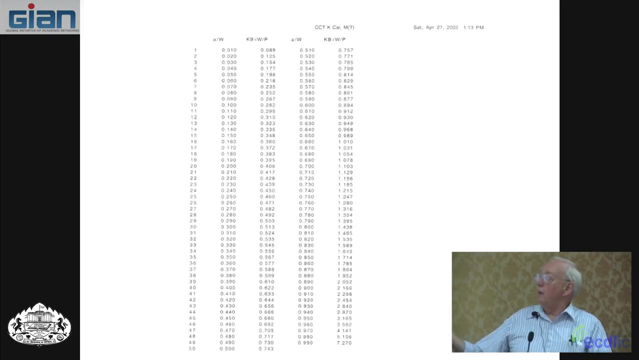 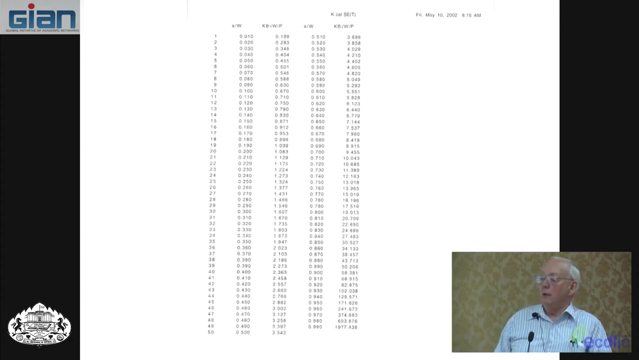 Goes from A over W All the way to. And then I have some other tables. This is for the center crack. You can use again that, That form, And then also For single edge tension, You can use that, Or you can use the capital F form. 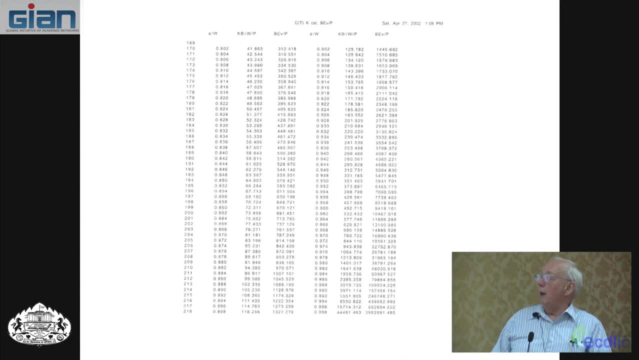 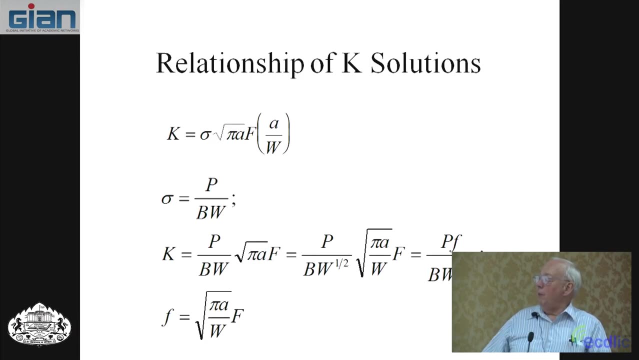 For both of those, For the compact specimen And the little f form. It doesn't make any sense Now. the Capital F form And the little f form Are related. I've just done the schematic So you can see. 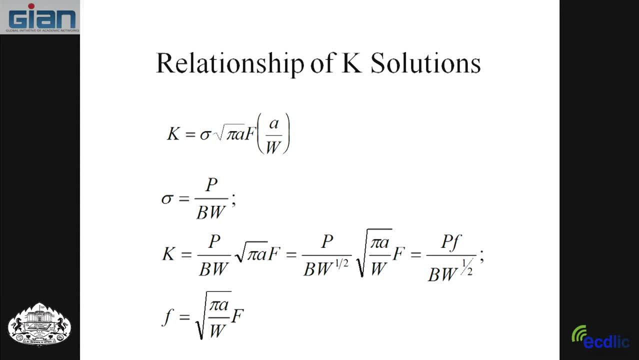 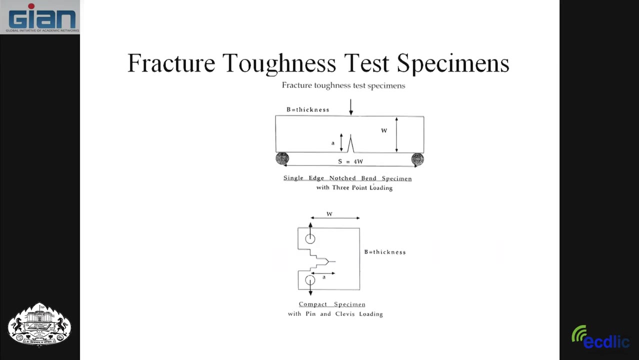 If you take the stress Is load divided by the area, B is thickness, W is width. When we do K calculations, You're always calculating stress Before the crack is in place. So you're taking a specimen Like this, Like this: 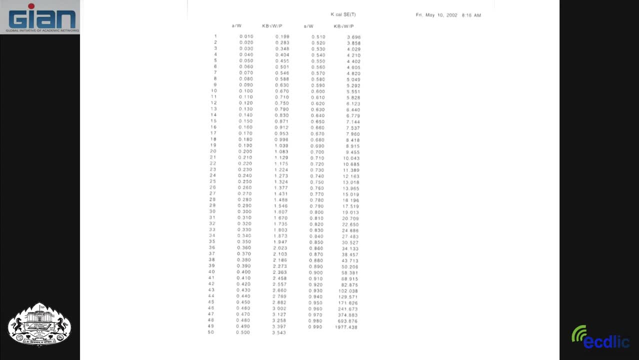 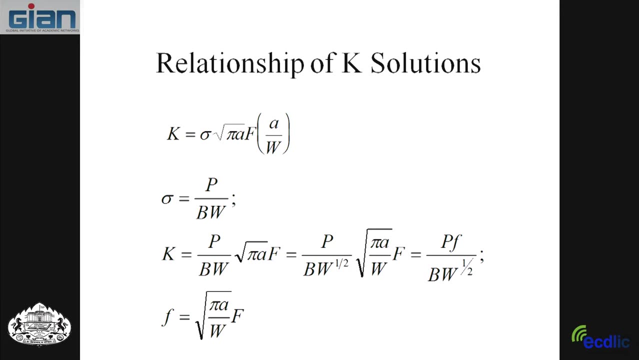 And assuming there's no crack in place- And doing the stress calculation For that, And then put that Here: for stress, Take the W and divide it Into two square root parts, And then this whole thing- here Is the little f. 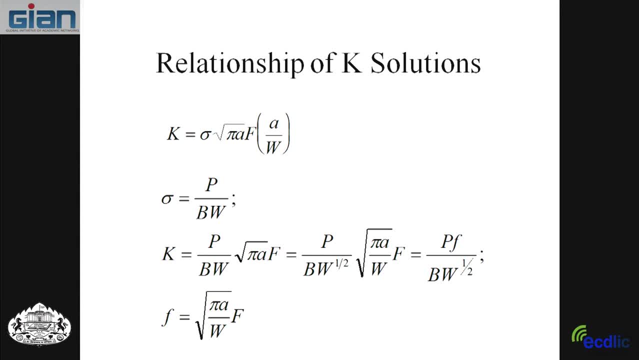 So the little f is that whole thing. So they're essentially the same thing. However, It's easier to use the capital F form And if you start with load P- here is the load- It's easier to use the little f form. 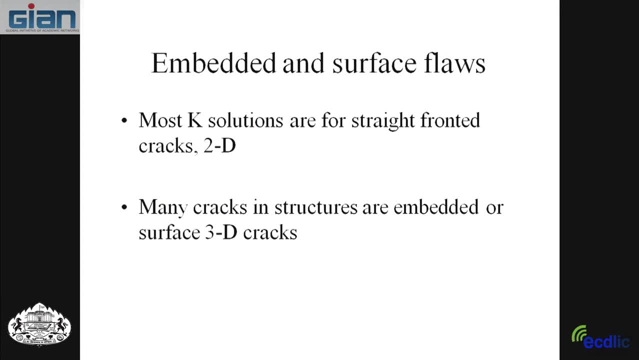 Those solutions I showed you Are two dimensional solutions And for most Two dimensional bodies, Where the crack goes all the way through, You assume that the crack front Is straight And then the K is the same All the way along that crack front. 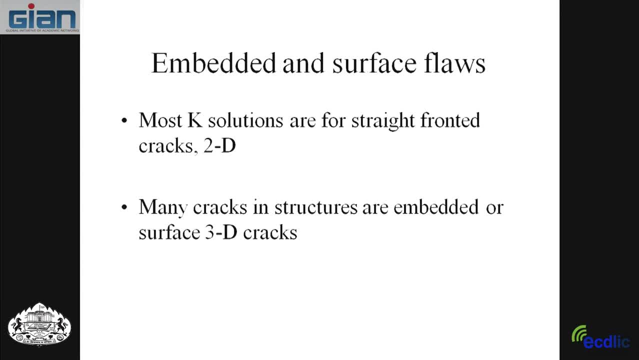 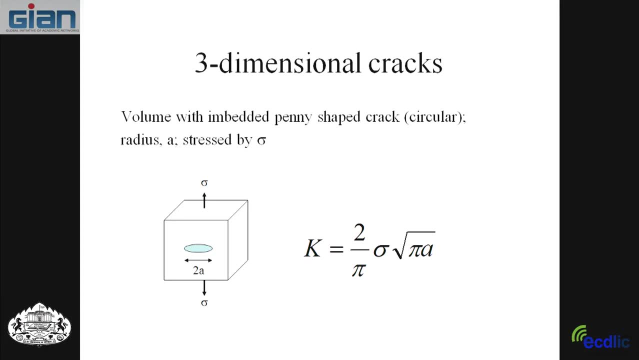 Any of the structural Cracks, though, Are three dimensional Or are not straight through, So I'll show you some of those. Here's one a little hard to imagine. It's called penny shaped crack. It's just a round circle crack. 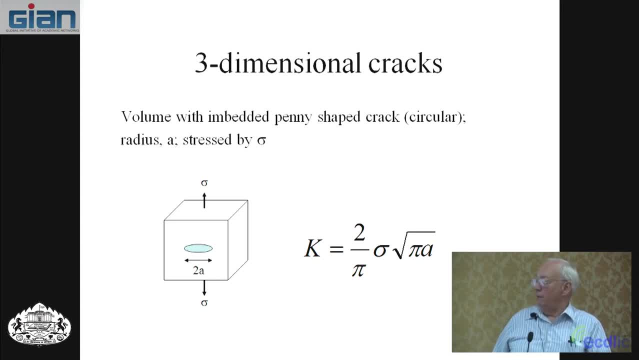 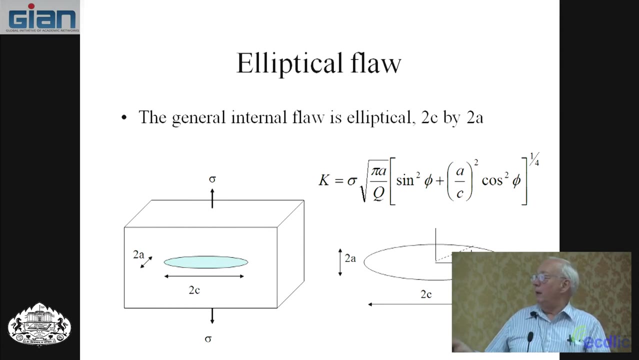 Embedded in this material And here's the K solution for that. It has Always has that form, stress And square root of crack length, But sometimes it has different. Now here is the Most common 3D crack, Called the elliptical flaw. 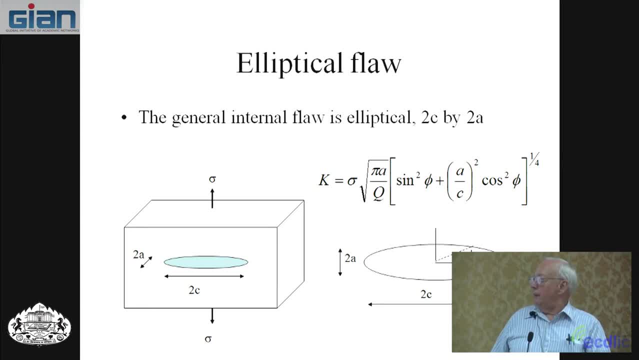 The elliptical flaw Has A major axis Of 2C And a minor axis of 2A, So this ellipse is embedded In that specimen. Again, you can see this is mode 1.. It's pulled load stress. 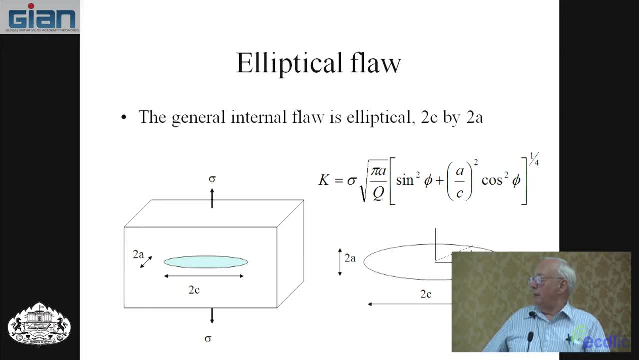 Perpendicular to the crack. So it has the form Sigma square root of pi A, And there's a Q factor here And there's also A little phi factor. The phi is the, The angle from the horizontal, So as phi is zero. 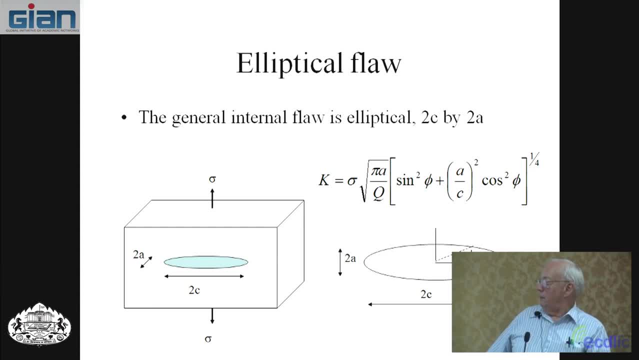 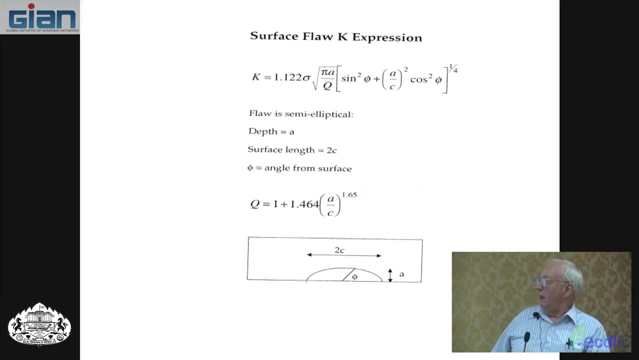 Would put you right here, And as you get to 90 degrees, You would be right there, So the K itself Changes as you go along The crack front In an elliptical flaw. Most often, though, This elliptical flaw 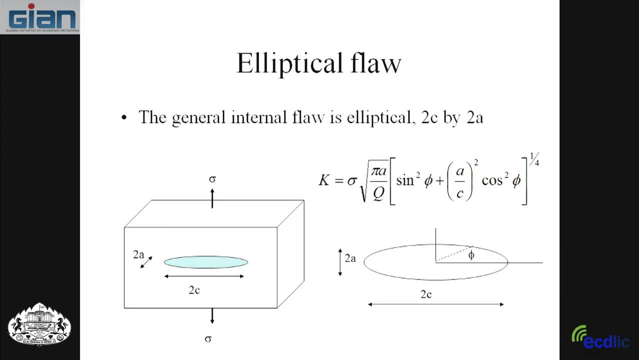 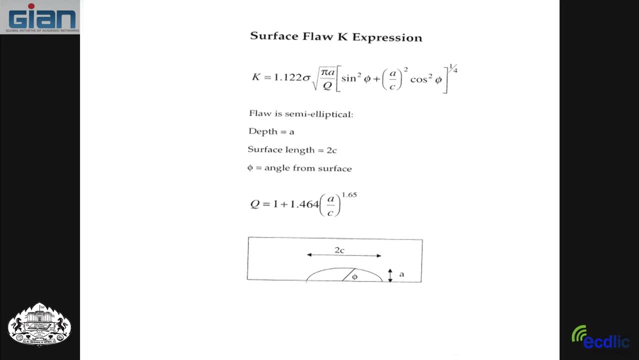 Is cut in half And you get the semi elliptical flaw. Now this is looking From top down here After you cut the thing in half: Semi elliptical flaw, So that the major axis is still 2C And this is a semi minor axis. 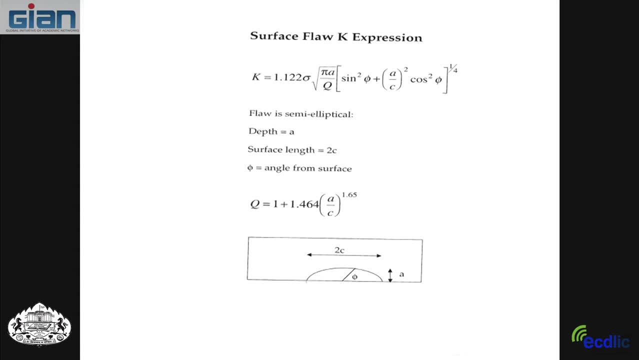 To the ellipse And you have then This K solution. You pick up the 1.122 factor Out front And the depth, then A, The surface length, 2C. Phi again is the angle from the horizontal, And so you need. 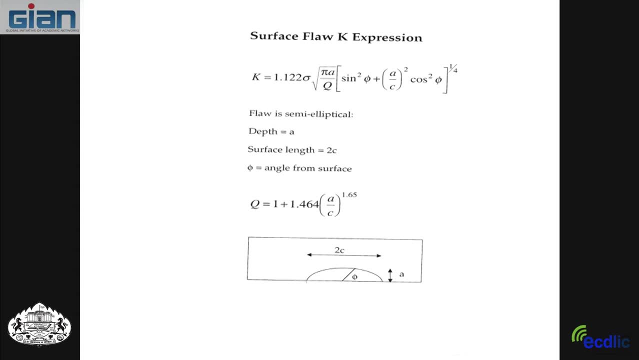 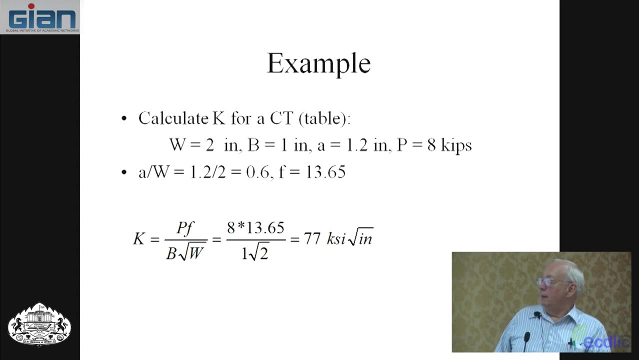 A Q factor And this is an approximate Q factor. Okay, Here is some Um K calculation Examples. I don't have the table things Right handy, But say you want to calculate K Using that table, You need some geometry things. 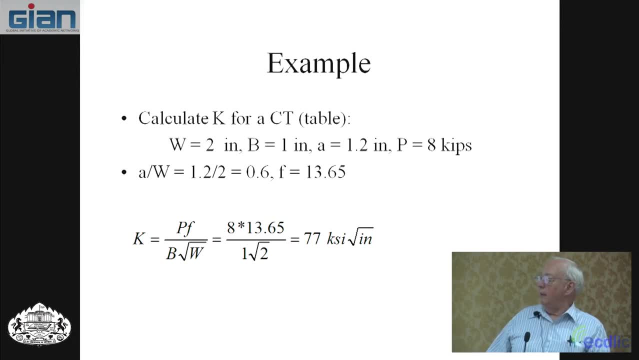 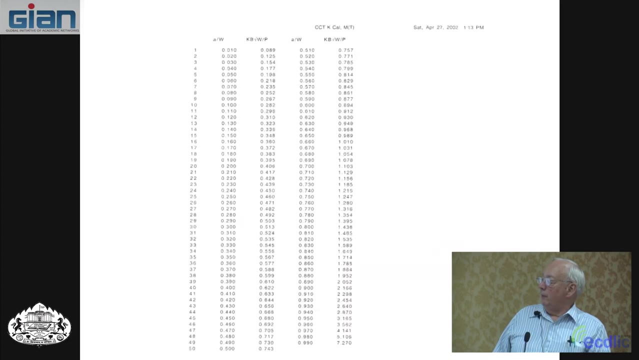 And these are Unfortunately in Engineering units. So the width is 2 inches, The B is 1 inch, A is 1.2 inches And load P is 8 kips. Um, Sorry, I have to go back to the picture. 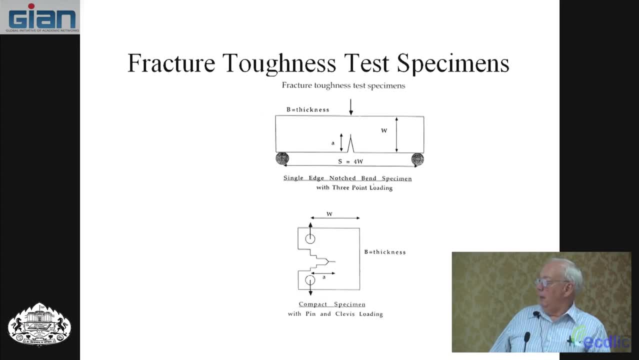 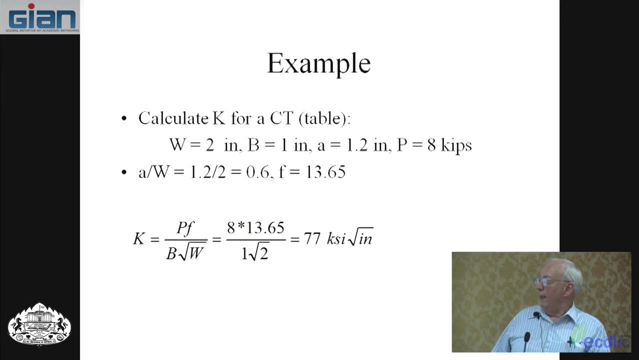 And B is Thickness 1 inch, W is 2 inches, The A is 1.2 inches, Is here, So back to this. First thing you have to do, Then, is take The crack length to width ratio. 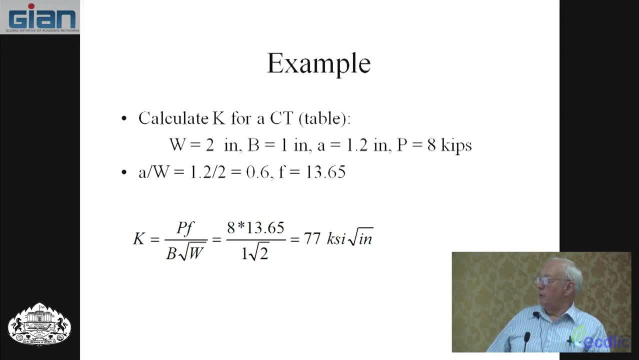 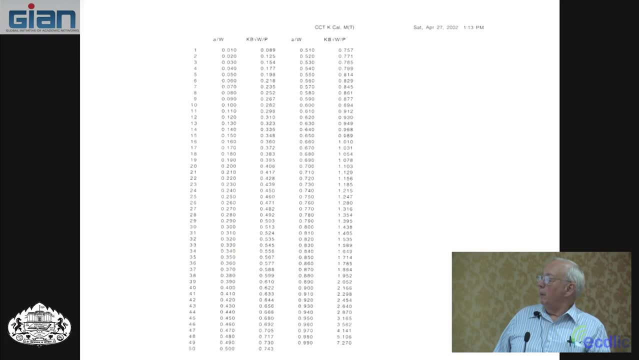 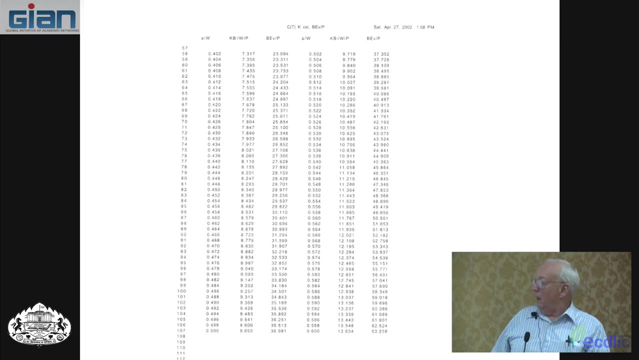 A over W, 1.2 over 2. Is 0.6.. You can go then to the table, Look up 0.6.. 0.6 is Right Here, And this is the F for that. 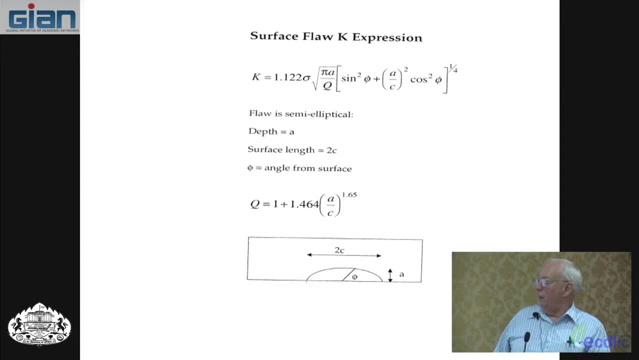 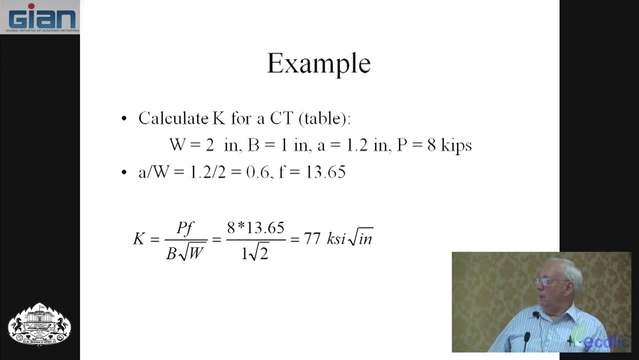 13.65 rounded off. So using 13.65 for For the F. So you put those all together, Load 8.. Little f, 13.65.. Thickness B is 1.. W is square root of 2.. 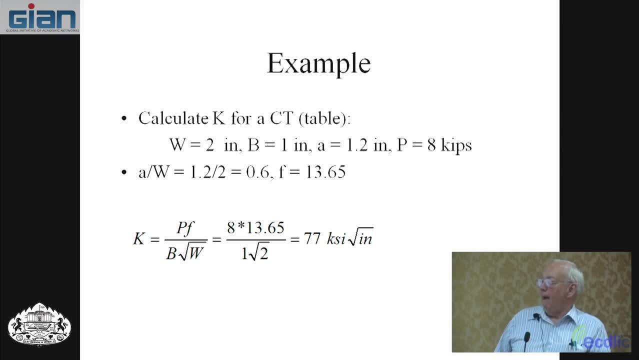 Get 77. You will. You will have to do A lot of K calculations, So you should try to get used to it As quickly as you can. Here is another example: The picture Of the center crack. I used 2B. 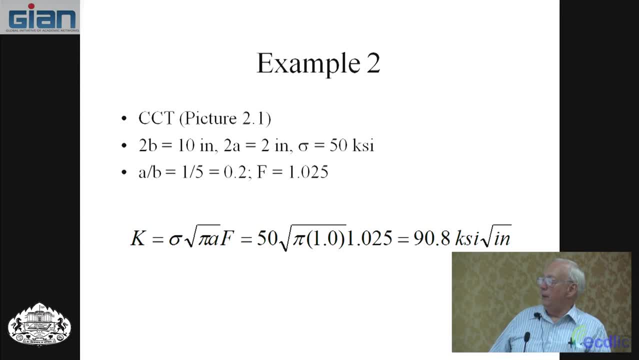 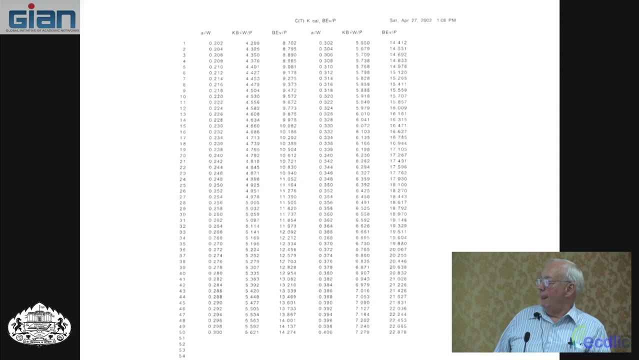 Because that is what Tata used. 2B is 10 inches, 2A is 2 inches, Stress is 50.. 1 over 5. Is 0.2. And then again 0.2.. Back to this. 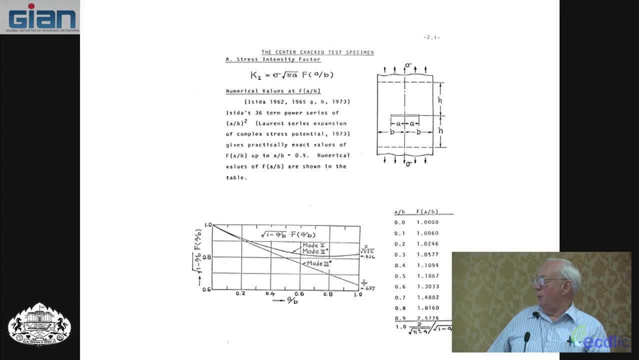 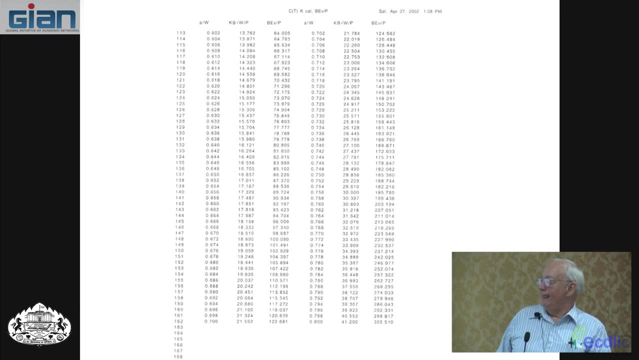 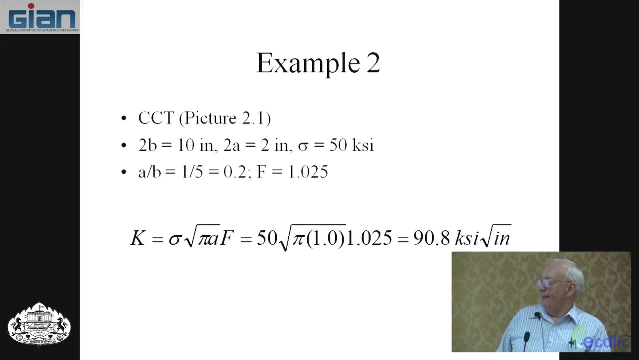 I can pick that off the table 1.2.. 1.0246.. 1.2046.. Round off to 1.205.. Stress 50.. Square root of pi, Square root of crack length, Is all under the radical. 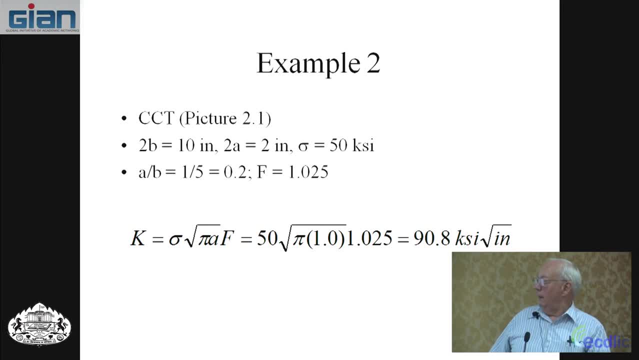 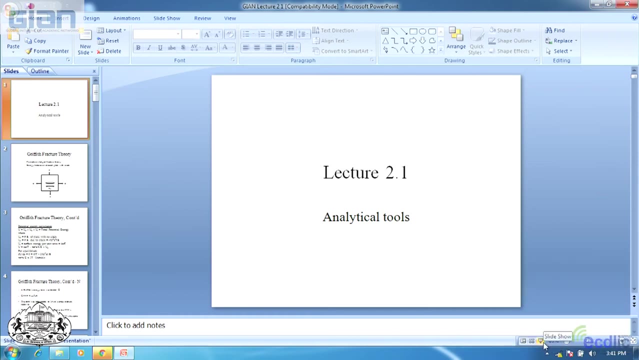 And then the capital F Is out front, You get a number 90.8.. So that is K calculation For a center crack Using the picture. Question Yeah, One That The This slide Our day. 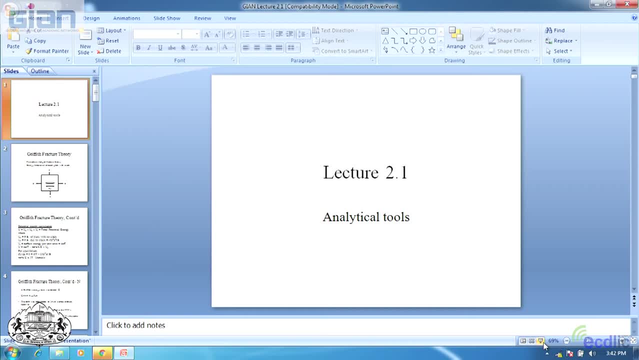 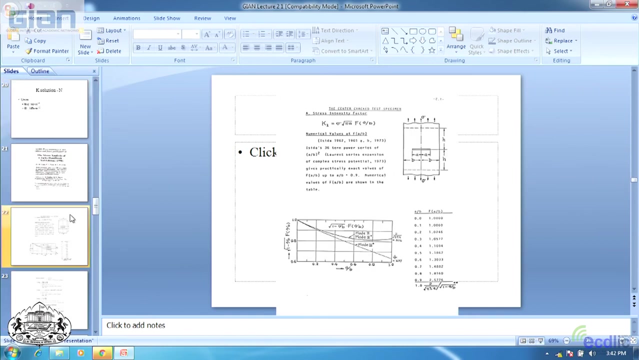 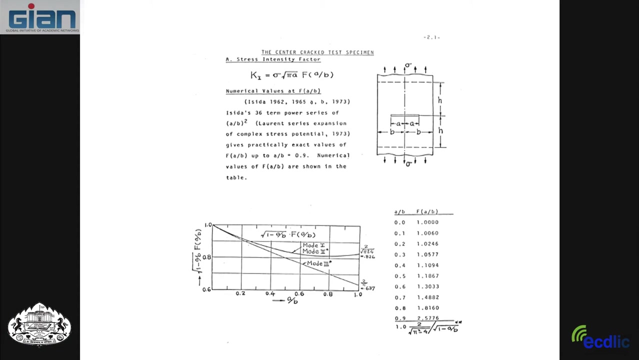 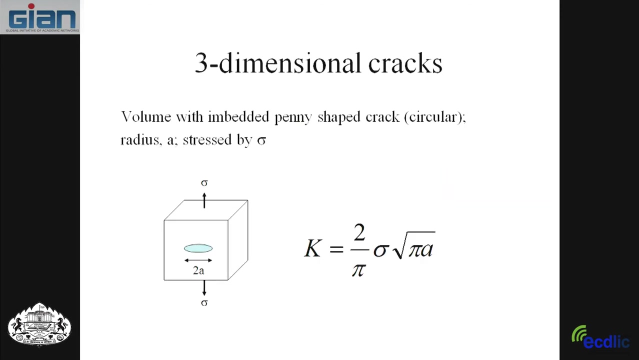 This, it's this one. Yeah, Oh, Penny Shaped, You want to see that picture. Okay, sorry, I didn't do any examples for him, But Yeah, you see The previous one. 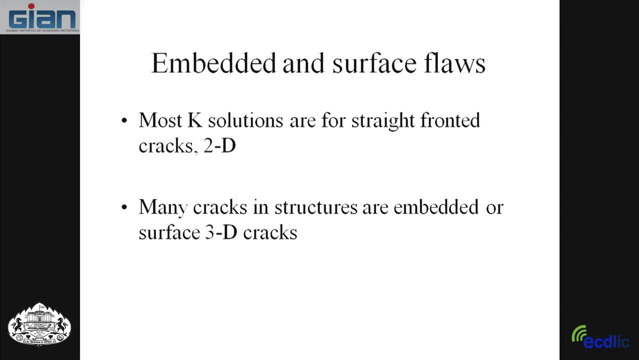 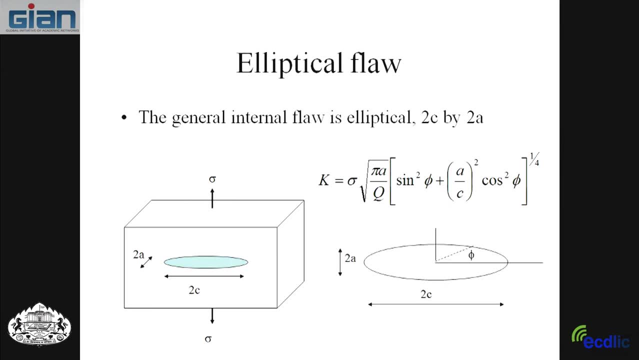 The previous one. Okay, That's elliptical flow, yeah, Yeah. Yeah, It's higher when it's 90 degrees, And this it's a round circle Where A and C are one. If this is one, then you get that identity. 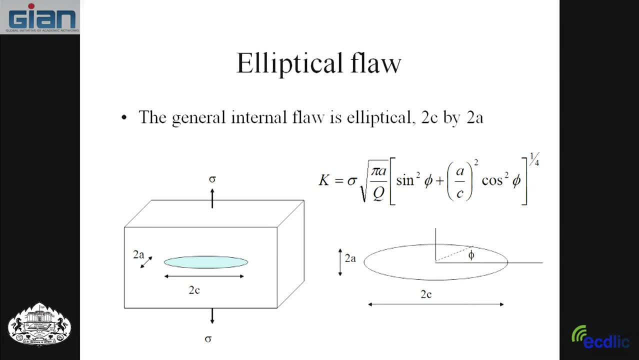 Sine squared plus cosine Sine squared equals one. So this thing goes away And you just have that. That goes to one too. Yeah, In elliptical crack, when you are closer to the center you get higher K's. 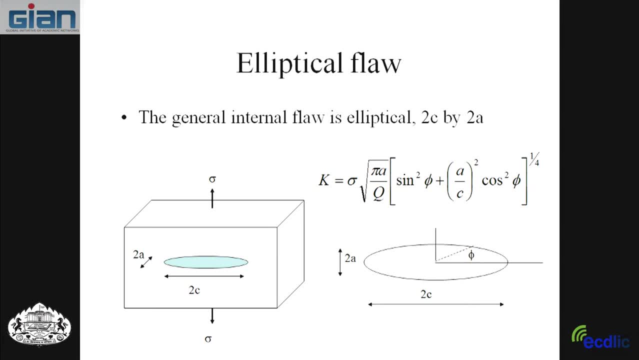 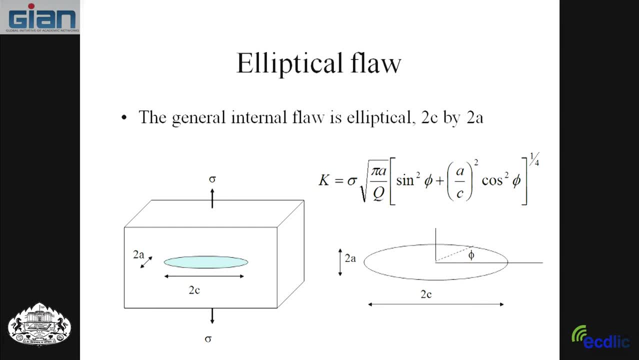 as you go from the distance out here and get closer and closer to the center, the K increases. It keeps going up and up. So a lot of times with an elliptical crack or a semi-elliptical crack, people just worry about that point right there. 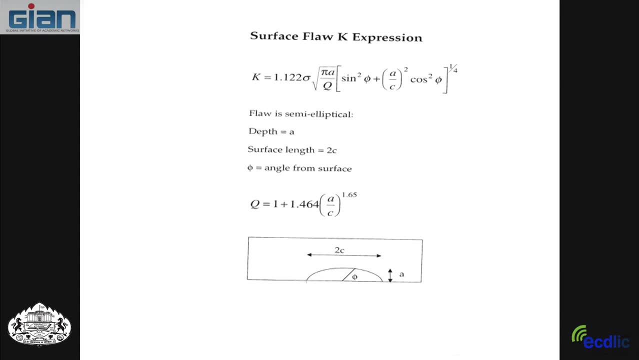 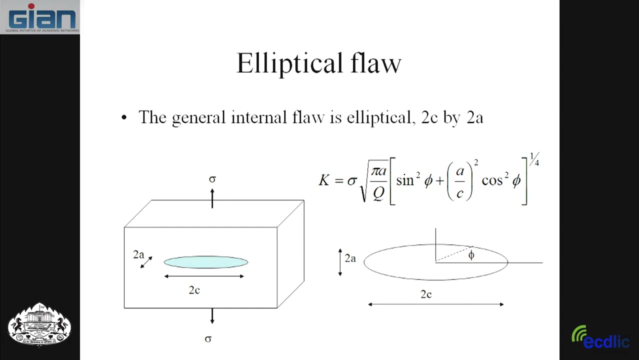 The K right there, Because it is the highest K. It could be the nose, the radius or the curvature. at that point It could be a relationship with the radius. It could be. yeah, I think, if you take this thing and pull on it. 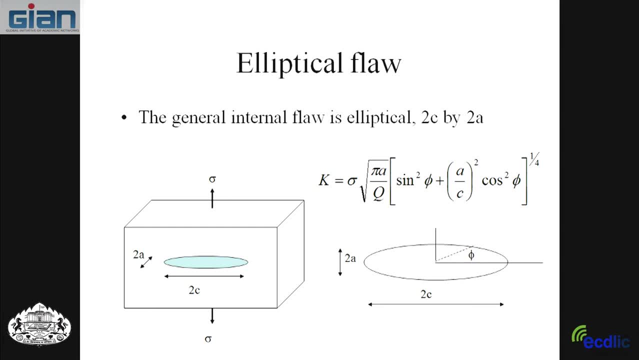 it's really not intuitive, Because the longer the crack, the higher the K. So you're saying, oh, that's the shorter distance, not the longer distance. K should be higher here, but it's not. Yeah, so it's counterintuitive. I'd say 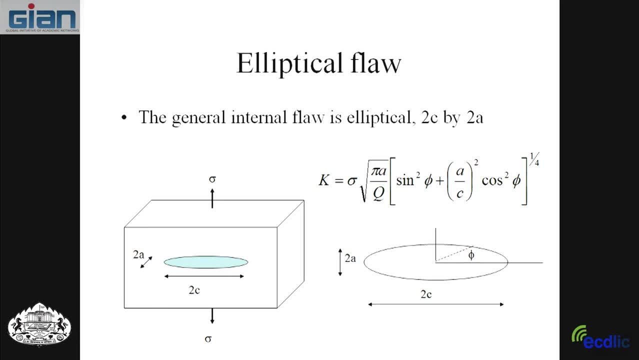 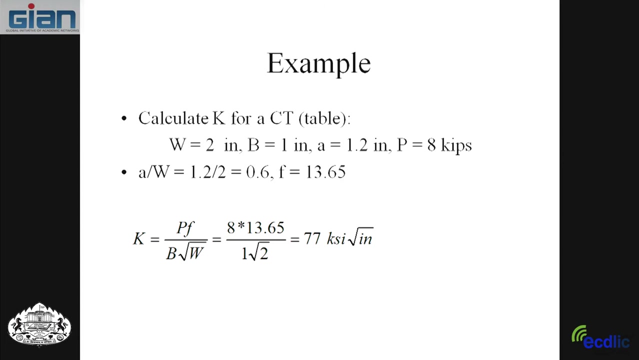 If you want to think intuitively, I don't know what else to say about it. That's the way it is. Other questions, Any other questions about these Now? So if you pull on it, the highest is right there at that short point. 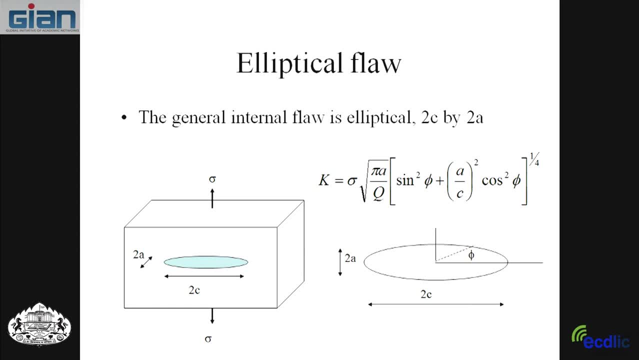 Yeah, right at the short point is: yeah, When you pull on it, Does that seem intuitively? so? Not necessarily. Yeah. Yeah, it seems like it's just more damage to the material. Maybe, Yeah, it would. Yeah, but it doesn't. 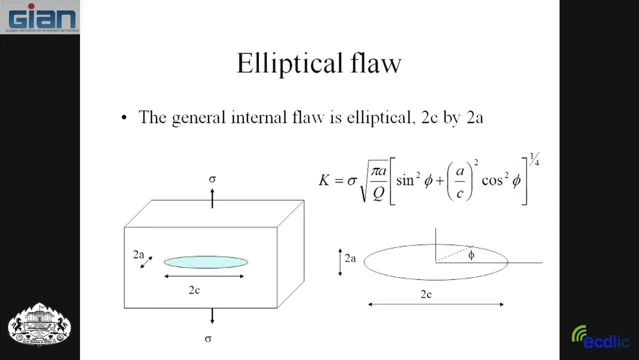 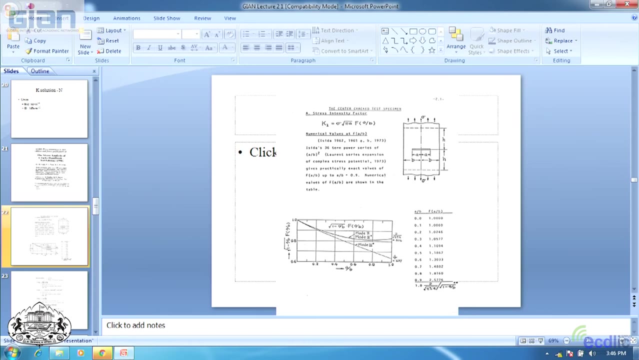 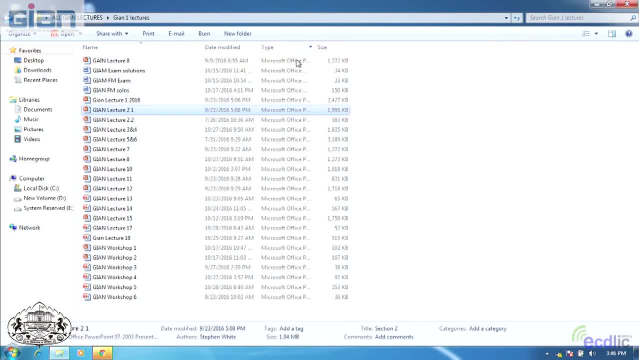 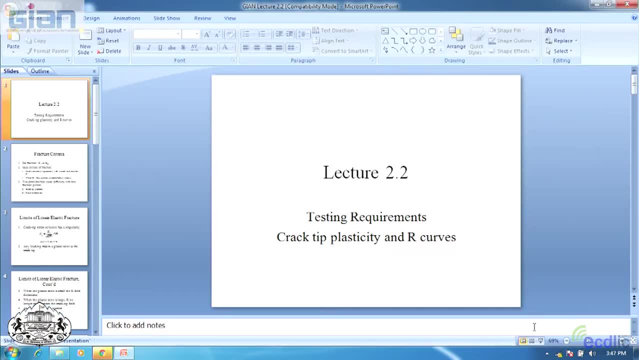 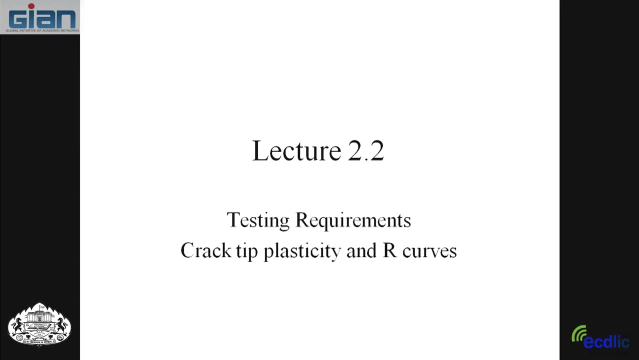 I'm not good on this computer. I have a short thing I want to show you you, and then I'll get you a chance to have your own fun of doing this. Before we talk about testing, I wanted to show you two problems that come up in our 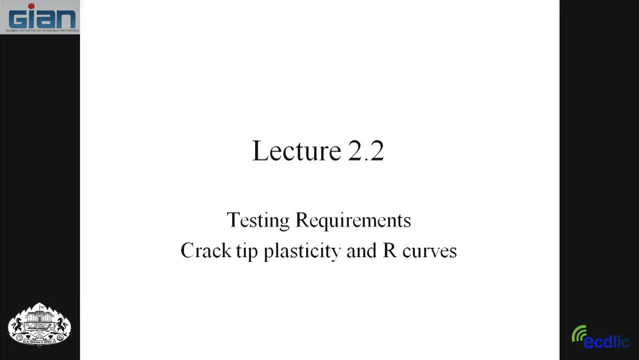 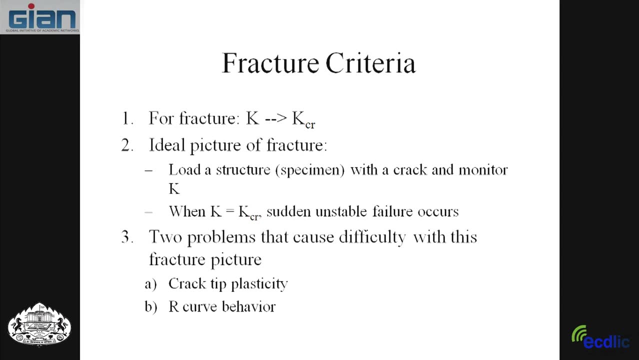 fracture mechanics, which I call crack-tip plasticity and R-curve behavior. Now, if you think about fracture, you learned about the Griffith's G and the Irwin K. If K would get to a critical fracture or critical value to cause fracture, ideally, then you 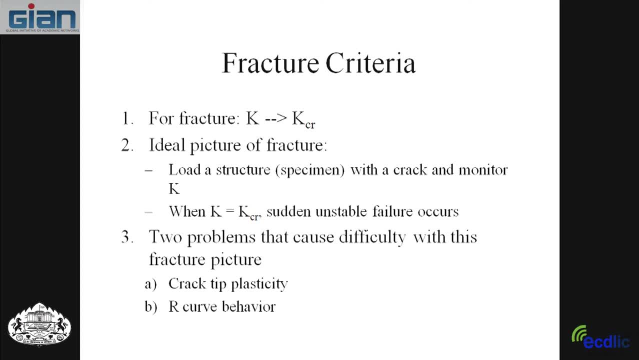 would just get the body to come into two pieces, like dropping a glass on the floor or something and bang, there's two or more pieces. And so ideally you want to load the specimen, keep a track of K. K gets to a certain point, then you get an unstable failure. We said 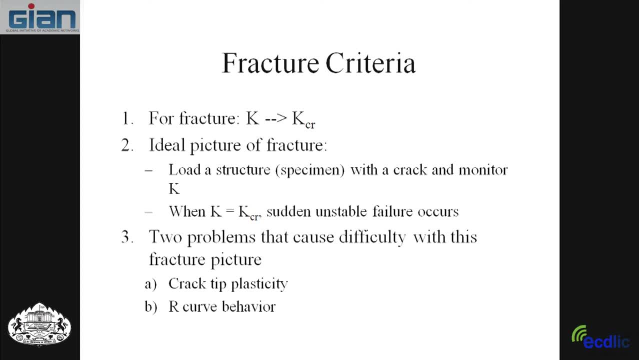 from the Griffith's point of view, that you would get that unstable failure because it's an unstable equilibrium. Anyway, two problems come and cause difficulty with this and they are the crack-tip plasticity and the R-curve behavior. And before you can do any testing you have to deal with those two difficulties First, 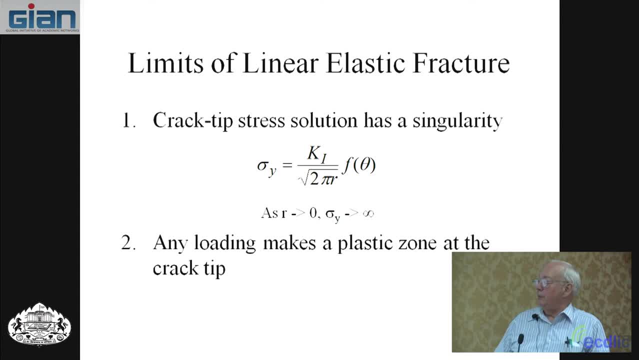 thing. look at the crack-tip stress and you see this: 1 over square. root of R and R, remember, is the distance from the crack-tip to the stress element. So as the stress element gets closer and closer to the crack-tip, you get what's called a singularity: 1 over square. 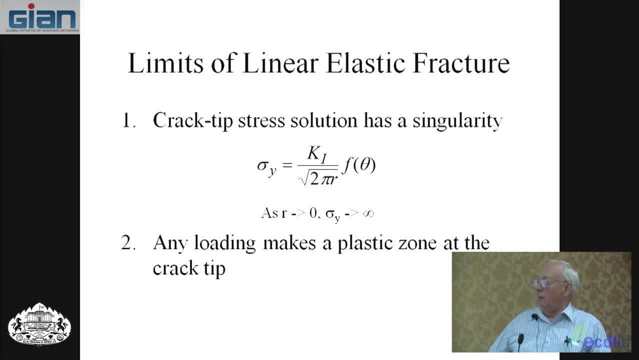 root of R singularity. So as R gets close to 0, the stress goes to infinity. Now you would think that infinite stress, then, should cause failure. but that's not necessarily so. It doesn't, because real materials, especially metals, can't abide very high stresses When 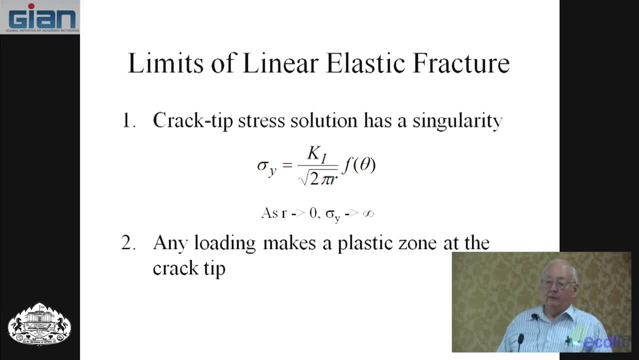 you get very high stresses. you get plasticity, So real materials get plasticity. So at the crack-tip, when you have this and you get close to the crack-tip, you get a plastic zone, And I'll show you this. So 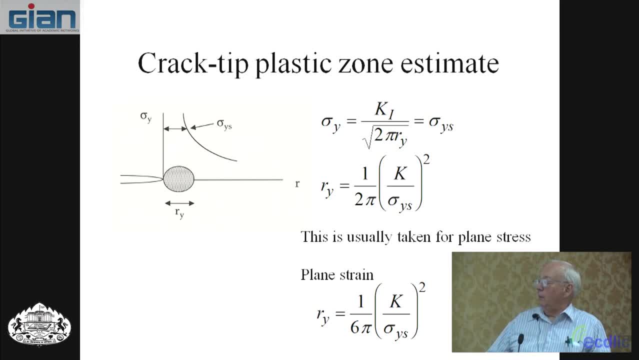 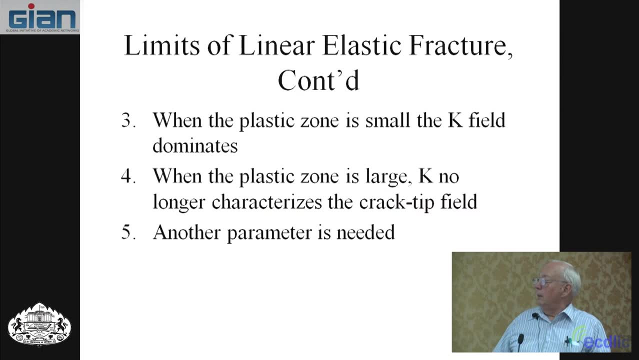 at the crack-tip. there this is the stress analysis: as you get close to the crack-tip and it gives you a plastic zone. If the plastic zone is small enough, it's contained by the K-field and the K-field dominates. But when the plastic zone gets too big, the K no longer. 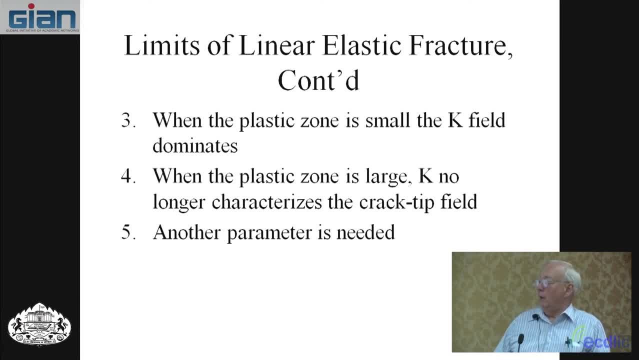 can dominate, And so it's not a good parameter anymore. So you can only use the K approach when the plasticity is sort of under control. When it's under control we call that behavior linear elastic fracture mechanics. So the whole stress analysis of Irwin is a linear. 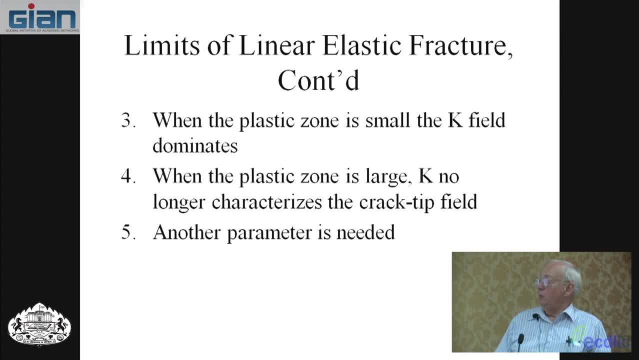 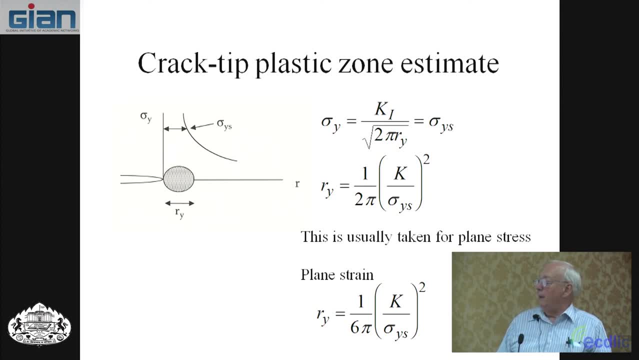 elastic stress analysis and to use it you need essentially linear elastic fracture analysis. Now, to calculate the size of the plastic zone, you can do this: Say that the Y stress K over square root of 2 pi r, and we're taking it where theta is 0. So when theta is 0, all. 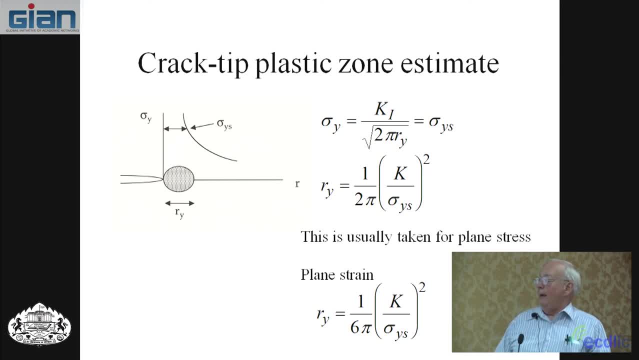 the theta functions go to 1, and then set that equal to the yield strength- Sigma sub Ys in our nomenclature stands for the yield stress- And then rearrange this and then you get the Ry is the size that a plastic zone has. 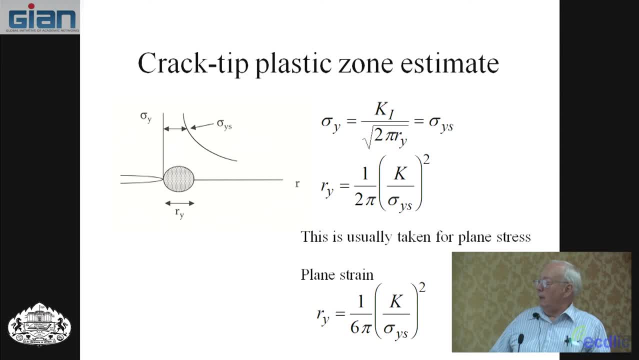 this character: 1 over square root of 2 pi K over the yield strength quantity squared. This size of plastic zone is the one we most often use. It's usually called the plane stress plastic zone If you have plane strain, which we'll talk more about later but means a more. 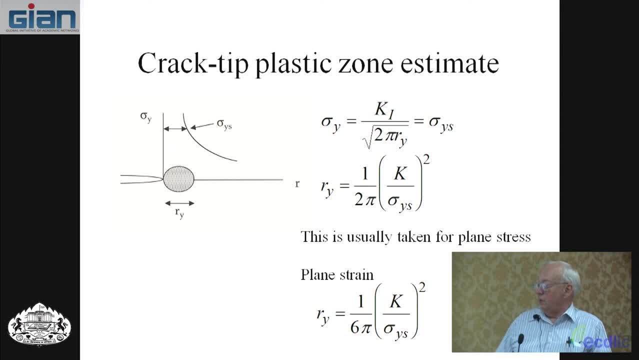 of a thickness constraint, a very thick structure. the plastic zone can be smaller and can have a 1 over 6 pi. So you go from 1 over 2 pi to 1 over 6 pi. And the reason we picked 1: 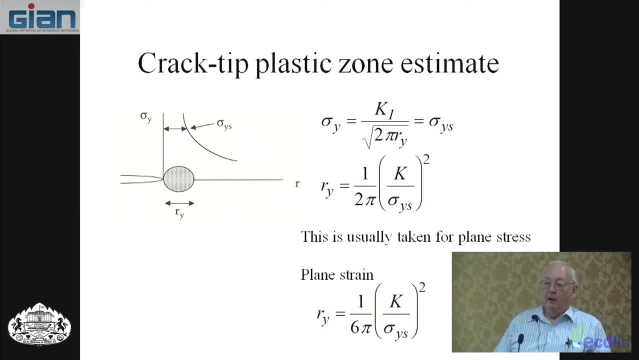 over 6 pi is because one time George Irwin said I think you ought to use 1 over 6 pi for plane strain And everybody said yeah, we ought to use 1 over 6 pi. So ever after that we've used 1 over 6 pi. However, when in doubt, use 1 over 2 pi. 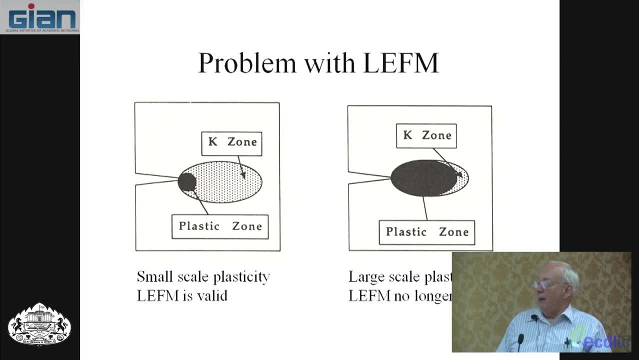 So here, schematically, is what happens. You get a little plastic zone, The K zone, which is the zone of where all the action is taking place. the black box dominates that plasticity and the plastic zone doesn't cause any problem. However, if the plastic 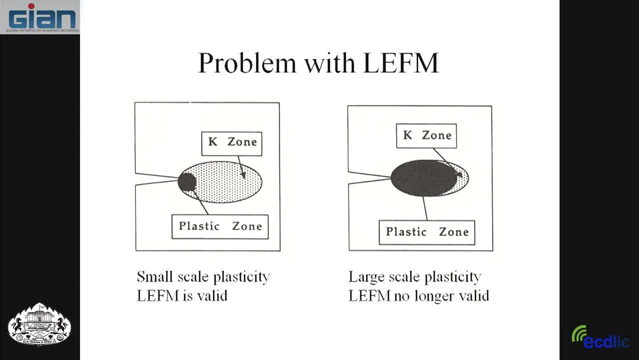 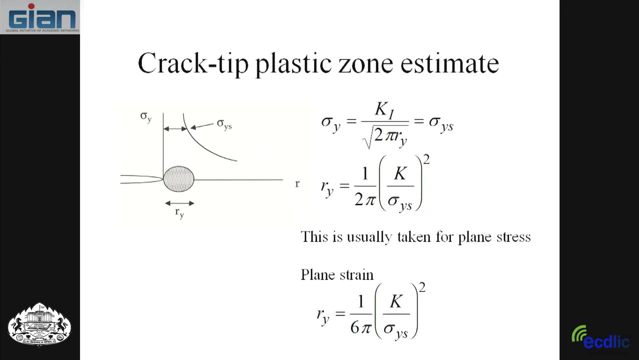 zone gets too big, then it wipes out the K zone And with the small plastic zone we have what we call linear elastic fracture matrix. It's valid here. Big plastic zone- it's no longer valid. Now, how big is too big All? 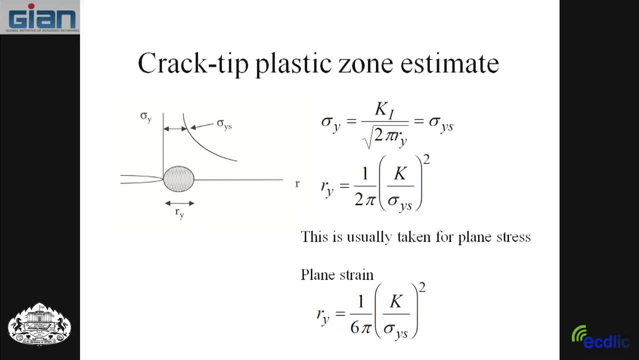 of the test methods have this built in automatically. So that automatically gets built in And you don't say up front how big is too big. But each test method, depending on what it is, has a different number for that or may have a different number, So it can vary from one. 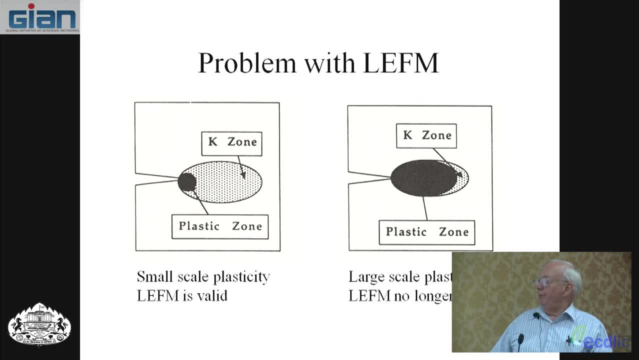 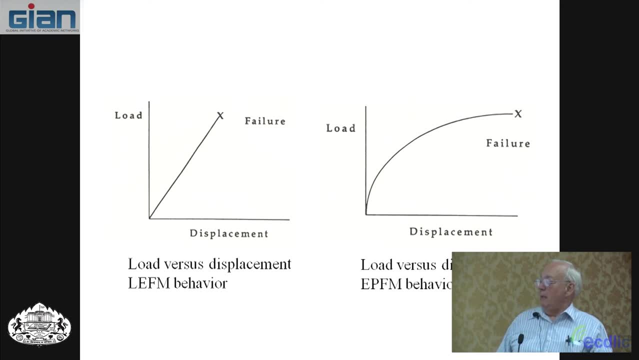 test method to another. So here's another way to tell that you have too much plasticity. If you have load and you measure displacement somewhere on the specimen and you get essentially a straight line, then you know it's essentially linear elastic behavior. So you know you're in this. 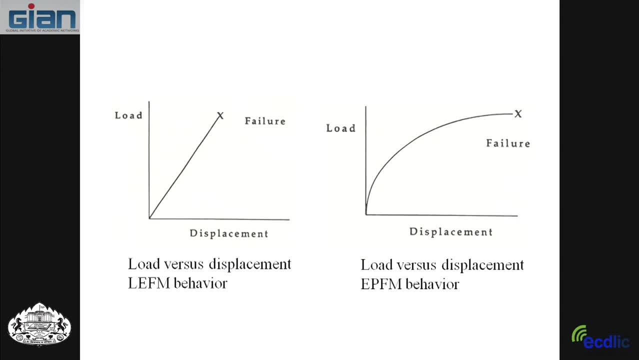 condition: small plastic zone. If you're loading and you get grossly non-linear load and displacement, then you have lost the linear elastic behavior And we often call that elastic plastic fracture behavior. So another way to tell- besides the plastic zone- is load and displacement. 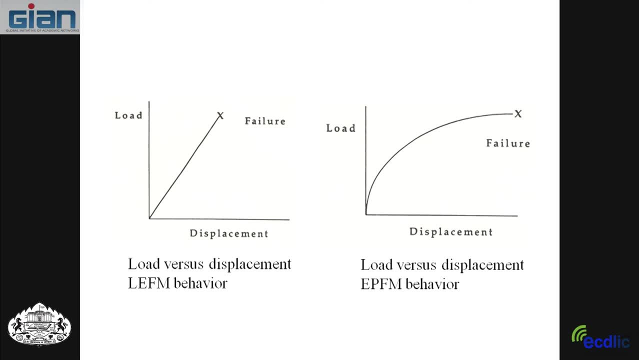 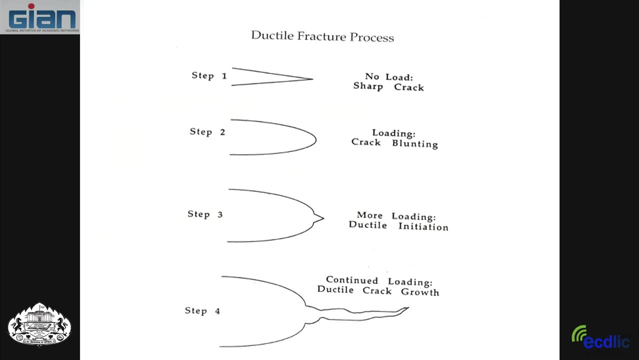 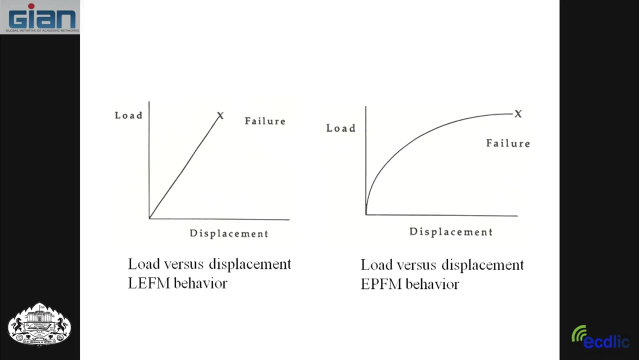 Almost all the tests have load and displacement measurement built into the test method So you can see if you essentially have this or essentially have that. Now the second problem, that's the plastic zone problem. So you always have to keep track of the plastic zone size and the amount of plasticity to tell. 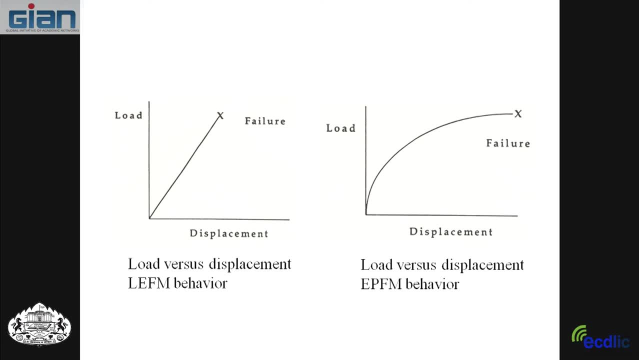 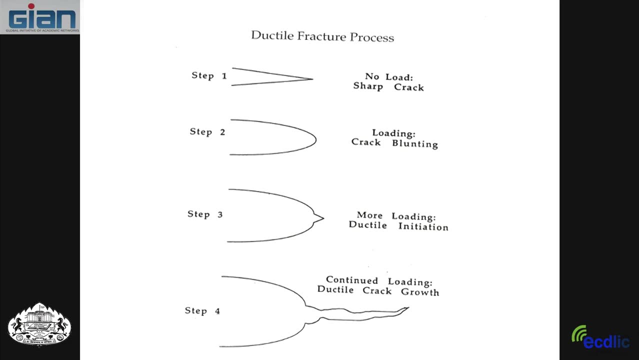 you whether or not you can use the K approach in your fracture mechanics. The other problem is called the R-curve problem or the ductile fracture problem. What you were kind of hoping is that when you pulled the specimen and got to the failure point, 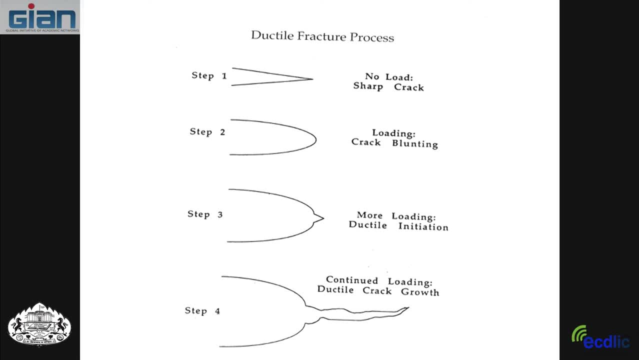 it would fail, Bang, It would come into two parts. But many materials, many metals are ductile and have a fracture process that doesn't involve breaking suddenly into two pieces. It kind of goes like this: You start with a sharp crack when you have no load. As you begin loading, that sharp crack can blunt As you. 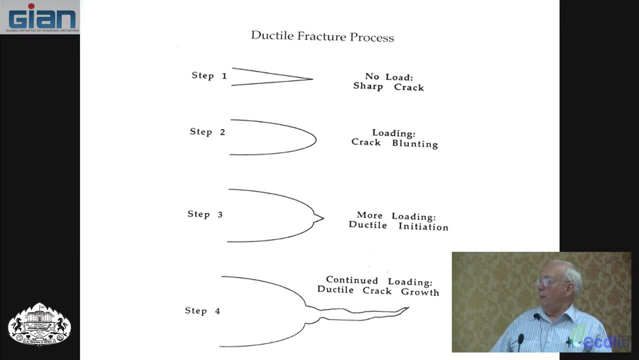 load some more. ahead of the blunted crack you develop another sharp crack which can grow in a stable manner. So this whole process can be stable. And what then is the difficulty is, where do you say fracture occurs? Of course it doesn't occur there. And maybe it's occurred. 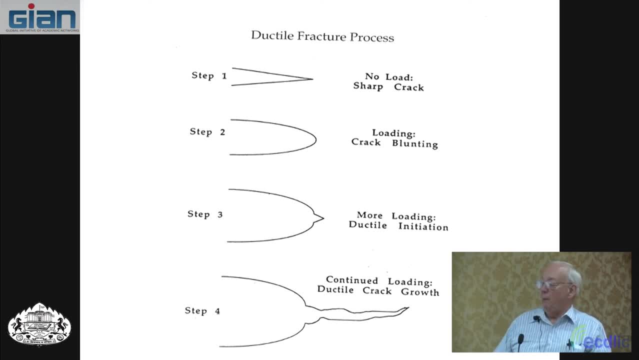 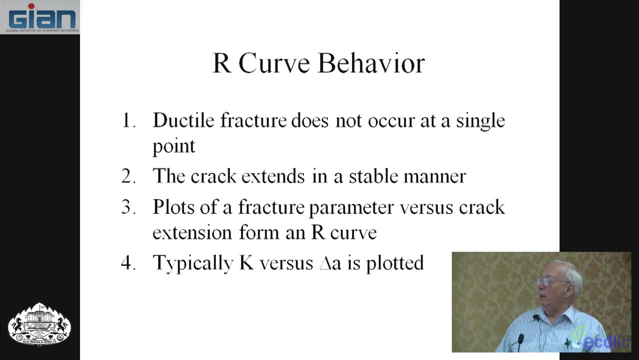 already here, But you have to be able then to pick a point that you say. this point is the fracture point And that again is built into the test methods. So R-curve behavior fracture does not occur at a single point, but rather crack extends in a stable manner. 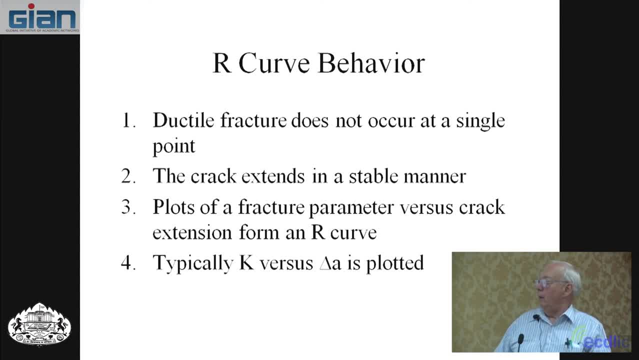 So people mostly plot then a fracture parameter versus crack extension and form an R-curve. Typically for a linear elastic fracture you would use K as a fracture parameter. Delta A is the change in crack length. It is plotted as the crack advance. So here's an example. 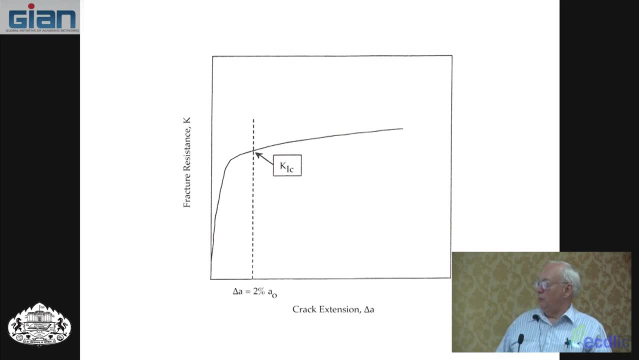 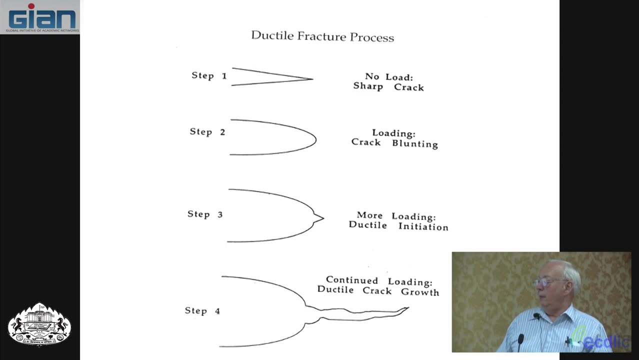 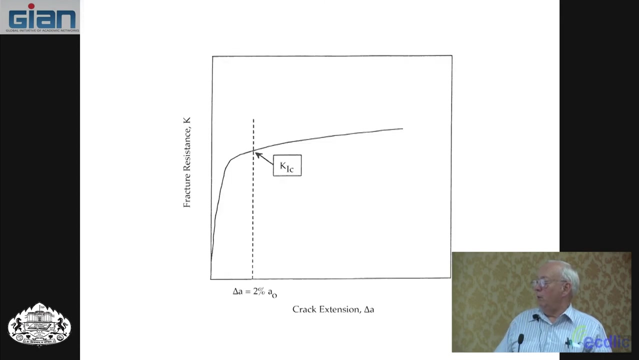 R-curve. You can ignore this for the time being, but it looks like this: This is crack extension. Delta A would be the current crack length versus the initial crack length. This is essentially this, And that's the R-curve plot, And so you have to be able to pick a point And in 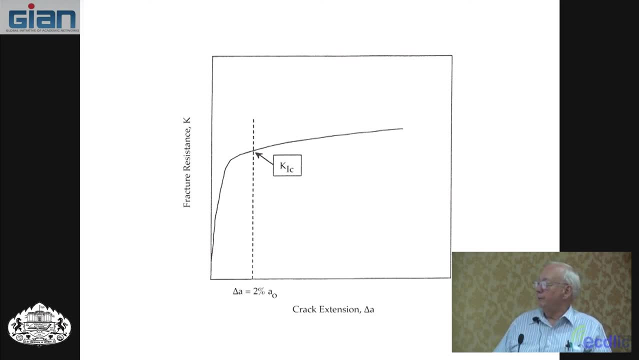 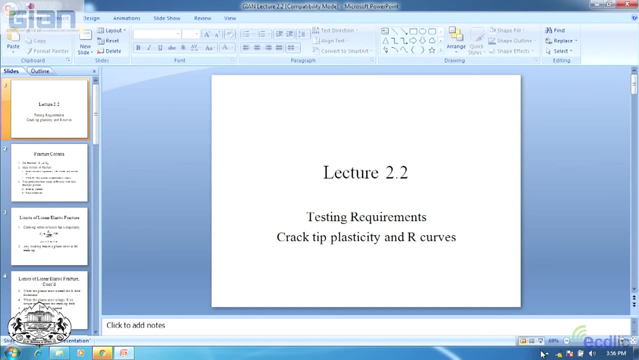 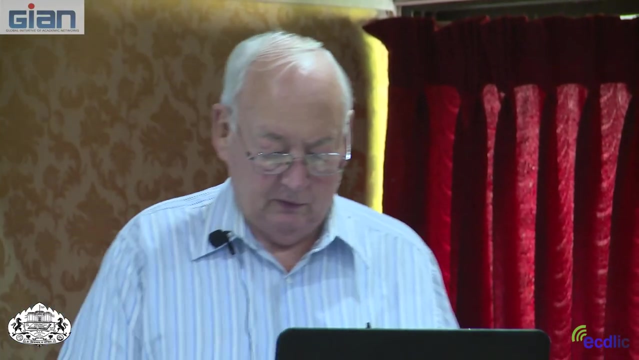 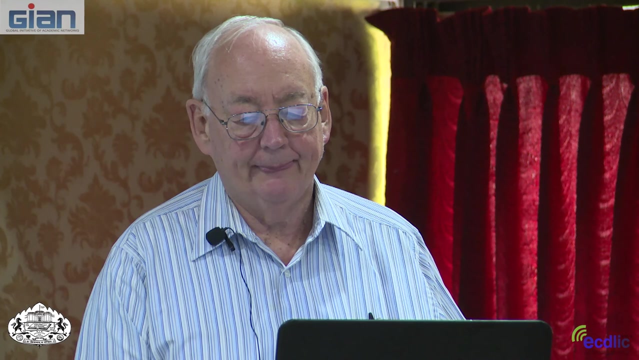 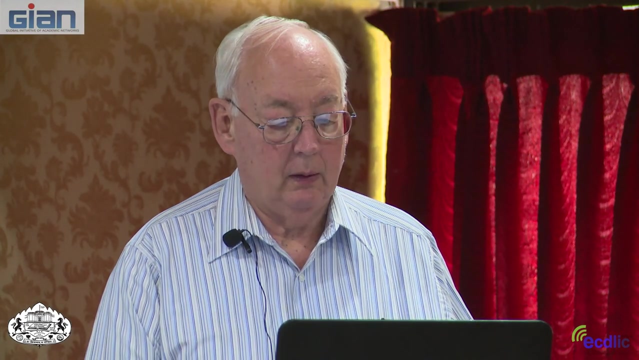 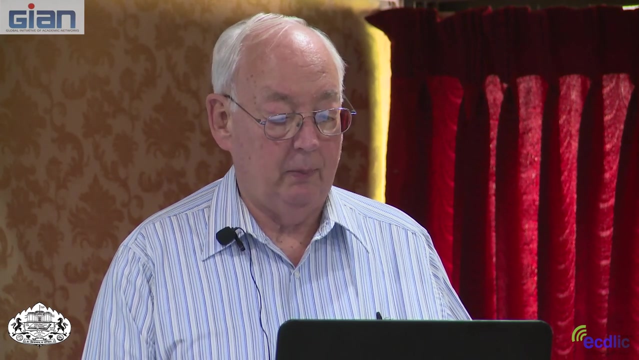 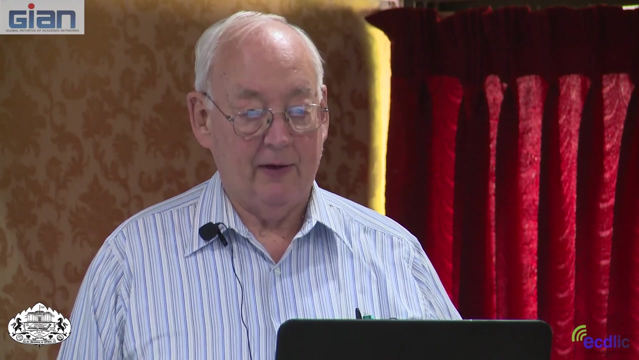 the K1C test. the point you pick is here, So let me show you this next thing. This is the most exciting part for you. I want you to do a little problem to determine whether or not this is a crack extension. Now, you still have a half hour, so you have time to work on this And I guess I'll go. 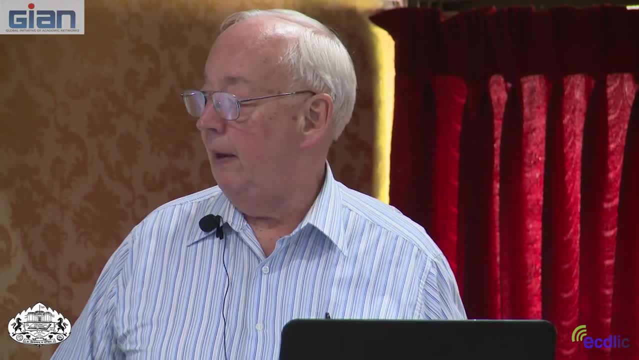 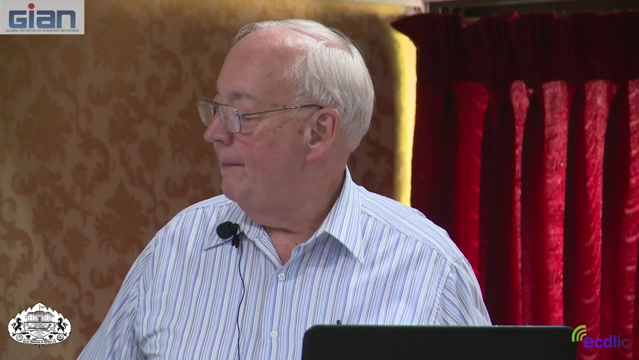 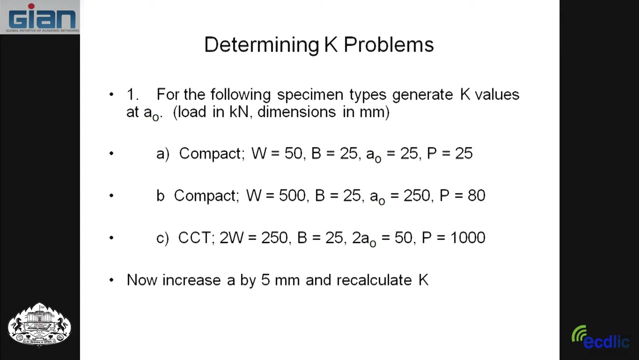 over the solution next time. But you should work then in determining the K Which. three examples here For the compact specimen: these are the W's And these are the K's. These are the W's, These are all in kilonewtons and millimeters, so SI units, here Two sizes. 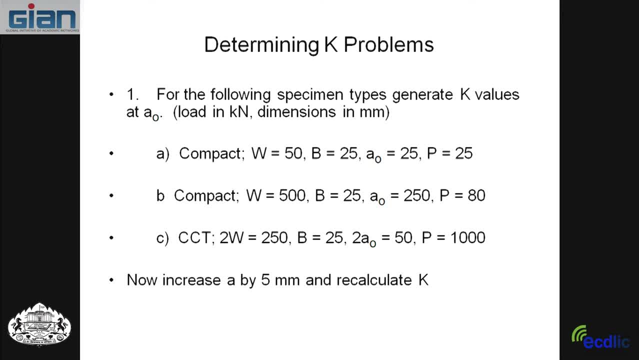 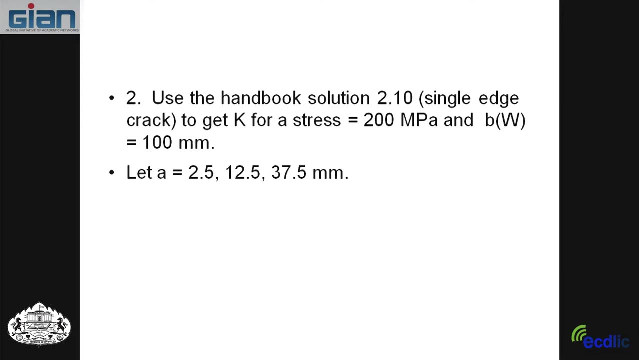 of compact specimen and one center crack. So for these initial conditions, calculate the K. Then you should increase the crack length by five millimeters and then recalculate the K. Here's another one. Use a single edge crack solution with a stress of 200 and B or W. 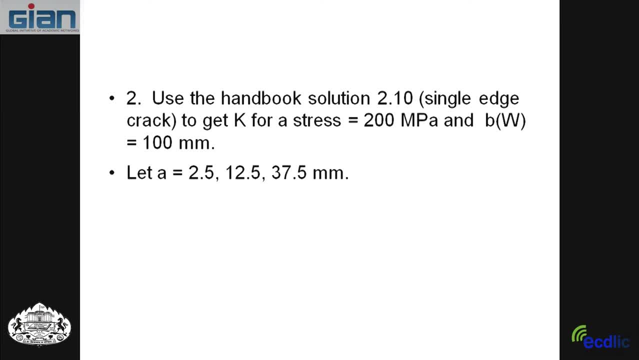 whatever you want to call it- 100 millimeters And crack lengths of these and get K. If you can do those, I'll give you a half hour to work on them. You'll have to learn to calculate your K so that you can go on and do other things because we'll be calculating. 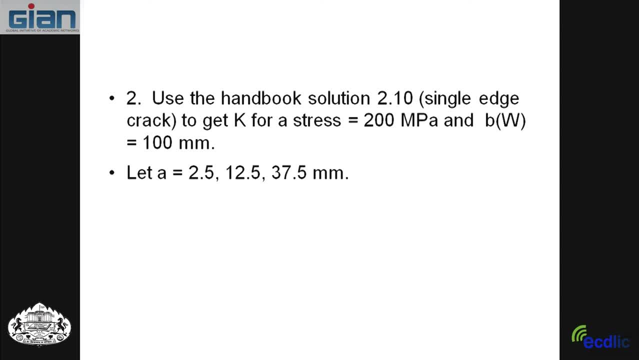 K's frequently. So everybody has a piece of paper. You have the K solutions. You can calculate a K if you want. My wife, I have a calculator here if you don't have one, but it's good to bring one. Does everybody have a calculator? 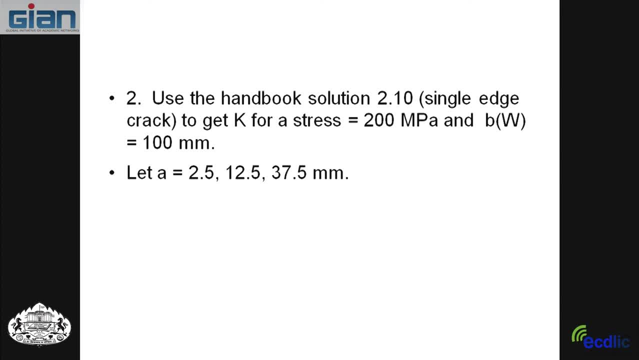 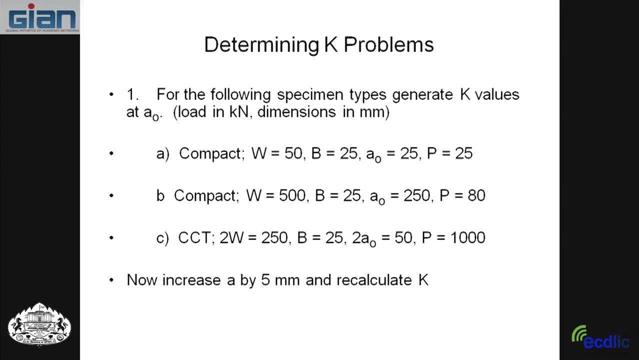 We don't have yours, It'll be much better. Let me keep this up for quite a while so you can see it, And you have the handout table. That's an important thing. You have to do a lot of math. You have to do some math as well. 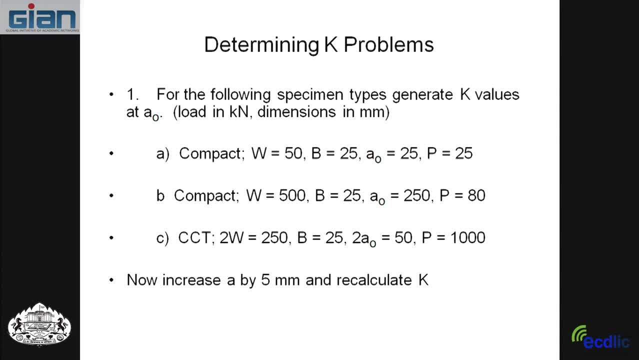 It's a lot of math. You have to do a lot of math, but you'll have to keep the K. You have to keep the K. Here's some more math And you're done. Here's the F, Thank you. 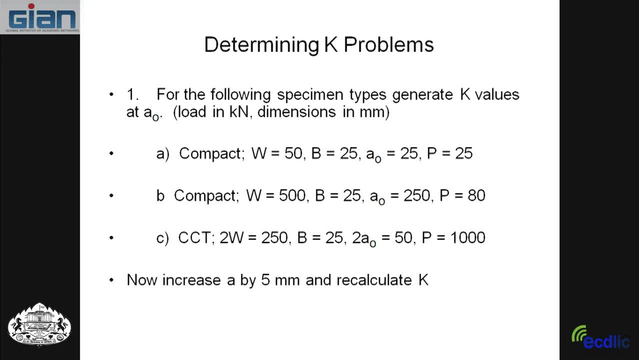 Thank you Again. if you're lacking a calculator, here's one. It's my favorite because it's the only one I have. Thank you, You can all work together. If you like the person sitting next to you, you can work together with them. 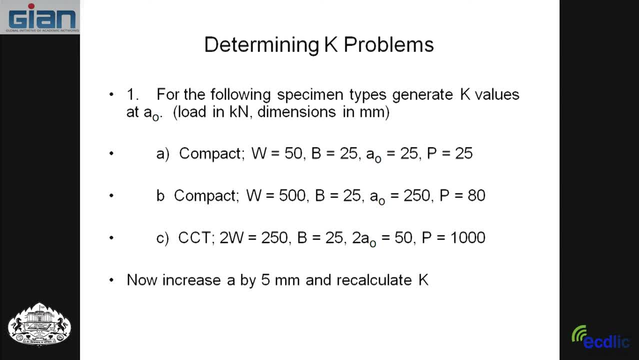 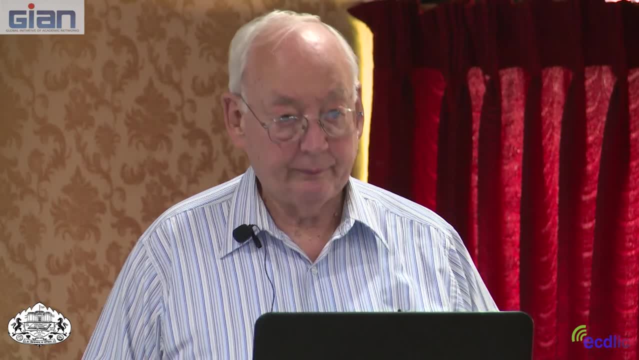 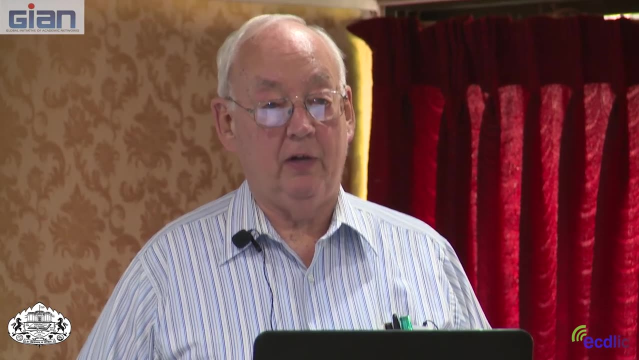 If you don't like them at all, you don't have to work with them. You may Thank you While you're finishing up. in the time remaining I'd like to go over the solutions for this, But as you're finishing up, let me tell you this problem. 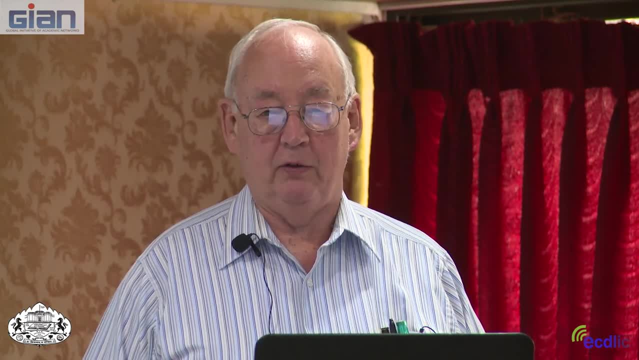 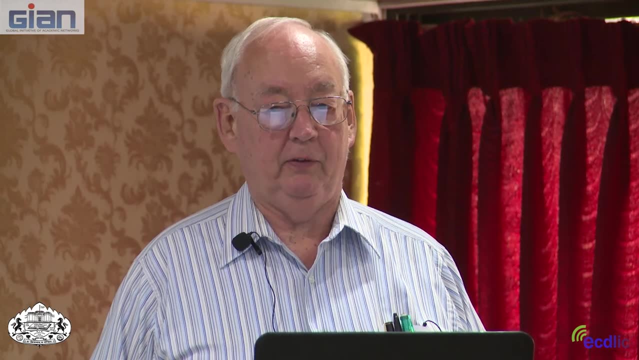 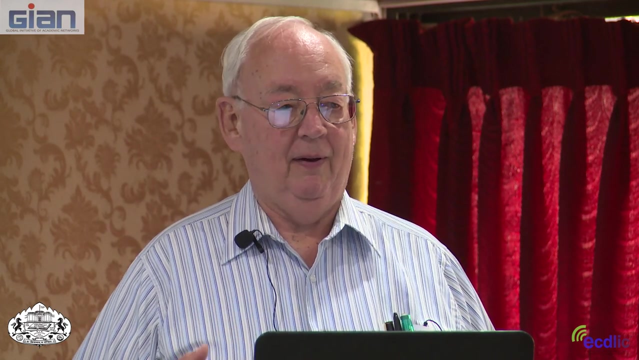 As you probably know, tomorrow we're having an important presidential election in our country And we thought, if things turn out badly, we might try to take a permanent residency in CUNA. We're staying in the Marriott, We have beautiful rooms, friendly people, great food and all the friends here. 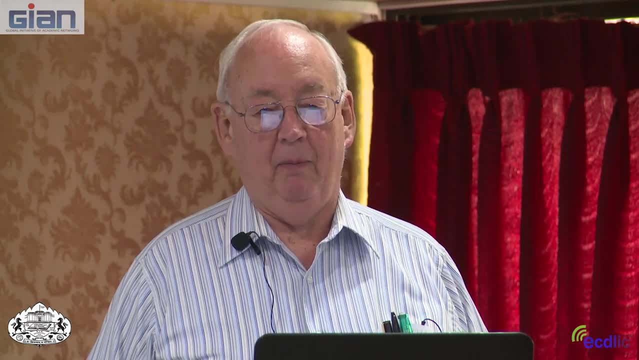 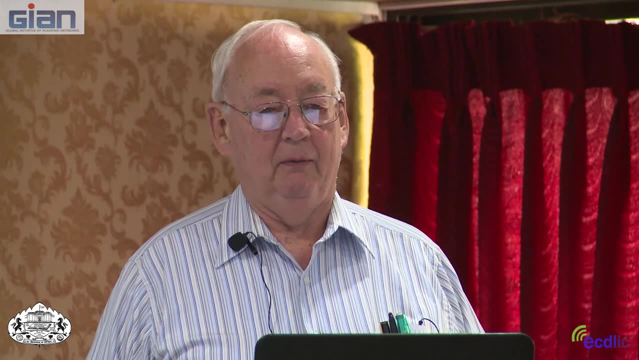 Mahir and everyone, Everybody. So the one problem we have, though, is my wife and I, and Becky also. we have three cats at home, And while we're home the cats don't say very much, But I know when we go away they get together and discuss the problem. 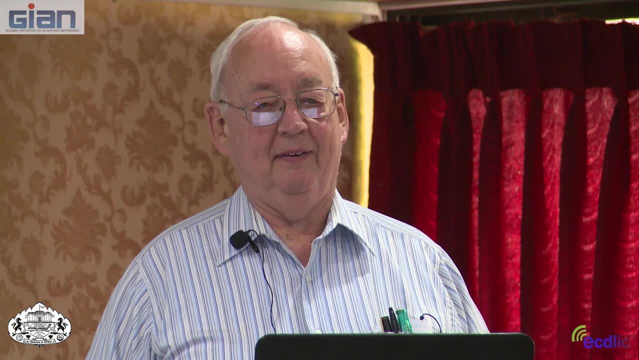 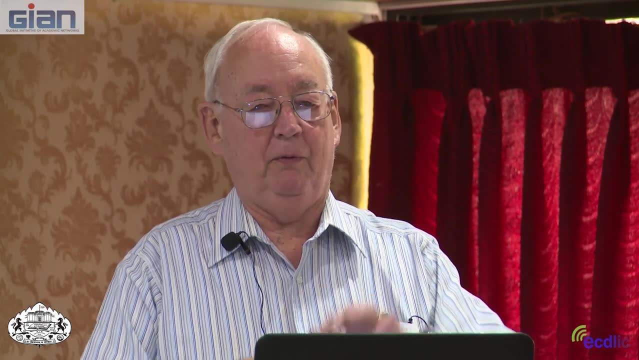 Do you think our parents are coming home today And to solve the problem? I tried to teach them to count, So I took their paws and their fingers and say one, two, three, four. They have four toes on each paw. 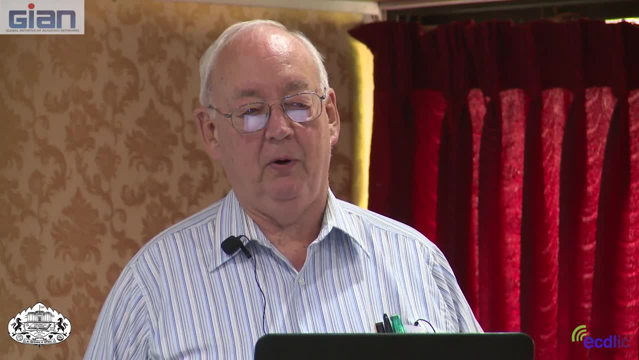 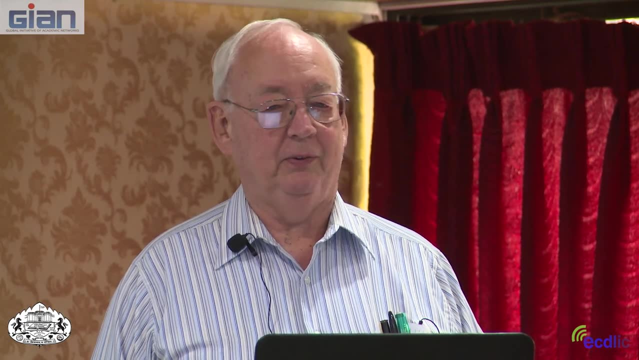 And the problem they have is it's only 16 paws and we're going 21 days Now. I don't know if you ever tried to teach a cat to count, But when they run out of toes they really get confused. 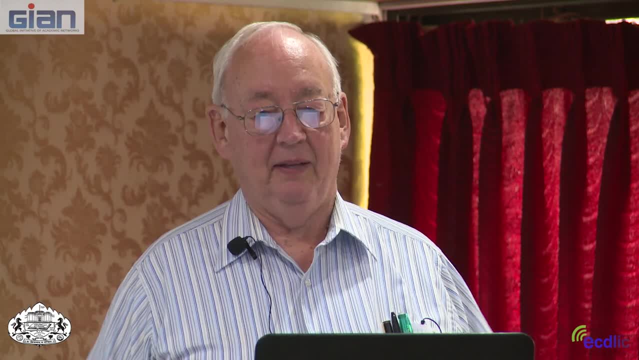 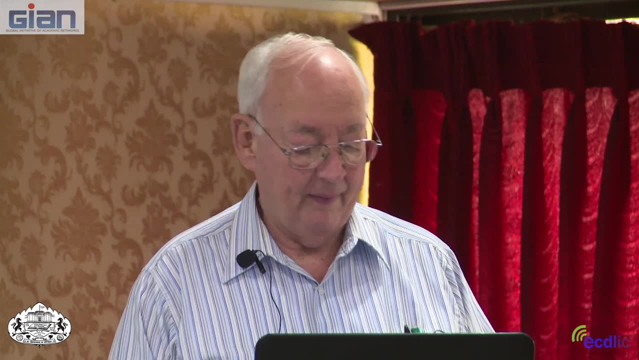 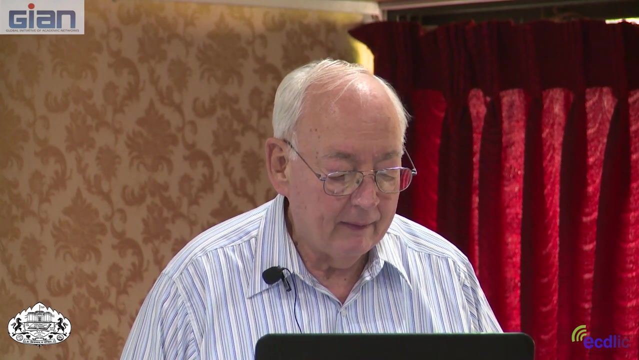 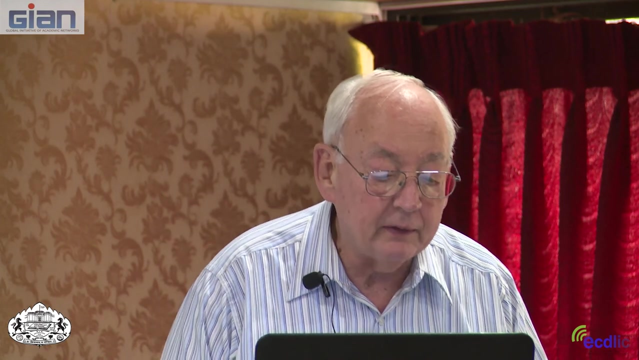 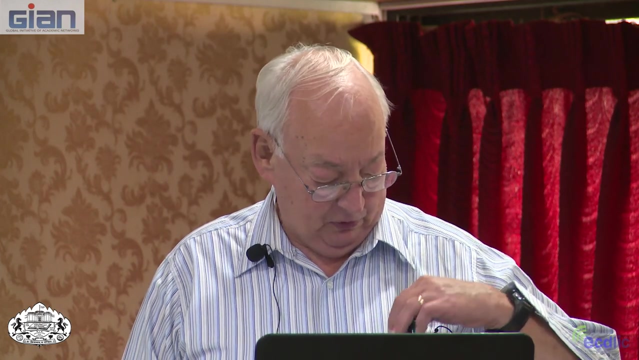 They can't do any more. So that's our problem. Might get us back. Yeah, I don't want to jump too much. Anyway, I don't know what that little field is. You can go away. Here are some solutions. 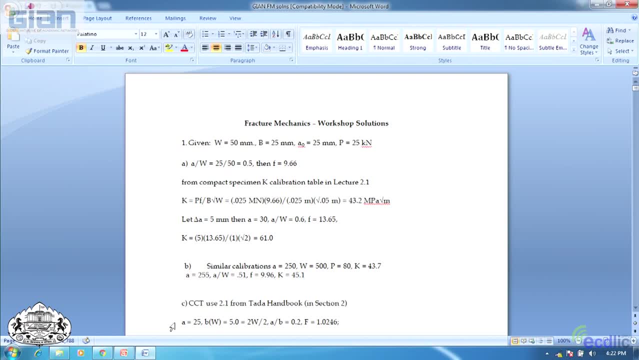 If you're not finished, you can just follow along, And this will take us to the end of our time. Anyway, for the first problem, W is 50, B is 25, A is 25, load is 25 kilonewtons. 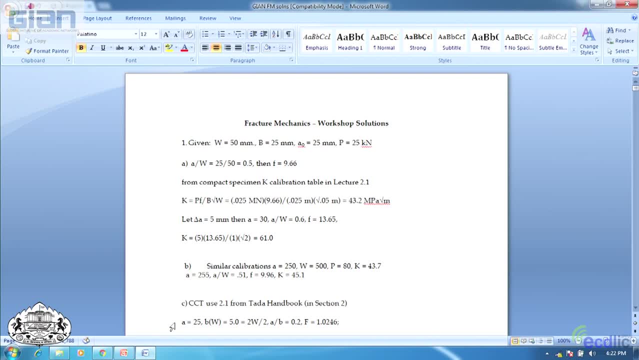 You got to make sure You keep the units straight. That's a little problem, But you always start out calculating Ks with A over W. So the crack length to the specimen width ratio is always important Because that tells you where to get on the table. 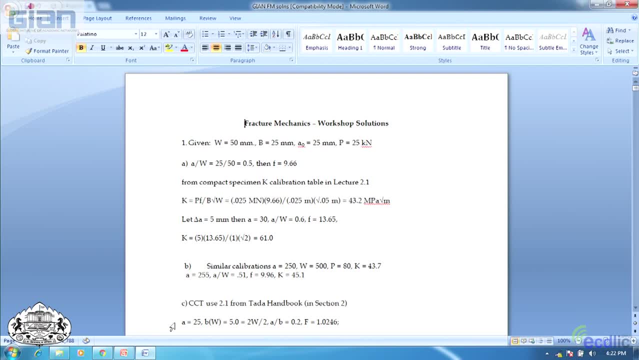 Here it's simply 0.5. Then if you go to the table, the table value says F is 9.66 rounded off And put that all together Now load is 25 kilonewtons. And remember the unit's MPA root meters. 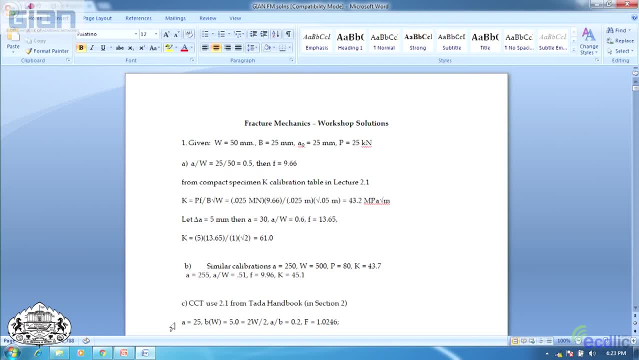 So in order to do that, I put everything in mega newtons and meters. If you're real good with units, you can get away without doing that, But I have trouble, So I put everything in mega newtons. That's the little F is unitless. 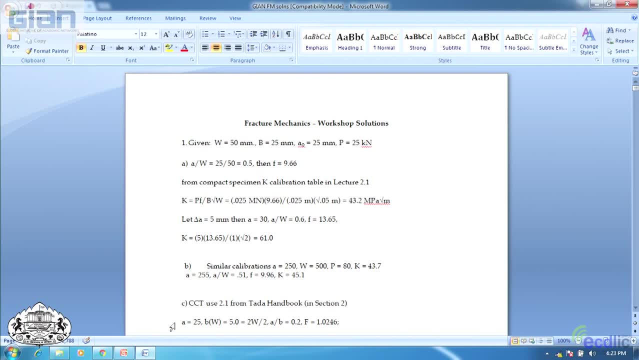 Then the thickness is .025 meters And this is square root. root of 0.05 meters. I got 43.2.. Now, if you didn't get that to start out, you ought to try it again, because that's what you should get. Anyway, if you change the crack length, 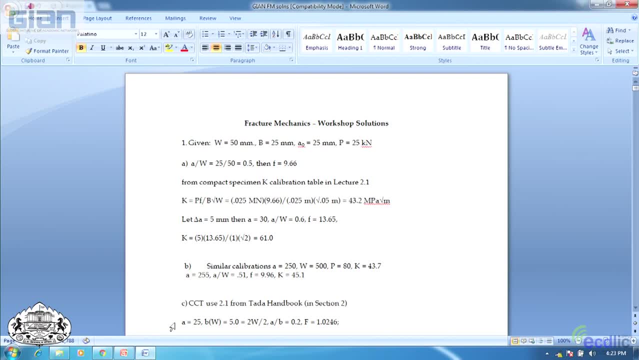 by 5 millimeters, then the crack size is now 30, A over W is 0.6, and F goes up. Everything else stays the same in the K calculation, but the F goes up. So recalculating that. 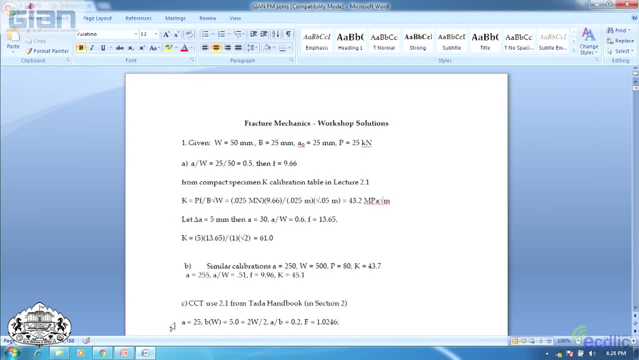 the K went up to 61. So you can see just increasing 5 millimeters went from 43 to 61, and it's very dependent on crack size. Now I don't have all the details, but part B is W is 500, and A is 250, so it's just a 10 times planar size specimen and same thickness. 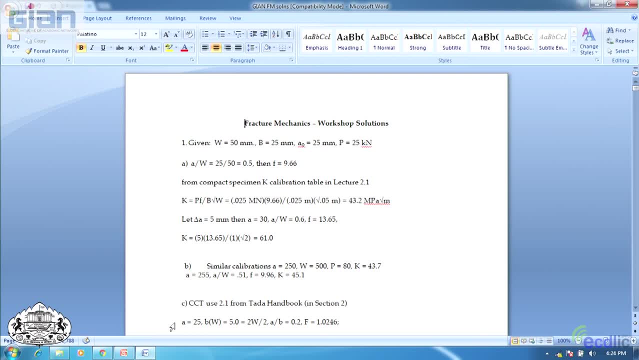 and then I got. I got K of 43.7, about the same Now when I increased crack size 5 millimeters, so 255 millimeters. A over W just goes up to 0.51, and F just goes up a very small amount. so 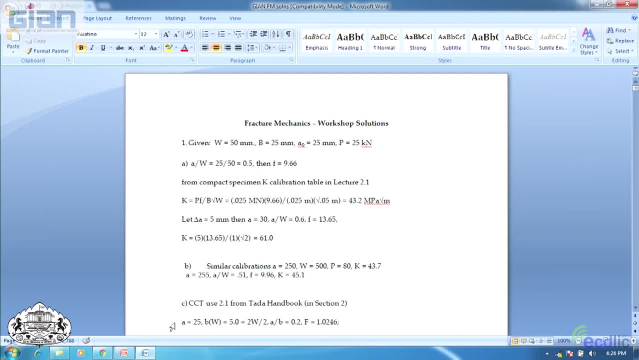 K went up to 45.1.. One point I wanted to make in calculating this is that K increases with crack size. It increases much more quickly when you have a really small structure or specimen. It increases much more quickly for a given increment of. 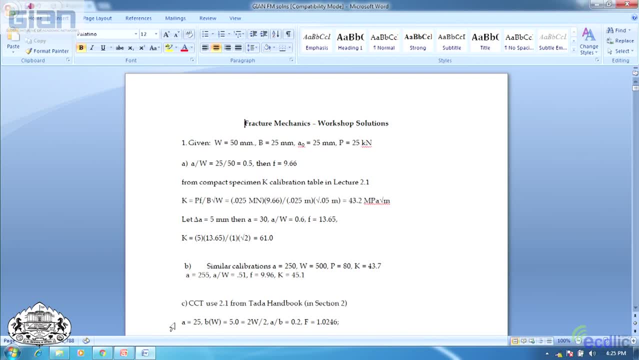 crack growth than it does on a real big specimen. So this one K went up almost 50%. Here it only went up a few percent. So that's, that's that Questions on that one. Okay, let me show you the other one, which. 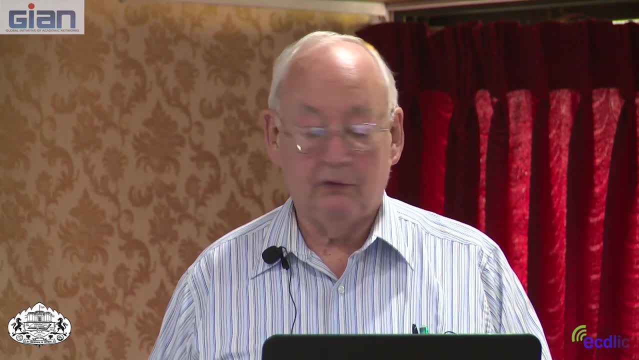 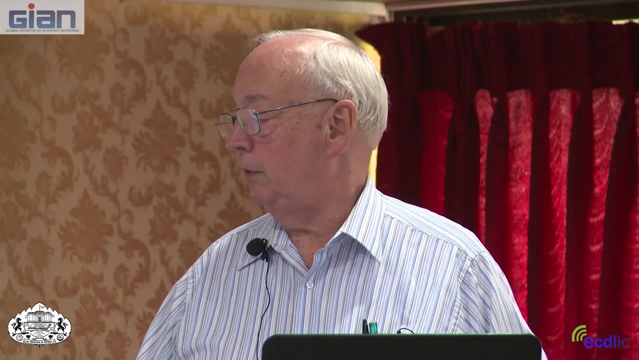 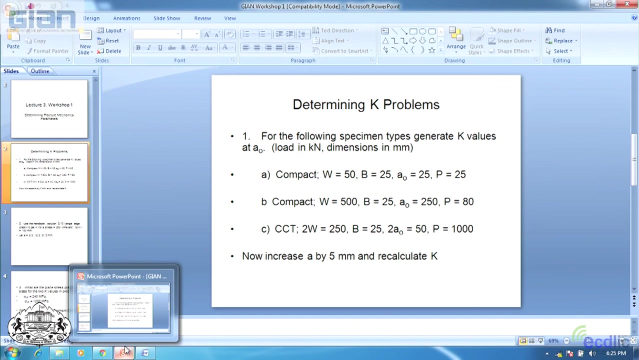 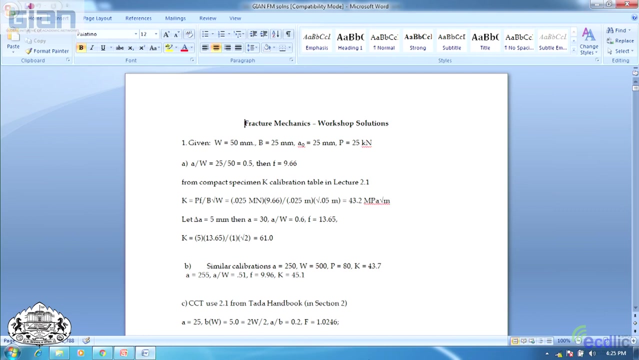 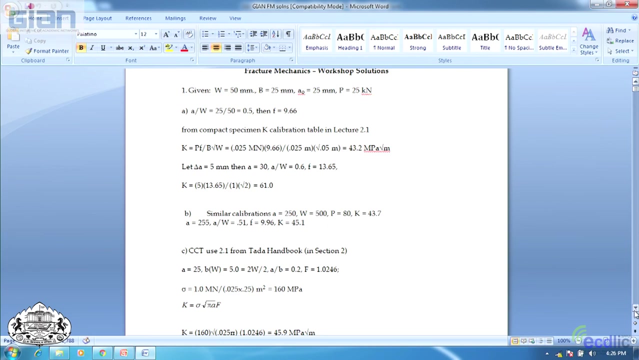 The center crack geometry, 2W or 2B is 250,, thickness is 25,, 2A is 50, and load is 100.. These are all millimeters and kilometers. This. you should definitely use that picture. So I have here A25, B or W is 0.5, which is 2W over 2.. 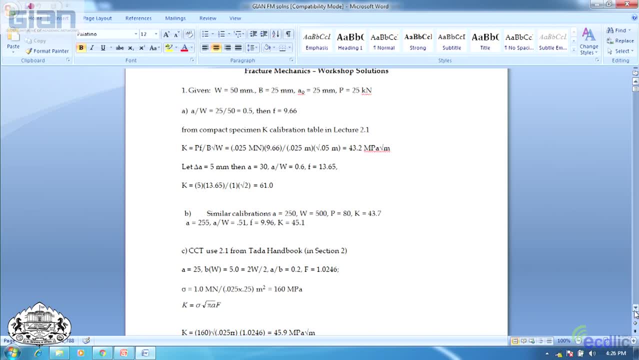 A over B is 0.2.. Then, if you read from the table and don't use the graph, F is 1.0246.. So now stress, I calculate it before the crack is there, As the load: 0.2.. 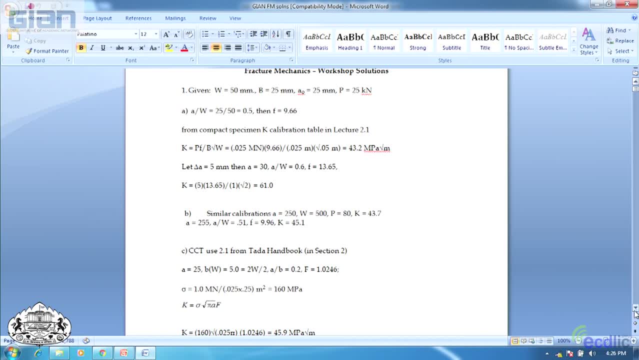 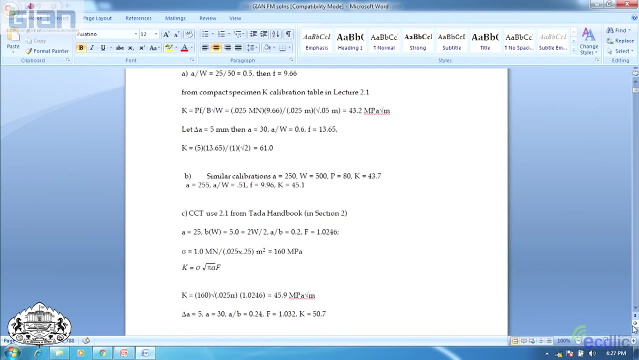 1 meganewton divided by 0.025 thickness and 0.25 meter square to get the stress of 160 using this k solution is then: k is sigma. Well, I'll do it here. My battery is gone here. k is sigma, 160 square to pi. a. This is all under the radical. I didn't have a software to do that. 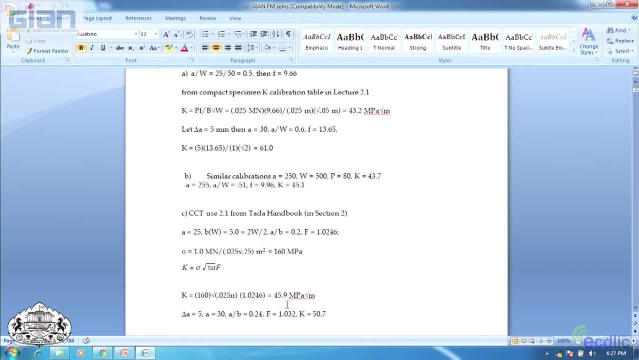 This is outside, But anyway 45.9.. Change the crack length by 0.5.. A over B is 0.24.. On that table, if you do linear interpolation that's good enough. You don't need to do anything real fancy. So linear interpolation pretty much gets it. And then capital F goes 1.032.. That was my linear interpolation.